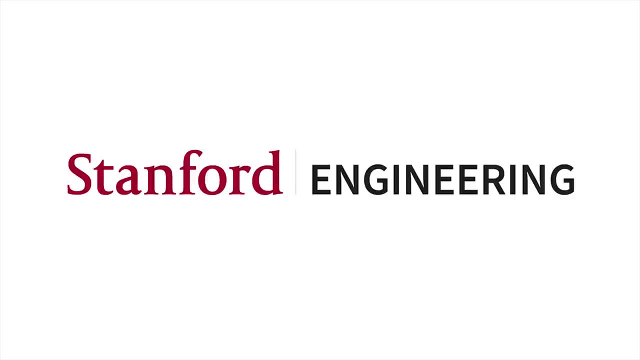 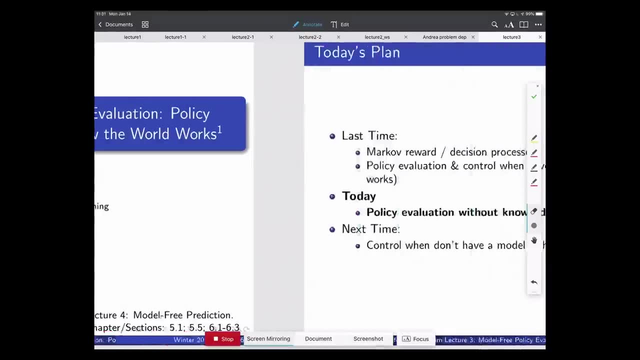 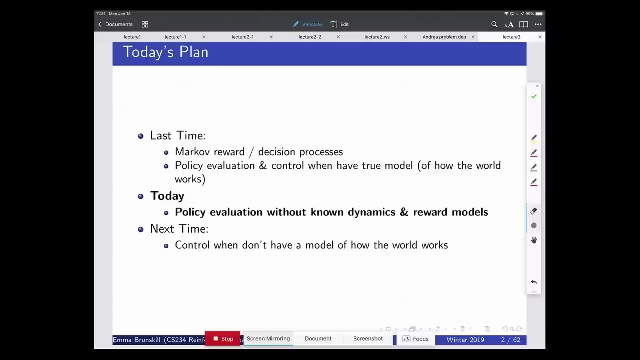 So what we're going to do today is we're going to start to talk about model-free policy evaluation. So what we were discussing last time is we started formally defining Markov processes, Markov reward processes and Markov decision processes, And we were looking at 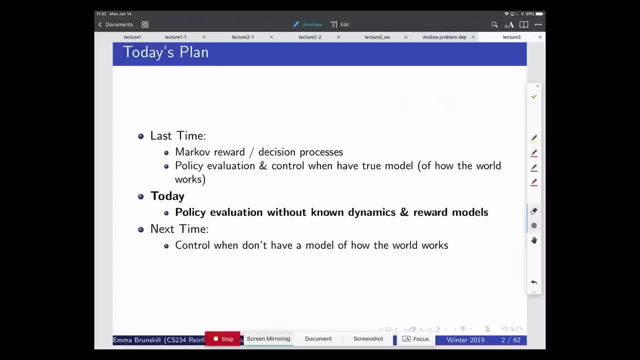 the relationship between these different forms of processes, which are ways for us to model sequential decision-making under uncertainty problems. So what we were thinking about last week was: well, what if someone gives us a model of how the world works, So we know what? 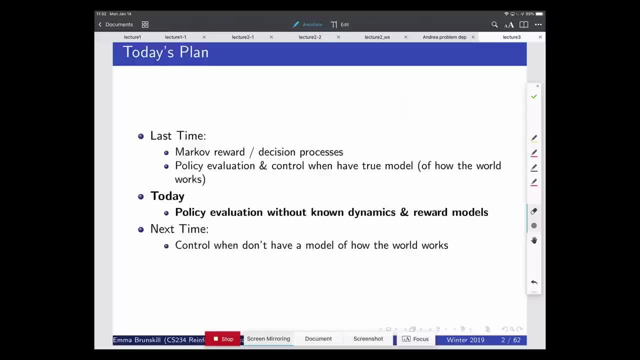 the reward model is. We know what the dynamics model is. It still might be hard to figure out what's the right thing to do. So how do we take actions or how do we find a policy that can maximize our expected discounted sum of rewards, Even if we're given a model? 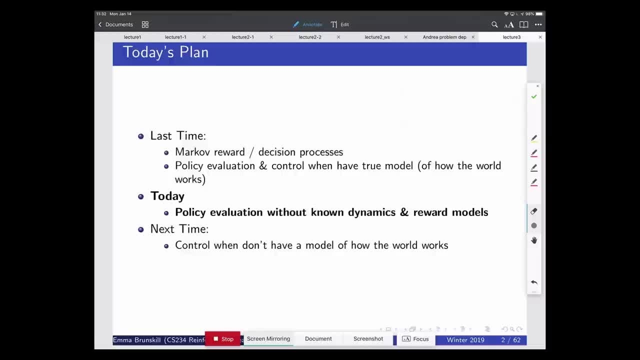 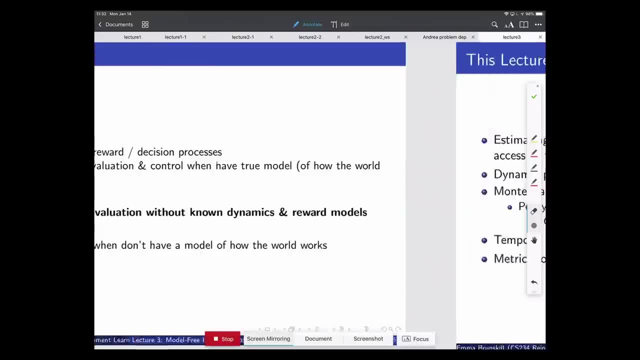 then we still need to do some computation to try to identify that policy. So what we're going to get to very shortly is: how do we do all of that when we don't get a model of the world in it? But let's just first recap this general problem of policy evaluation. So we heard a little. 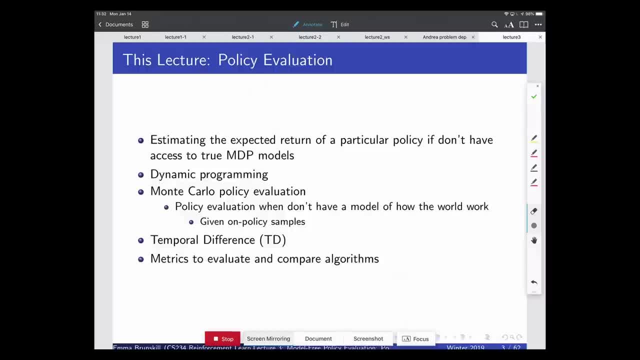 bit about policy evaluation last time when we talked about policy evaluation as being one step inside of policy iteration, which alternated between policy evaluation and policy improvement. So the idea in policy evaluation is that somebody gives you a way to act and then you want to figure out how good that policy is. So what is the expected discounted 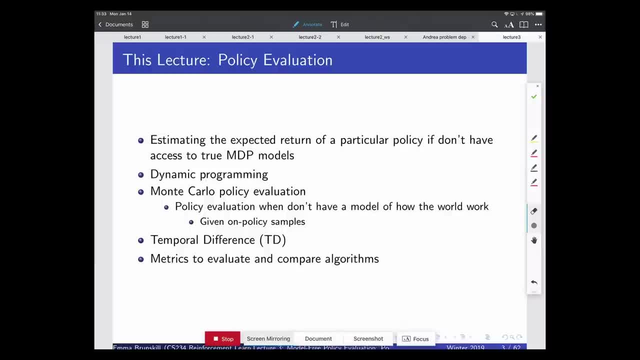 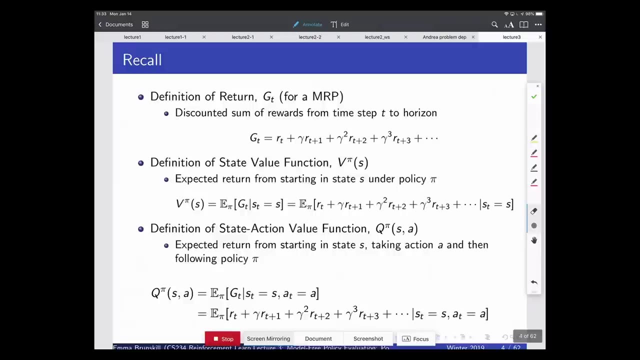 sum of rewards for that particular policy, And what we're going to be talking about today is dynamic programming, Monte Carlo, policy evaluation and TD learning, as well as some of the ways that we should think about trying to compare between these algorithms. So, just as a brief recall, remember that last time. 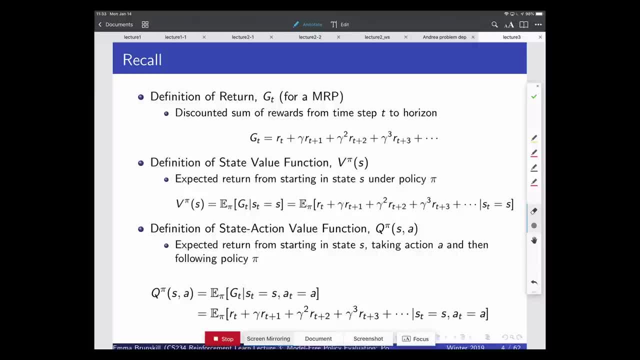 we defined what a return is for a Markov reward process, And a return for a Markov reward process that we defined by GT was the discounted sum of rewards we get from that particular time, point T Onwards. So we're going to get an immediate reward of our T And then after that we're 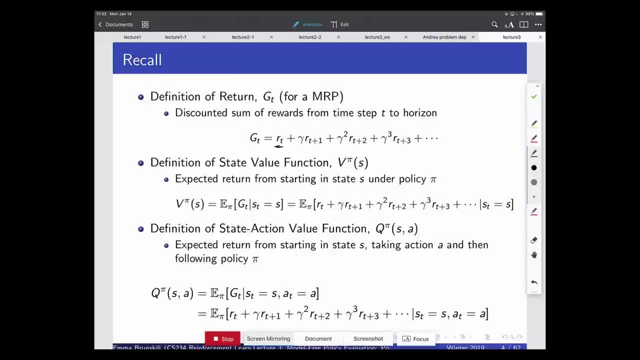 going to get gamma, where gamma was our discount factor And remember we're going to assume that's going to be somewhere between 0 and 1. And so we're sort of weighing future rewards generally less than the immediate rewards. The definition of a state value function was: 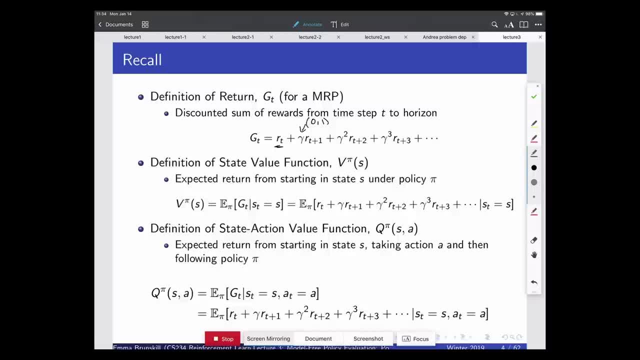 the expected return And, in general, the expected return is going to be different from a particular return if the domain is stochastic, Because the reward you might get when you try to drive to the airport today is likely going to be different than the reward you get when you. 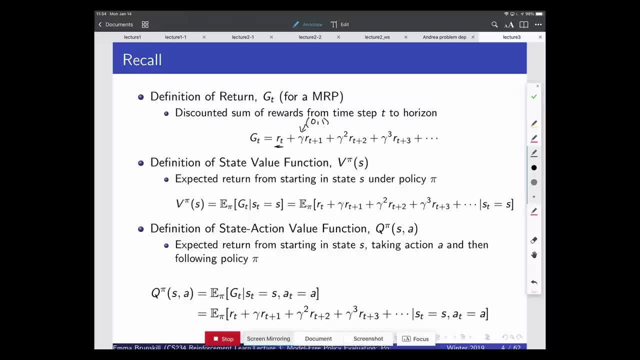 drive to the airport tomorrow, because traffic will be slightly different And it's stochastic. It varies over time And so you can compare whether in a particular day, if it took you two hours to get to the airport, versus on average, it might take you only an hour. 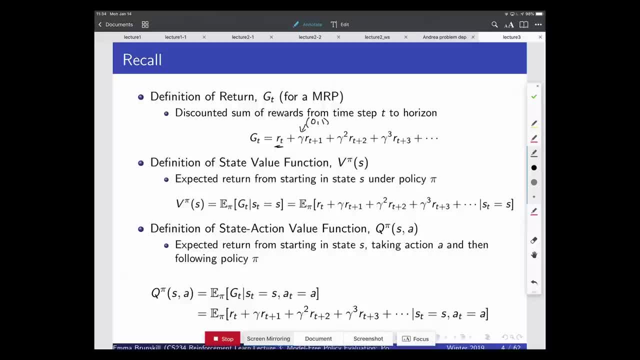 We also defined the state action value function, which was the expected reward if we're following a policy pi, But we start off by taking an action A. So we're saying, if you're in a state S, you take an action A And from then onwards you follow this policy pi that someone's given. 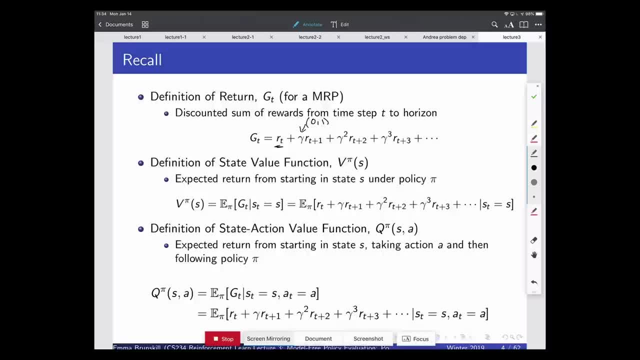 you, What is the expected discounted sum of rewards? And we saw that Q functions were useful because we could use them for things like policy improvement, because they allowed us to think about: well, if we want to follow a policy later, but we do something slightly. 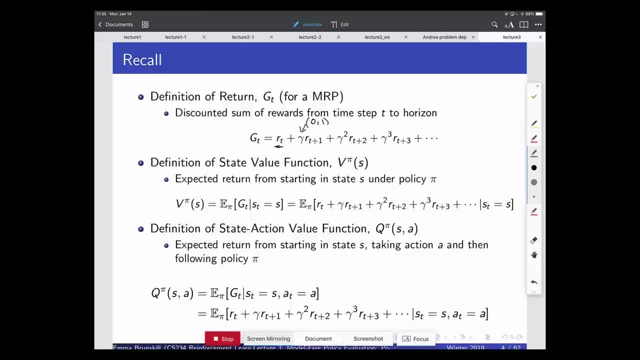 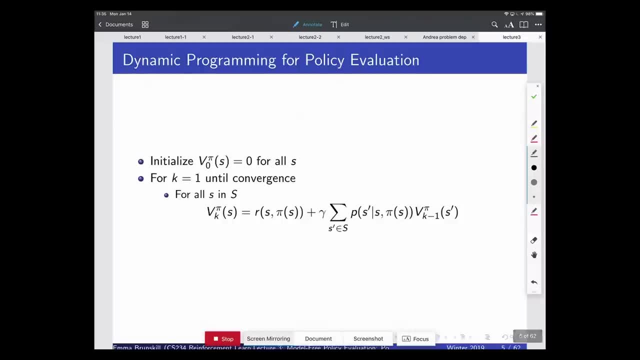 different to start? can we see how that would help us improve in terms of the amount of reward we'd obtain? So we talked about this somewhat but, as a recap, we talked about doing dynamic programming for policy evaluation. So dynamic programming was something we could apply when we know how. 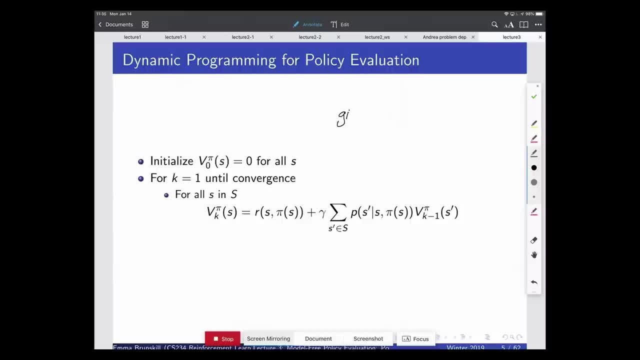 the world works. So this is when we're given the dynamics- And I'll use the word dynamics or transition model interchangeably in this course. So if you're given the dynamics or the transition model, P and the reward model, then you can do dynamic programming to evaluate how good a policy is, And so the way we talked- 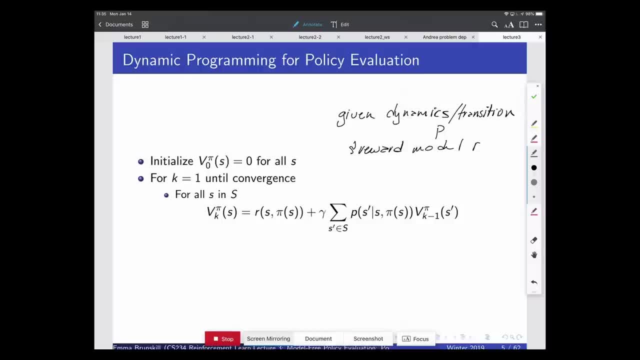 about doing this is that you initialize your value function, which you can think of generally as a vector- Right now, we are thinking about there being a finite set of states and actions- So you can initialize your value function for this particular policy to be zero And 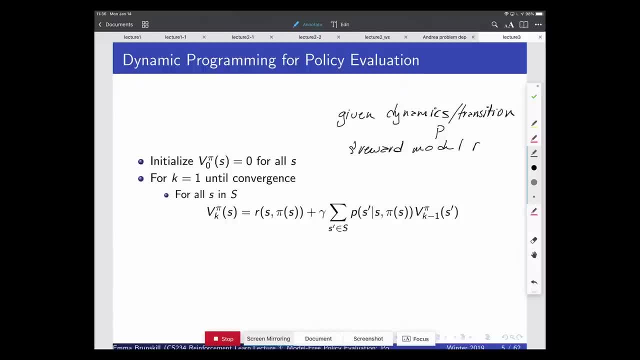 then you iterate until convergence, where we say the value of a state is exactly equal to the immediate reward we get from following that policy, And so you can do dynamic programming in that state, plus the discounted sum of future rewards we get using our transition model and the value that we've computed from a previous iteration. 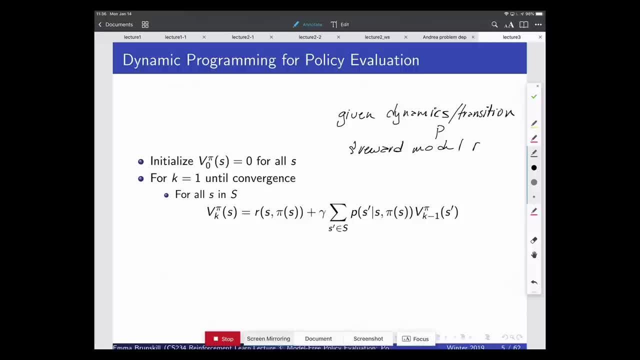 And we talked about defining convergence here, Convergence generally. we are going to use some sort of norm to compare the difference between our value functions on one iteration and next. So we do things like this: V pi at k minus V pi at k minus 1. And wait for. 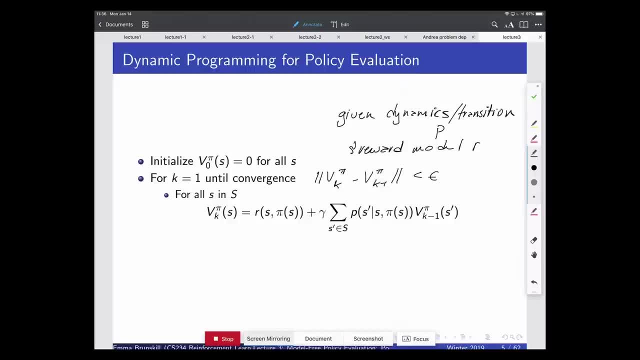 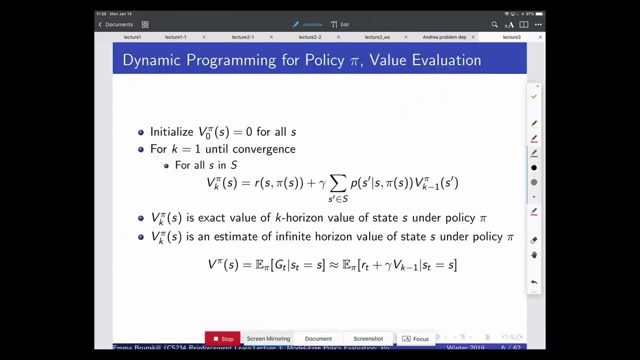 this to be smaller than some epsilon. So, just as a reminder too, what is this quantity that we're computing representing? Well, we can think of this quantity that we're computing as being an exact value of the k-horizon value of state s under that policy. So, on any particular iteration, it's as if we know exactly what. 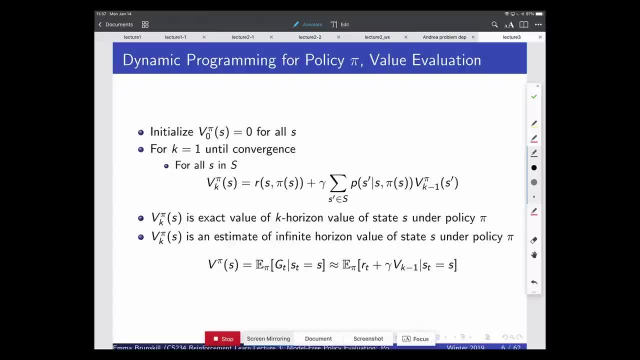 value we would get if we could only act for a finite number of time steps, like k time steps. It says: you know, how good would it be if you followed this particular policy for the next iteration, And so we can think of this quantity as being an exact value of. 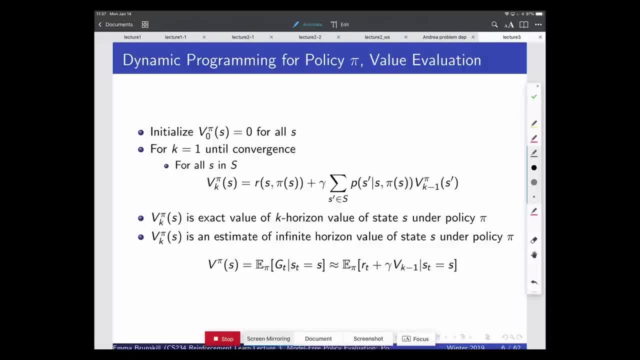 the next k time steps. Equivalently. you can think of it as an approximation of what the value would be if you acted forever. So if k is really large, k is 20 billion, then it's probably going to be a pretty good approximation to the value you'd get if you'd act forever. 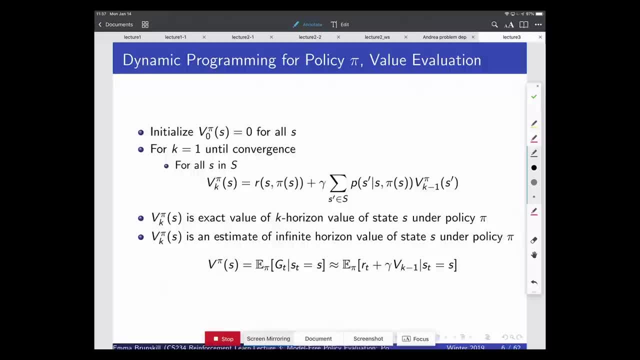 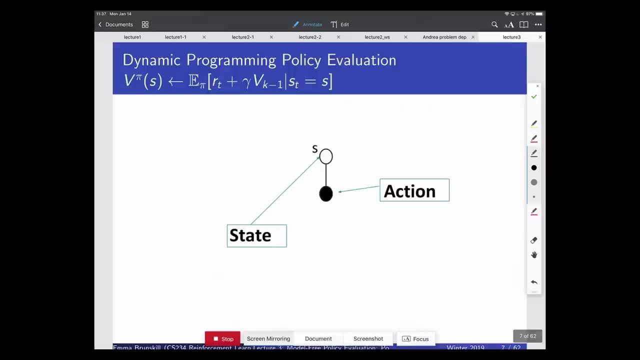 And if k is 1, it's probably going to be a pretty bad estimate. This will converge over time, So I think it's useful to think about some of these things graphically as well. So let's think about this as you're in a state s, which I'm denoting 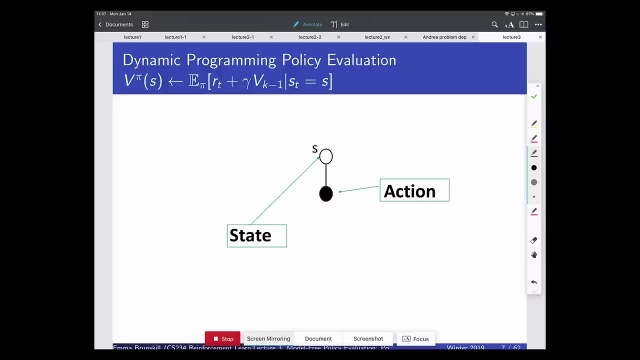 So I'm denoting with that white circle at the top, And then you can take an action. So what dynamic programming is doing is it's computing an estimate of the v pi here at the top by saying what is the expectation over pi of rt plus gamma, v k minus 1? And 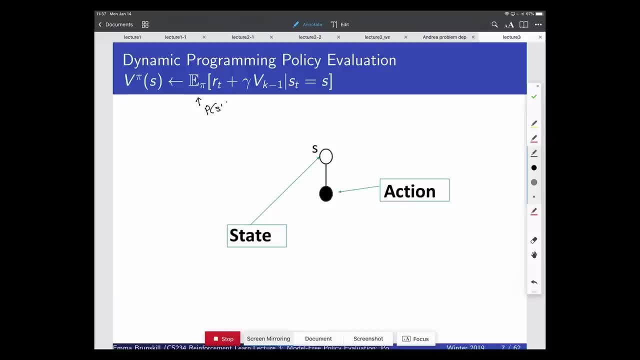 what's that expectation over? It's going to be the probability of s prime given s pi of s OK. so how do we think about this graphically? Well, we start in this state, We take an action And then we think about the next states that we could reach. We're again assuming that. 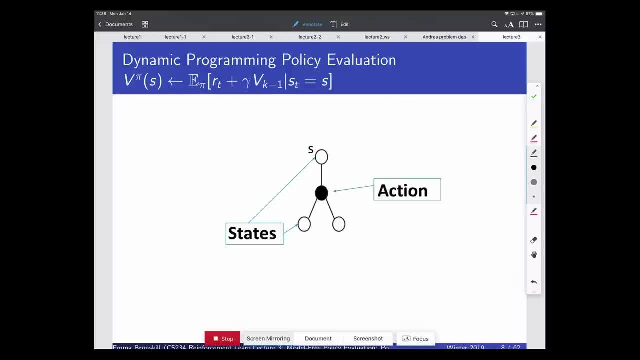 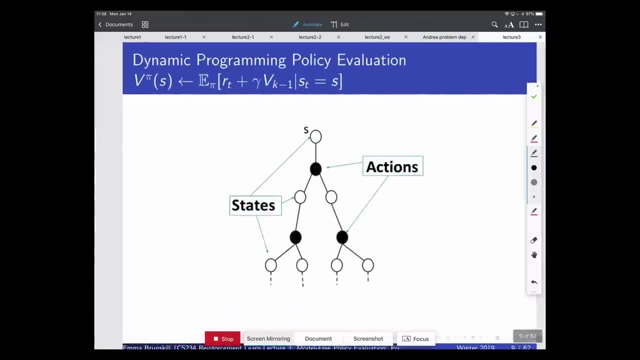 we're in a stochastic process so maybe sometimes the red light is on and sometimes the red light is off. So, depending on that, we're going to be in a different next state. We're trying to drive to the airport And then we can think about after we reach that state. then we could take some other. 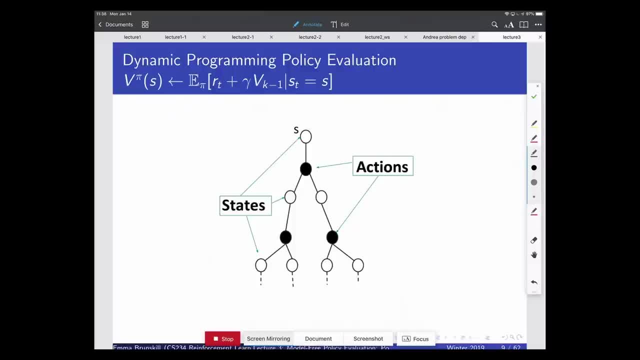 actions And in particular, we could take one action in this case, because we're assuming we're fixing what the policy is And then from those, those actions would lead us to other possible states. three of trajectories that we might reach if we start in a state and start following our policy. 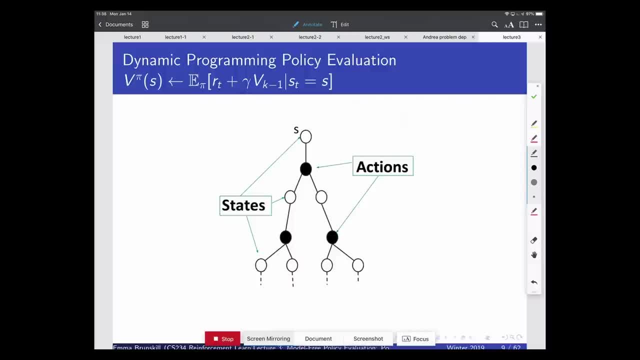 Where, whenever we get to make a choice, there's a single action we take because we're doing policy evaluation, And whenever there's sort of nature's choice, then there's like a distribution over next states that we might reach. You can think of these as the S primes and the S double primes. 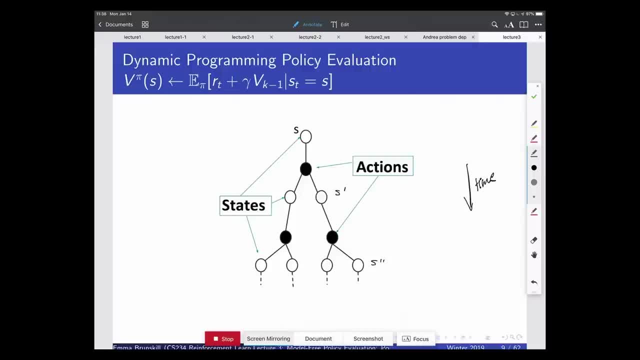 kind of times going down like this. All right. So this is sort of you know the- the potential futures that your agent could ar- arise in, And I think it's useful to think about this graphically, because then we can think about how those potential futures 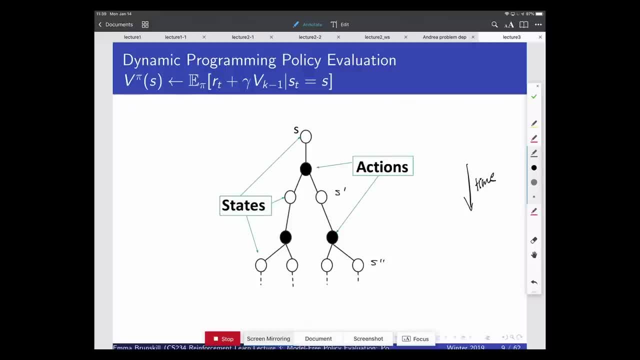 how we can use those to compute what is the value of different- of this policy. So, um, in what dynamic program? what we're doing- and in general we're trying to compute the value of a policy- is we're going to take an expectation over next states. 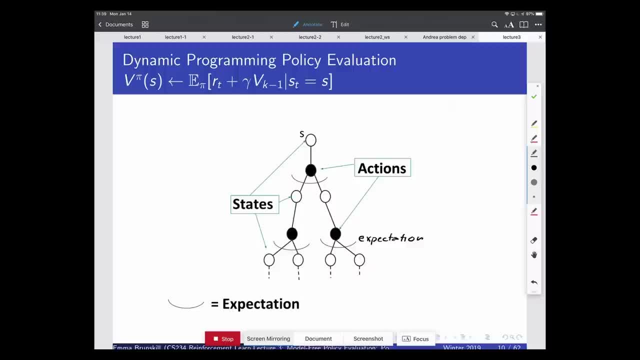 So the value is the expected discounted sum of future awards if we follow this policy and the expectation is exactly over these values. So the value is the expected discounted sum of future awards if we follow this policy and the expectation is exactly over these values. 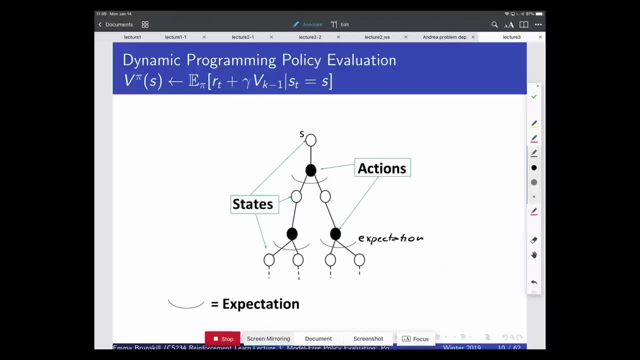 So the value is the expected discounted sum of future awards if we follow this policy and the expectation is exactly over these values, distributions of futures. So whenever we see an action and then we think about all the next possible nodes we could get to, 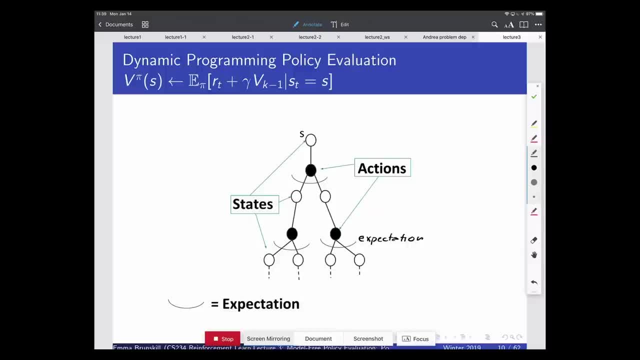 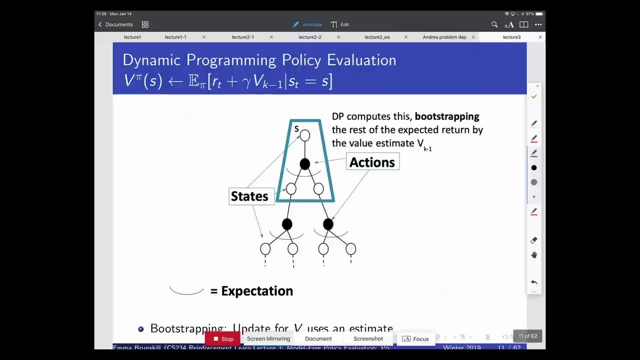 we want to take an expectation over those futures, an expectation over all the rewards that we could get. So that's what dynamic programming is- or that's what we can think of this graph as doing. And when we think about what dynamic programming is doing, 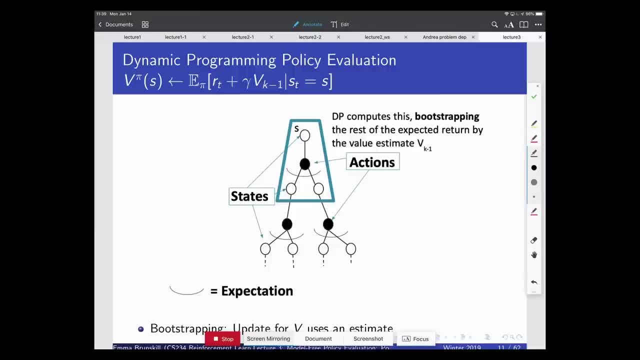 is. it estimates this expectation over all those possible futures by bootstrapping and computing a one-time step expectation, exactly. So what does does it do? again? It says: my b pi of s is exactly equal to r of s pi of s, my immediate reward. 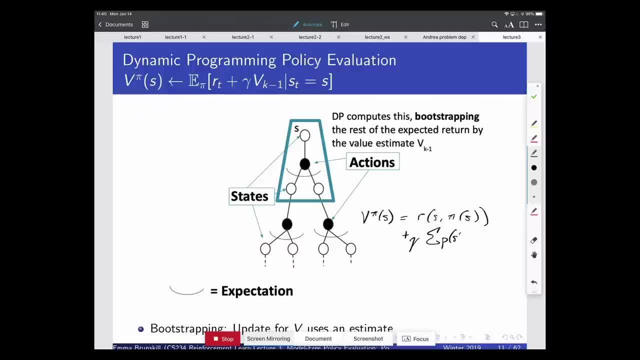 plus gamma sum over probability of s prime, given s a, b, pi k minus 1 of s prime. So it bootstraps- and we're using the word bootstraps there because it's not actually summing up all of these lower down potential rewards. 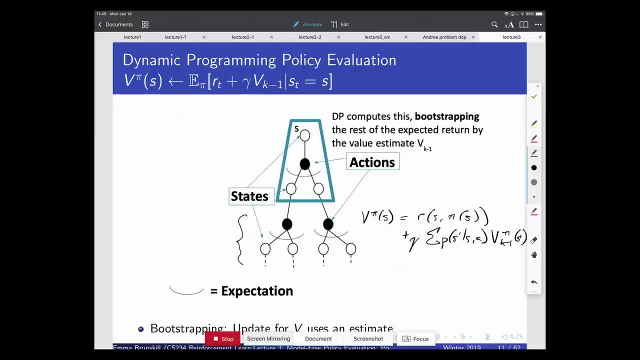 It's saying I don't need to do that. Previously I computed what it would be like if I started, say, in this state, and continued on for the future, And so I- now I already know what the value is of that state. 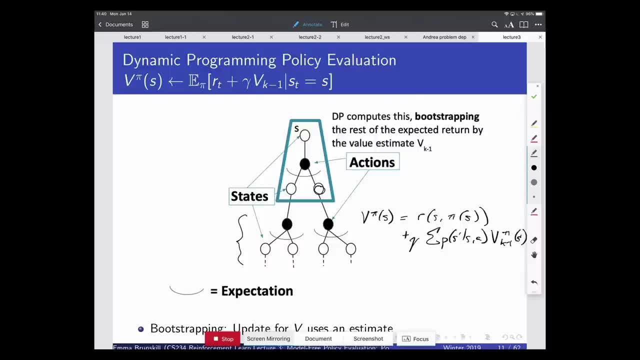 I'm going to bootstrap and use that as a substitute for actually doing all that rollout, And also here because I know what the expected discount is, or I know what the um sorry, the model is that I can also just take a direct expectation of s prime. 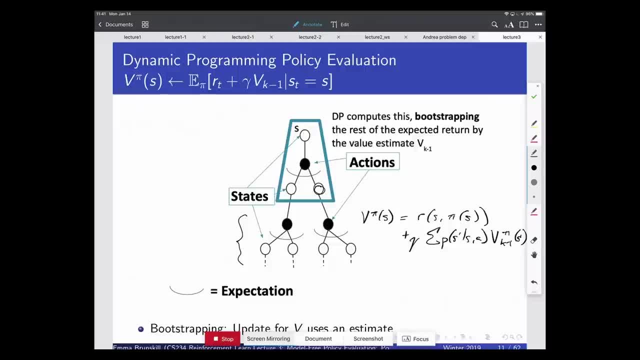 So my question is: is there an implicit assumption here that the reward- at a given state, and thus the value function evaluated at a state, doesn't change over time? So like because you're using it from the prior iteration? So I think the question is saying um. 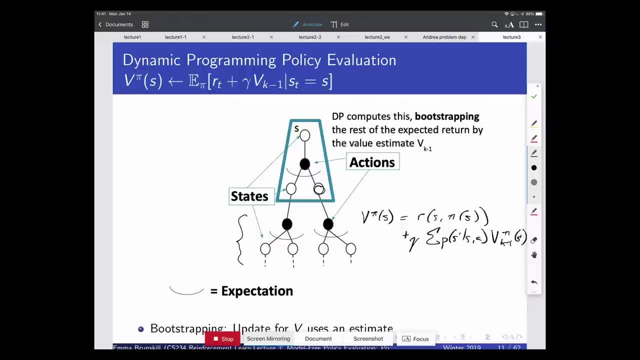 is there an explicit assumption here that the value doesn't change over time? Yes, The idea in this case is that the value that we're computing is for the infinite horizon case and therefore that it's stationary. It doesn't depend on the time step. 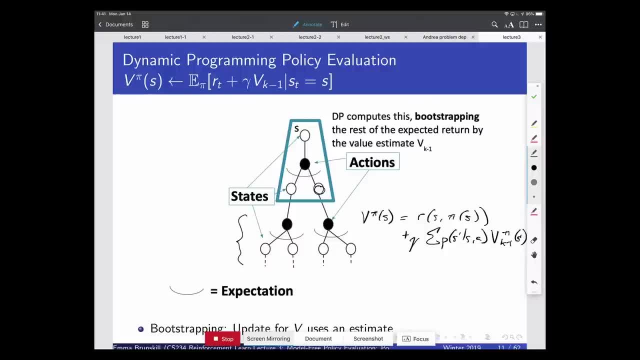 From that way, we're not going to talk very much about the finite horizon case today. In that case it's different. In this situation, we're saying at all all time steps. you always have an infinite number of more time steps to go. 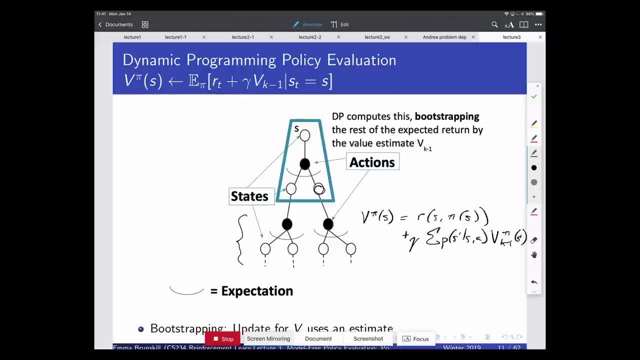 So the value function itself is a stationary quantity. So why is this an okay thing to do, Like we're bootstrapping? Um, the reason that this is okay is because we actually have an exact representation of this Vk minus one. You're not getting any approximation error of putting that in instead of. 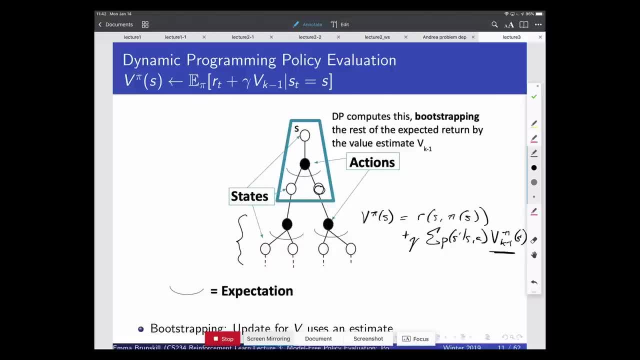 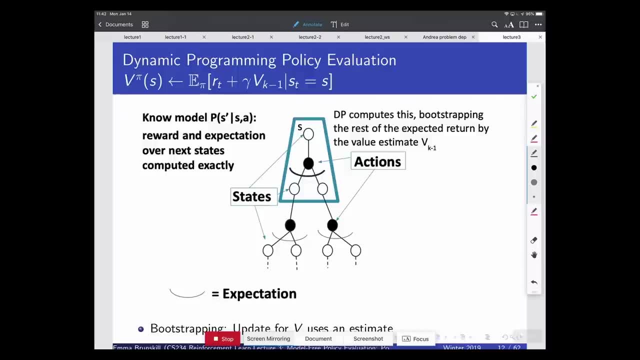 sort of explicitly summing over lots of different histories- Sorry, lots of different future rewards. So when we're doing dynamic programming, the things to sort of think about here is if we know the model, the know the dynamics model and know the reward model. 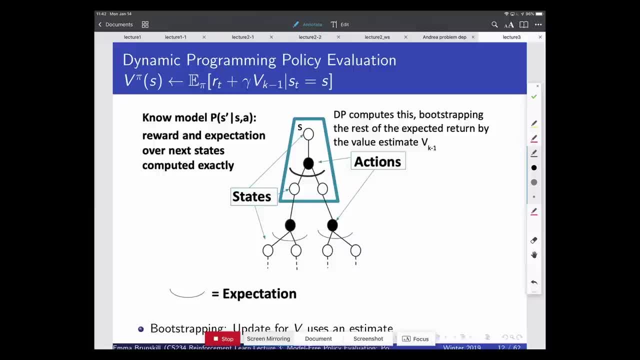 then we can compute the immediate reward exactly, We can compute our expected sum over future states exactly, And then we substitute in- instead of thinking about- we- instead of thinking about expanding this out as being a sum over rewards, we can just bootstrap and use our current estimate of Vk minus one. 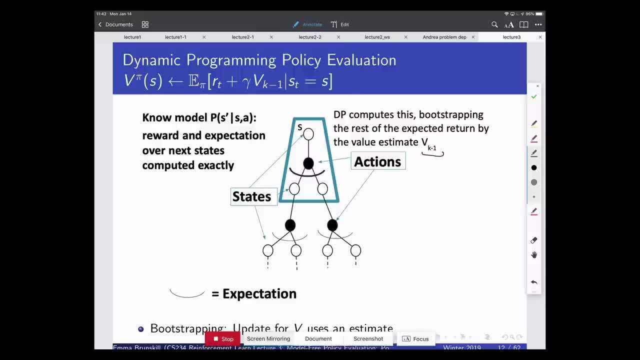 And the reason that I'm emphasizing this a lot is that when we start to look at these other methods, like Monte Carlo methods and TD methods, they're not gonna do this anymore. They're gonna do other forms of approximation, of trying to compute this tree. 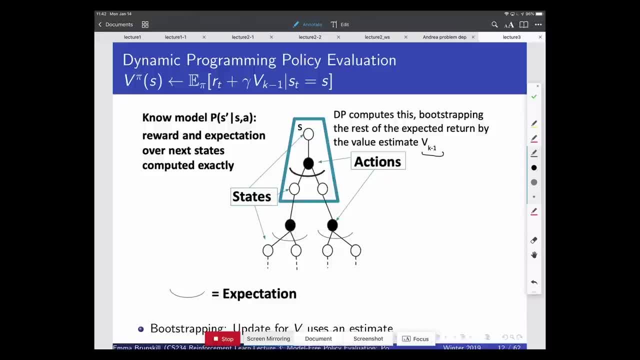 So, ultimately, to compute the value of a policy, what we're essentially doing is we're thinking about all possible futures and what is the return we'd get under each of those futures, And we're trying to make it tractable, to compute that. 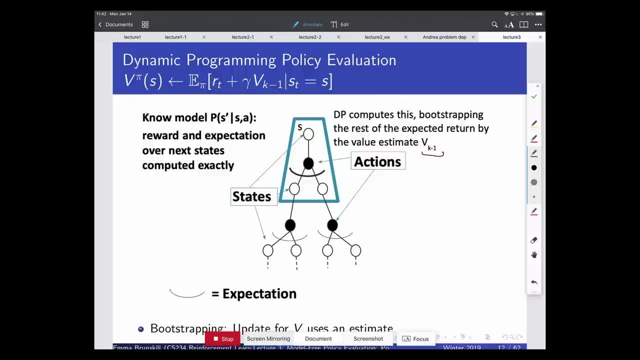 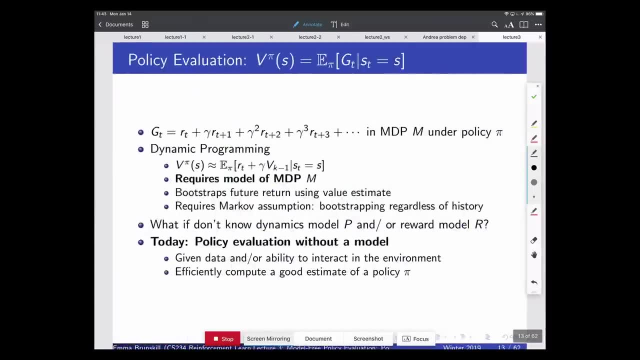 particularly when we don't know how the world works and we don't have access to the dynamics model or the reward model. Okay, Okay, Okay, Okay, Okay. So, just to summarize, dynamic programming, which we talked a little- a little bit about last time. 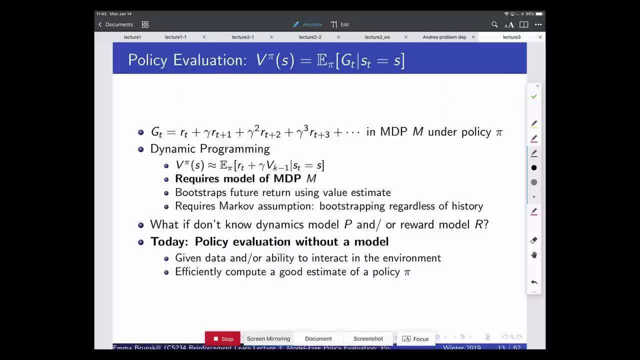 but we didn't really talk about the bootstrapping aspect. Dynamic programming says the value of a policy is approximately equal to the expected. next, the expectation over Pi of the immediate reward plus Gamma times the previous value you computed, requires a model. It bootstraps the future return using an estimate. 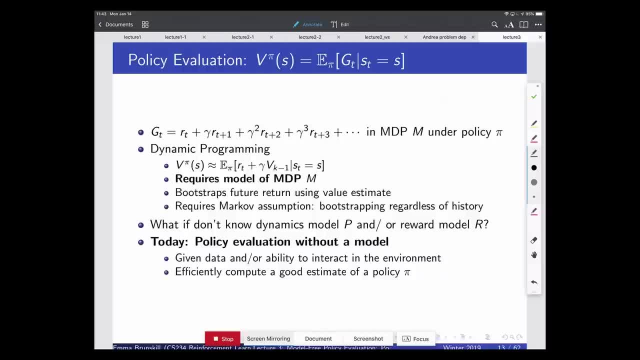 using your Vk minus one Um, and it requires the Markov assumption. And what- what I mean by that? there is that um, you're not thinking about all the paths you got to which will reach a certain state. You're saying: no matter how I got to that previous state. 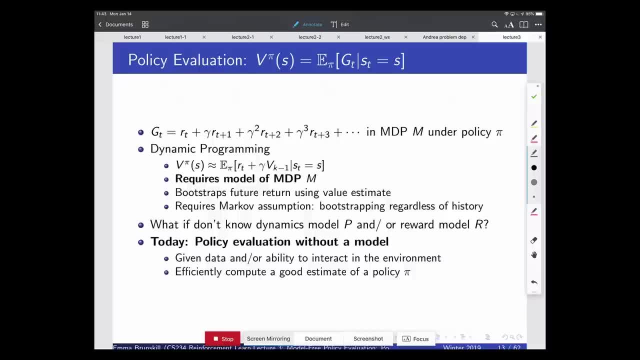 my value of that state is identical. um, and I can sort of assume that- and I can compute that singly based on the current observation. So we have any questions about this. So right now we sort of- it's mostly a recap of last time. 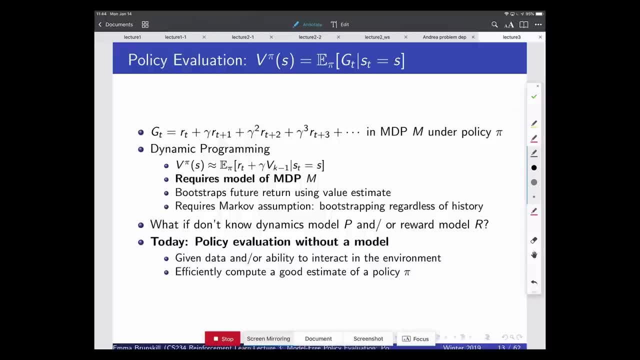 um, but sort of slightly pointing out some things that I didn't point out before, Okay, Okay. So those things are useful now that we're going to be talking about policy evaluation without a model. So what we're going to talk about now is Monte Carlo: policy evaluation. 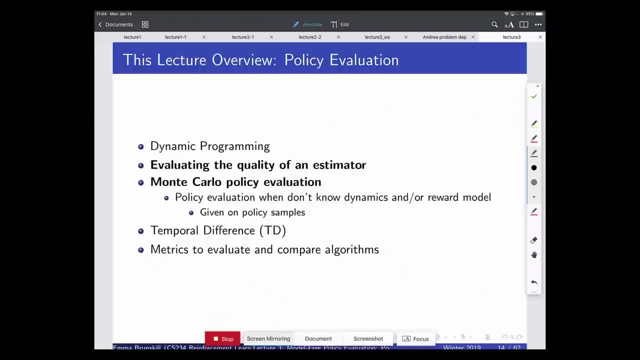 which is something that we can apply when we don't know what the models are of the world, And we're going to talk a little bit about how we can start to think about comparing these different forms of estimators: estimators of the value of a policy. 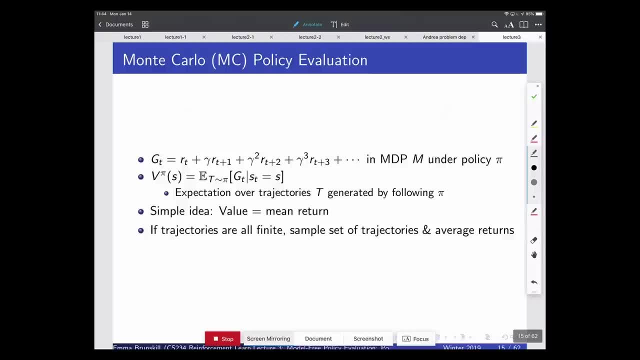 So in Monte Carlo policy evaluation, um, we can again think about the return. So the return again gt, our discounted sum of future rewards under a policy, And the value of a policy we can represent now is just let's think about all the possible trajectories we could get. 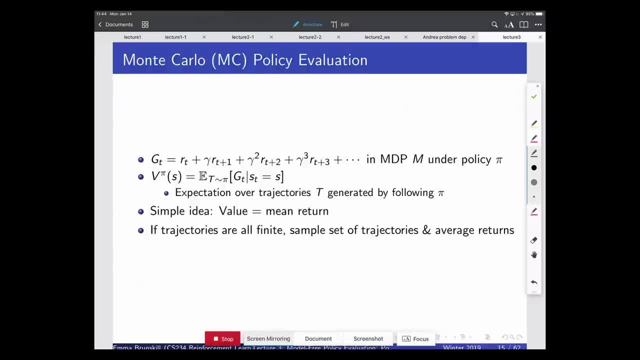 um, under our policy, and let's average all their returns So we can again think about that tree we just constructed. Each of those different sort of branches would have had a particular reward. um, and then we're just going to average over all of them. 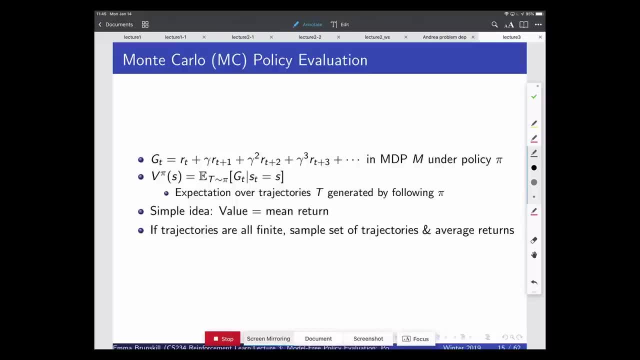 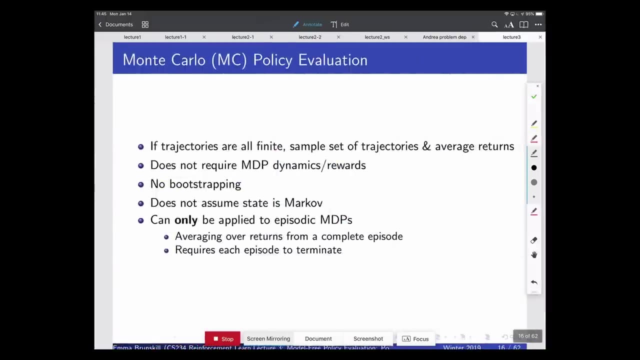 So it's a pretty simple idea. The idea is that the value is just equal to um, your expected return, And if all your trajectories are finite, you just can take a whole bunch of these and you average. So the nice thing about Monte Carlo policy evaluation is it doesn't require you to. 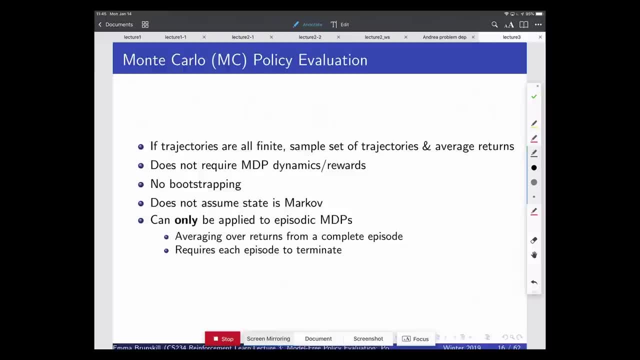 have a specific model of the dynamics or reward. It just requires you to be able to sample from the environment. So I don't need to know a particular, like parametric, model of how traffic works. All I have to do is drive from. 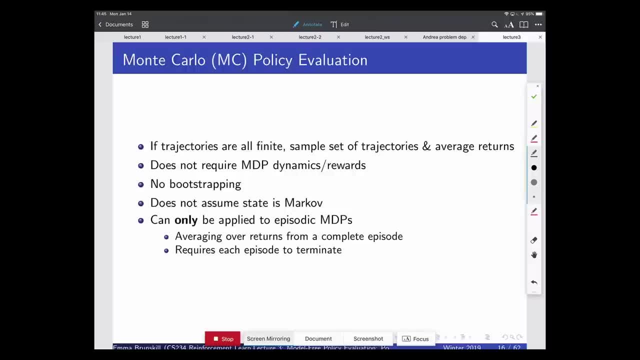 here to the airport, you know hundreds of times, and then average how long it takes me. And if I'm always driving with the same policy, let's say I always take the highway. um then if I do that, you know. 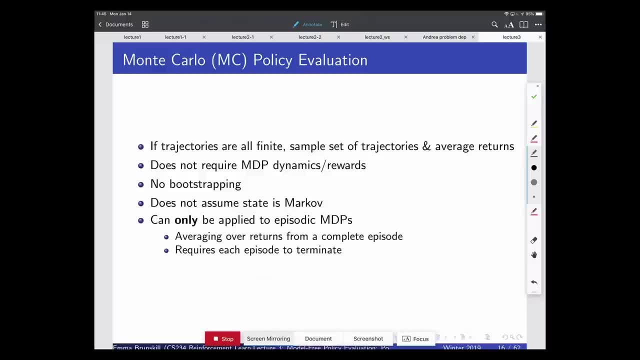 a hundred times, then I have a pretty good estimate of what is my expected time to get to the airport if I drive on the highway. So that is my policy. It doesn't do bootstrapping, It doesn't try to maintain at this room. vk minus one. 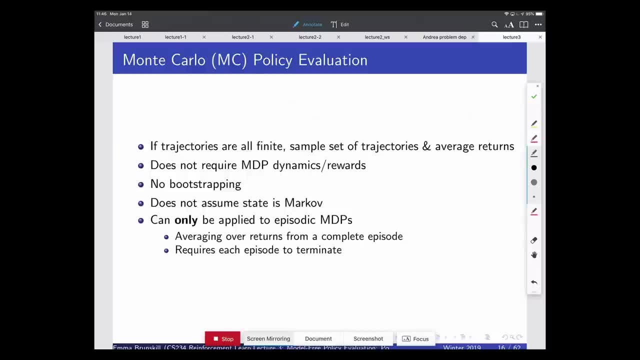 Um, it simply sums up all the rewards from each of your trajectories and then averages across those. Okay, It doesn't assume the state is Markov, It's just averaging. It doesn't- there's no notion of the next state and whether or not that's. 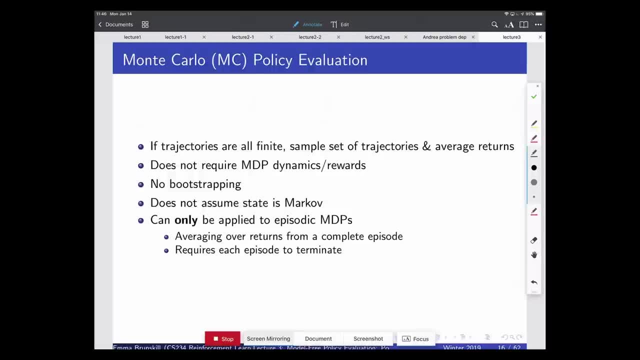 sufficient to um. to summarize: the future returns. An important thing is that it can only be applied to what are known as episodic MDPs. If you act forever, if there's no notion of um, if this is sort of like averaging over your life, 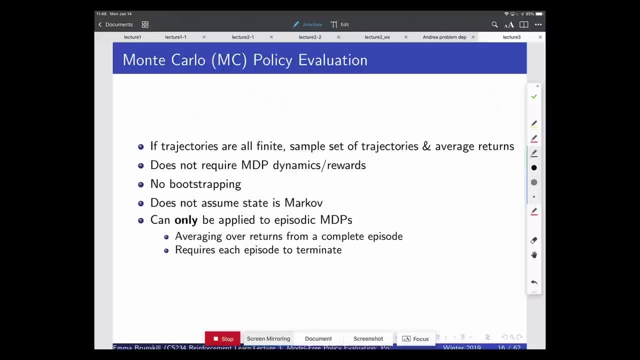 this doesn't work because you only get one. So you need to have a process where you can repeatedly do this many times And the process will end each time. So like driving to the airport might be really long, but you'll get there eventually and then you can try again tomorrow. 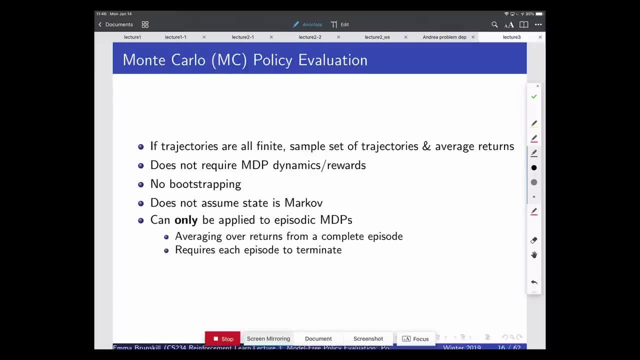 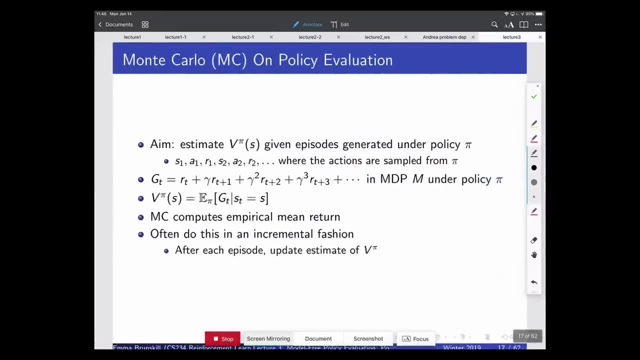 So this doesn't work for all processes, Like if you have a robot that's just going to be acting forever, you can't do Monte Carlo policy evaluation Okay. So we also often do this in an incremental fashion, which means that after we maintain a running estimate, 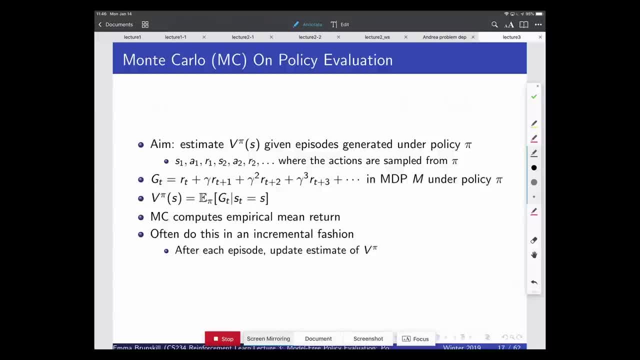 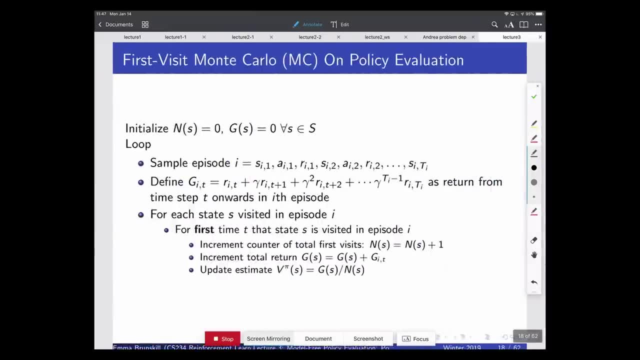 after each episode, we update our current estimate of v? pi, And our hope is that as we get more and more data, this estimate will converge to the true value. So let's look at um what the algorithm for this would be. 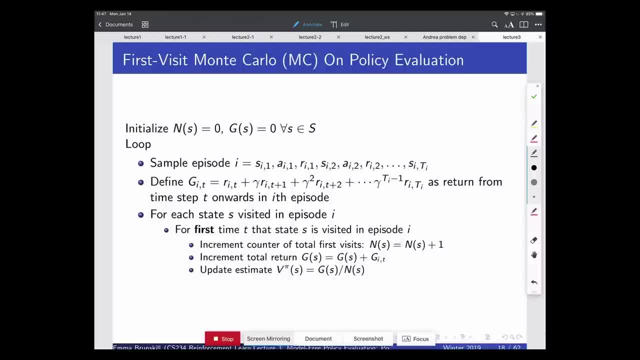 So one algorithm, which known- is known as the First Visit Monte Carlo on Policy Evaluation Algorithm: As we start off, then we assume that we haven't- and here is essentially the number of times we visited this state. So we start off and this is zero. 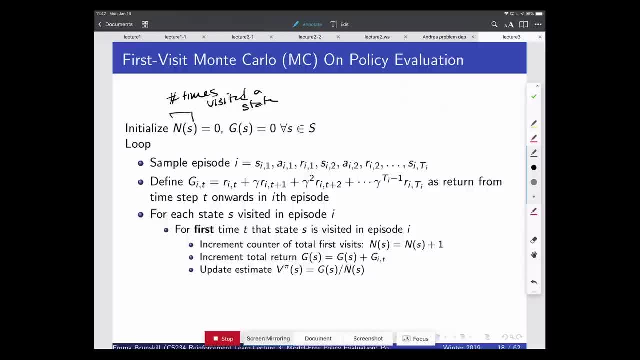 Also the return. our average return from starting in any state is also zero. So we initialize, say right now, or we think that you know, we get no reward from any state and we haven't visited any state. And then what we do is we loop, And for each loop 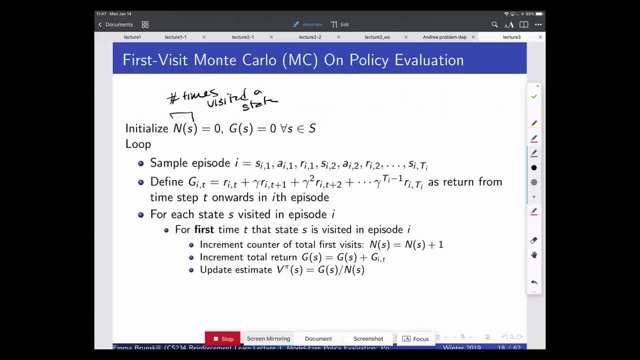 we sample an episode which is we start in a starting state and we act until our process terminates. I start off in my house and I drive until I can get to the airport And then I compute my return So I say okay, well, maybe that took me two hours to get there. 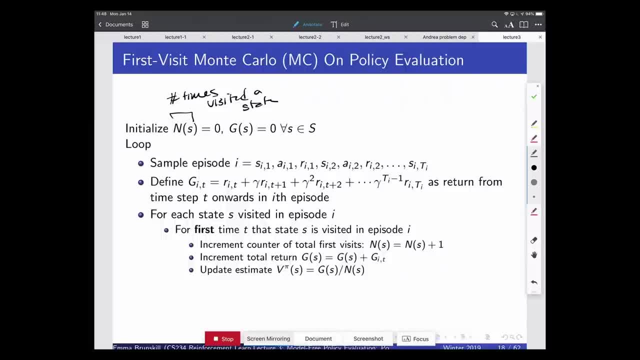 So now my GI is two hours, But you just compute your return and you compute it for every time step T inside of the episode. So GIT here is defined: from the T time step in that episode. what is the remaining reward you got from that time step onwards, And we'll instantiate this. 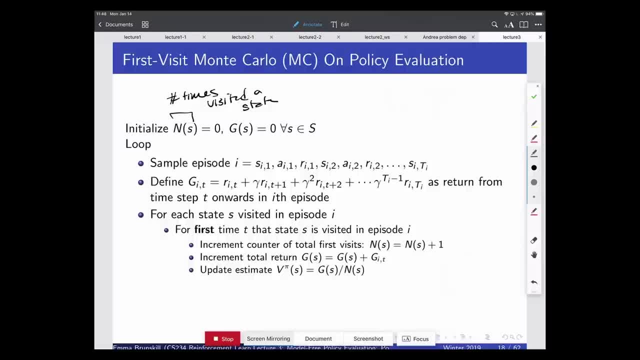 in our Mars rover example, in a second, And then for every state that you visited in that particular episode, for the first time you encountered a state, you increment the counter and you update your total return And you use- then you just take an average of those estimates to- 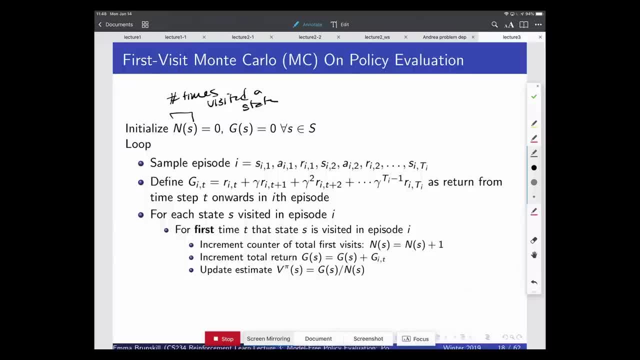 compute your current estimate of the value for the state Now why you might be in the same state for more than one time step in an episode. Well, let's say I get to the red light. Let's say I've discretized my time steps so I look at my state every one minute. Well, I got to a red light. 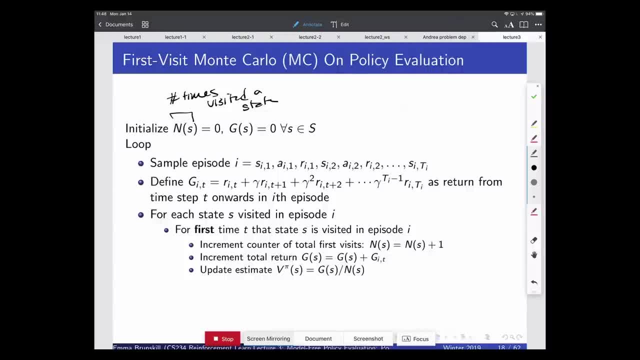 and there was a traffic accident. So, on time step one: I'm at the red light. On time step two, I'm on the red light. Time step three: I'm on the red light, And so you can be in the same state for multiple time steps during the episode. And what this is? 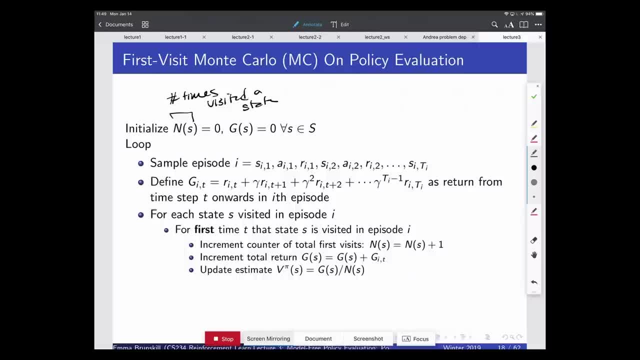 saying is that you only use the first time step. you saw that state and then you sum up the rewards. you get till the end of that episode. Okay, So if we saw the same state but in, I guess, like different time steps in the same episode, we'd still increment twice because it's not. 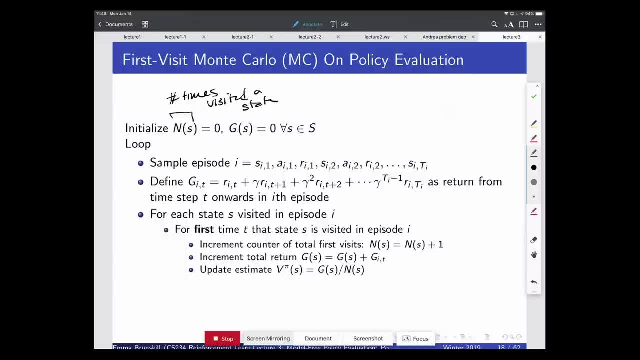 like there could be a gap. The question is about what happens if we see the same state in the same episode In first visit. you only use the first occurrence, So you drop all other ones. So the first time I got to my red light, then I would sum up the future rewards till the end of: 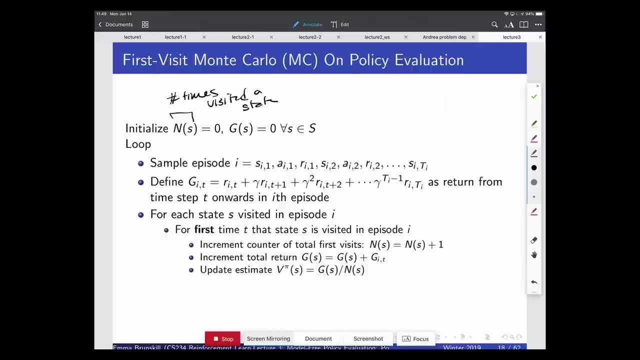 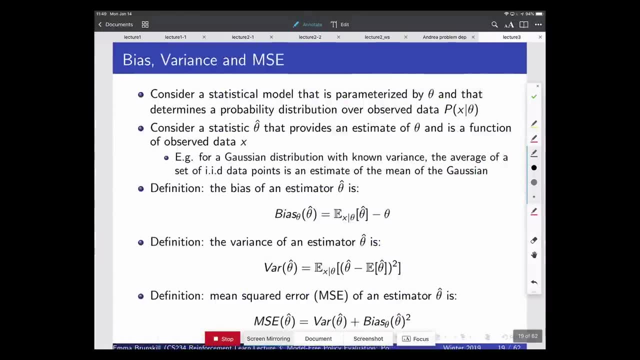 the episode. If I happen to get to the same red light during the same episode, I ignore that data. We'll see a different way of doing that in a second. Okay, So you know. how do we estimate whether or not this is a good thing to do? How do we evaluate whether or not this particular 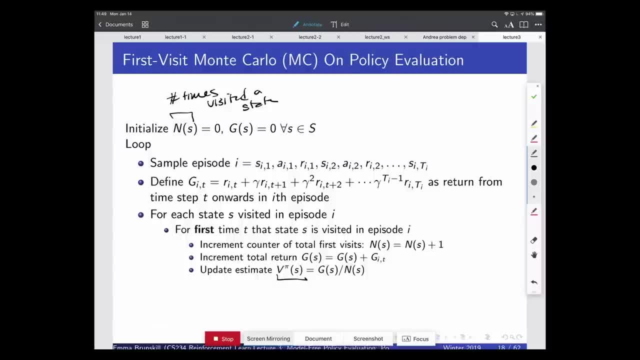 this is an estimate. It's likely wrong, at least at the beginning, when we don't have much data. So how do we understand whether or not this estimate is good and how are we going to compare all of the estimators and these algorithms that we're going to use? So 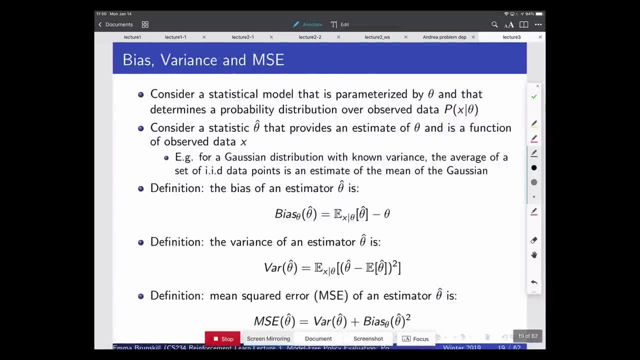 actually just raise your hand because I'm curious. Um, who here has sort of formally seen definitions of bias and variance in other classes? Okay, Most people, but not quite everybody. So just as a quick recap, um, let's think about sort of having a statistical model. 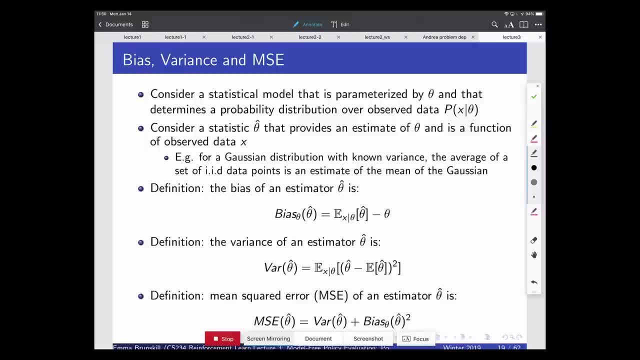 that is parameterized by theta um and that we also have some distribution over some observed data. p of x, given theta. So we want to have a statistic theta hat, which is a function of the observed data. So theta hat is a function of the observed data and it provides an estimate. 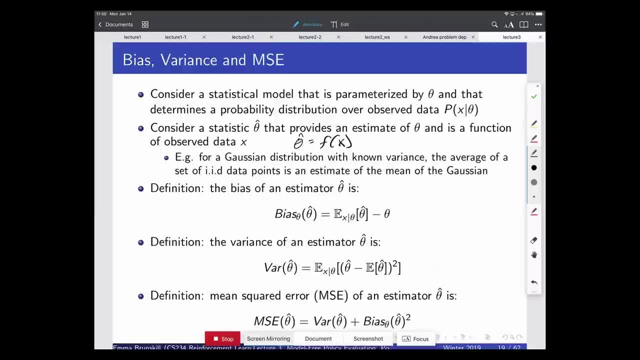 of theta. So in our case, we're going to have this value, this estimate of the value we're computing. This is a function of our episodes and this is an estimate of the true discounted expected rewards of following this policy. So the definition of a bias of an estimator. 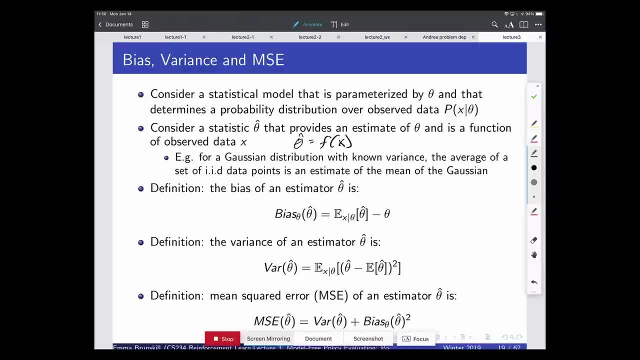 is to compare what is the expected value of our statistic versus the true value For any set of data. So this would say: if I compute, you know the expected amount of time for me to get to the airport, based on trying to drive there three times. does the 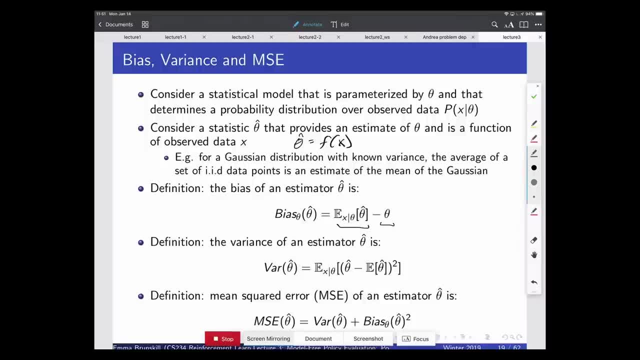 algorithm that I just showed you. is that unbiased? On average, is that the same as the true amount? expected time for me to get to the airport? The definition of a variance of an estimator compares my statistic to its expected value, squared expected over the. 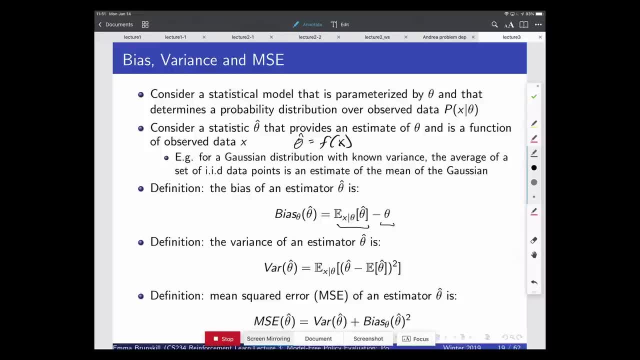 the um the type of data I could get under the true parameter And the mean squared error combines those two. Mean squared error is normally what we care about. Normally we ultimately care about sort of how far away is our estimate of the quantity we care about versus the true quantity. 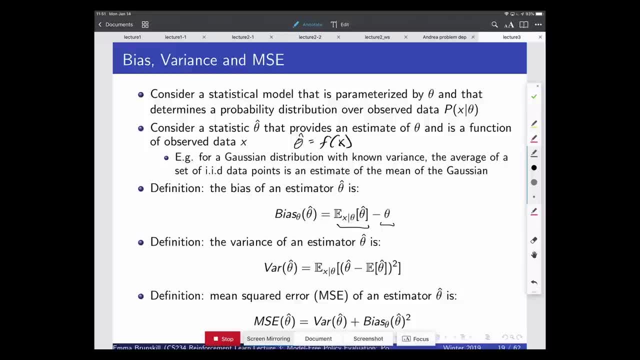 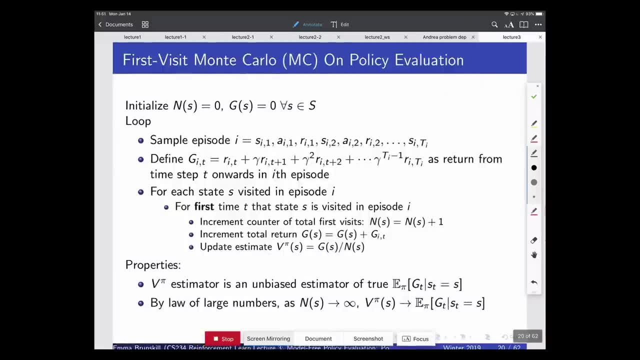 And that's a sum of its bias and its variance, And generally, different algorithms and different estimators will have different trade-offs between bias and variance. Okay, So if we go back to our first visit, Monte Carlo algorithm, the V pi estimator that we use there is: 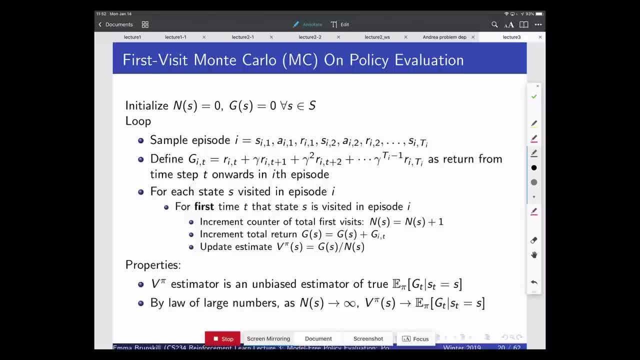 an unbiased estimator of the true expected discounted sum of rewards from our policy. It's just a simple average um and it's unbiased And, by the law of large numbers, as you get more and more data, it converges to the true value. 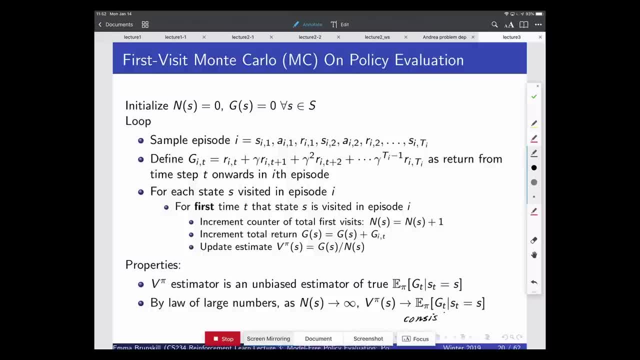 So it's also what is known as as consistent. Consistent means that it converges to the true value as the as data goes to infinity. So this is reasonable, um, but it might not be very efficient. So, uh, as we just talked about, 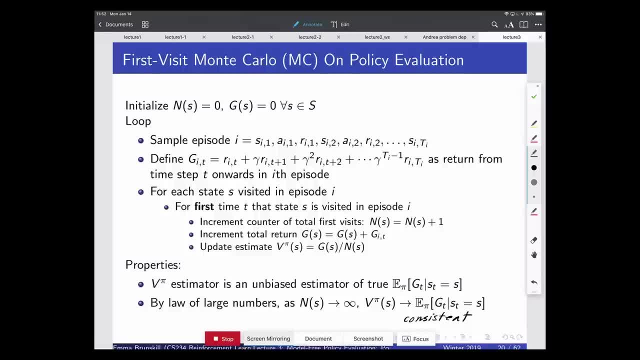 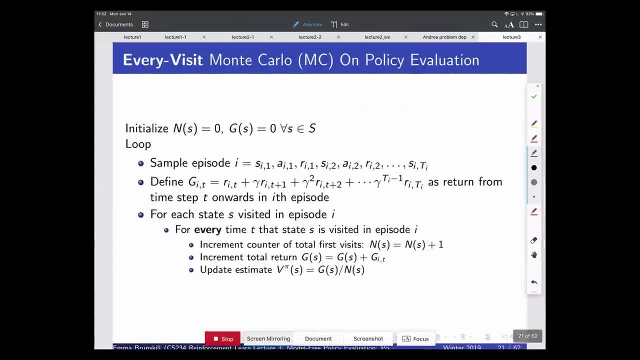 you might be in the same state, might be at the same stoplight for many, many time, steps um, and you're only gonna use the first state in an episode to update. So every visit at Monte Carlo simply says: well, every time you visit a state during the episode. 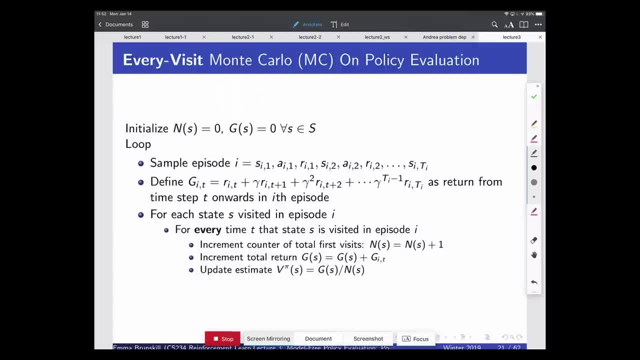 look at how much reward you got from that state till the end and average over all of those. So essentially, every time you reach a state you always look at the sum of discounted rewards from there to the end of the episode and you average all of that. 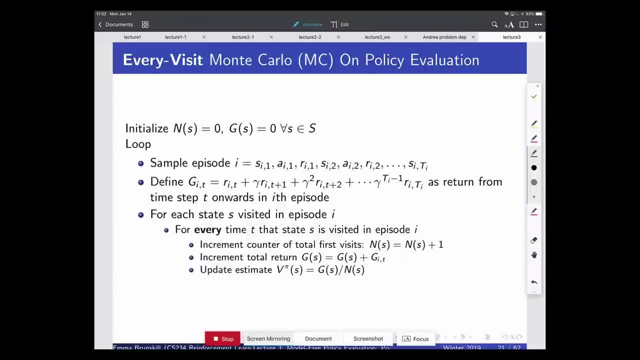 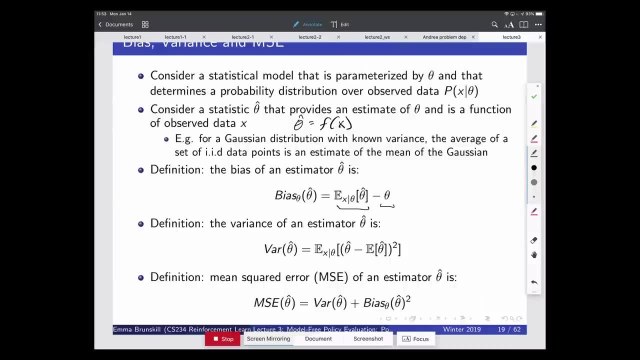 This is generally gonna be more data efficient. Back to the bias definition. I guess I'm just a little confused how we would uh get bias given that we don't actually know data. How do we compute bias? Yeah, given that we don't know data. 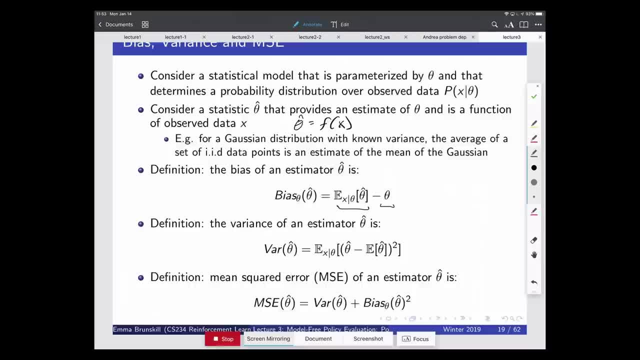 It's a great question is: how do you compute bias? Yes, if you, uh, if you can compute bias, exactly, that normally means you know what data is. in which case, why are you doing an estimator? Generally, we do not know what bias is. 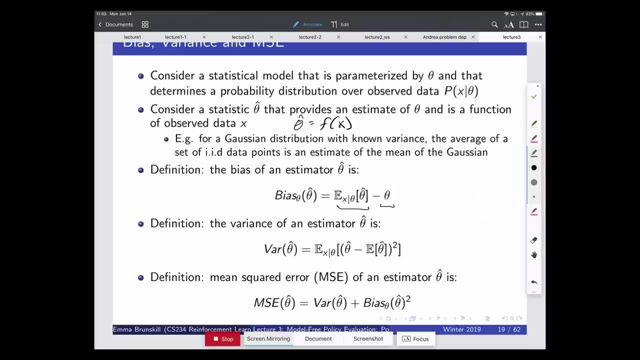 um, uh. we can often bound it So often using things like concentration inequalities. we can um well, concentration inequalities are more for variance. Often, um, we don't know exactly what the um bias is, unless you know what the ground truth is. 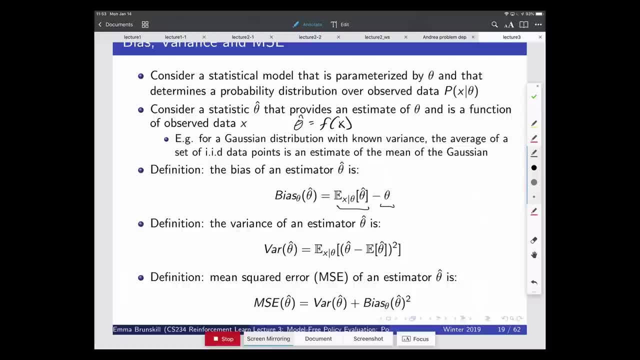 And there are different ways for us to get estimates of bias in practice. Sometimes you compare across different forms of parametric models. um, sometimes you can do structural risk, uh uh, structural mix maximization and things like that to try to get sort of a quantity of how you 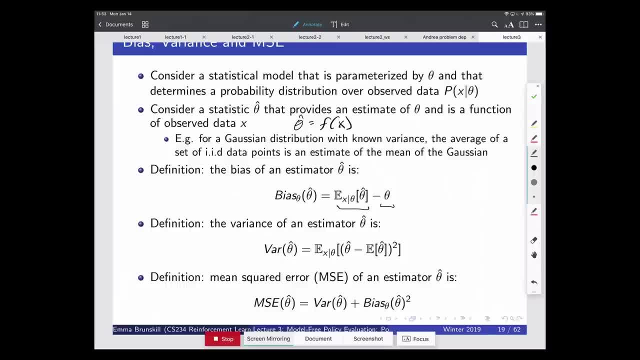 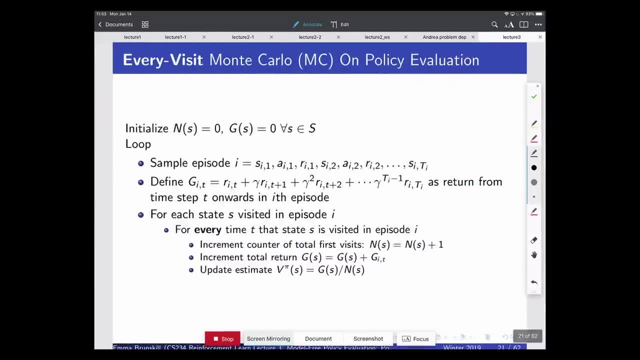 compare your estimator and your model class. I'm not gonna go very much into that here, but I'm happy to talk about it in off-sales. So in every visit Monte Carlo we're just gonna update it every single time and that's gonna give us another estimator. 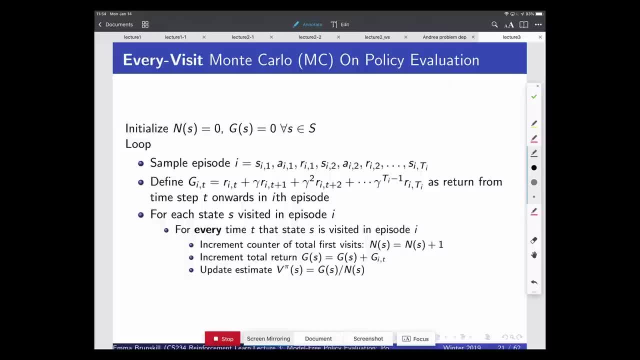 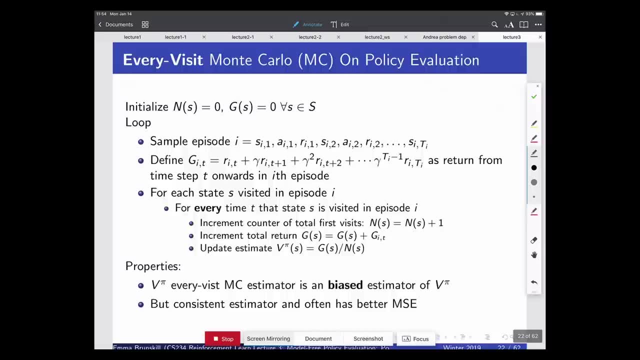 And note that that's gonna give us generally a lot more counts because, um, every time you see a state you can update the counts, but it's biased, So you can show that this is a bias estimator or V-pi. 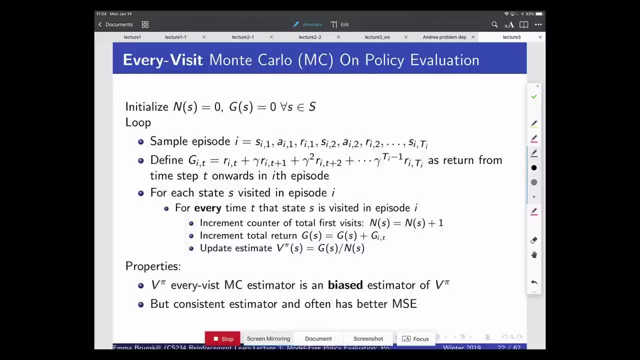 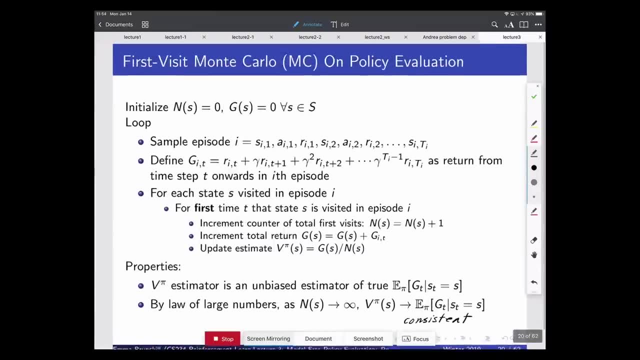 You may have an intuition of why it might be biased. So, in the first case, um. for those of you that have seen this before, um, or not necessarily this particular, but seen this sort of analysis, first visit Monte Carlo, um. 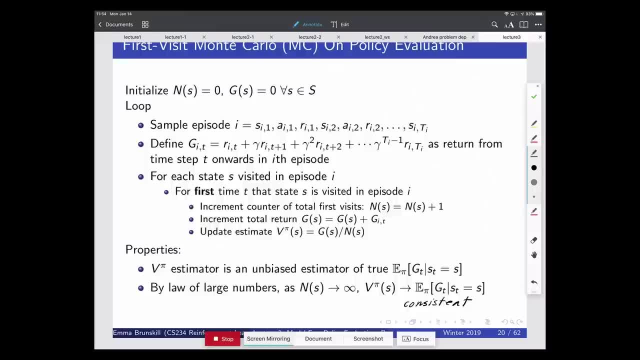 is you're getting iid estimates of a state, of a state's return. right Because you only take that um. each episode is um is iid because you're starting a starting state and you're you're estimating from there. um. 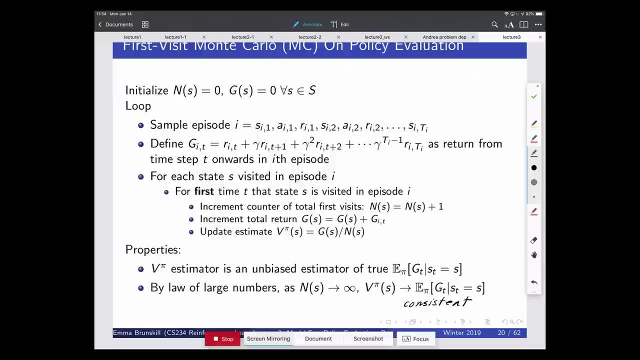 and you only use the return from the first time you saw that state. If you see a state multiple times in the same episode, are their returns correlated or uncorrelated? Correlated, right, So your data is no longer iid. So that's sort of the intuition for why, when you move to ev- move to every visit Monte Carlo. 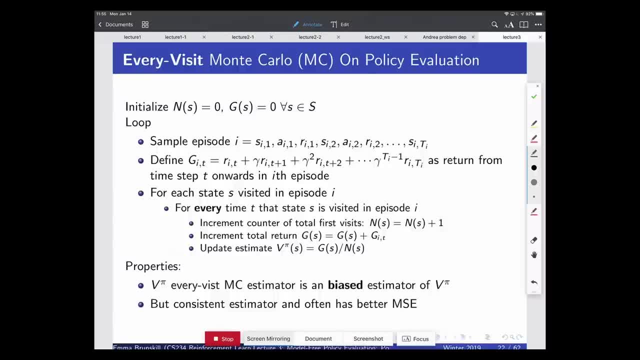 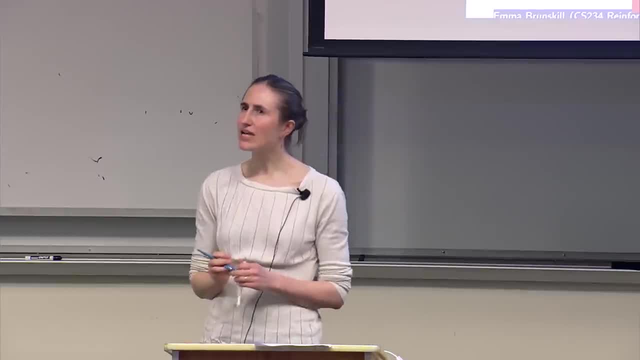 your estimator can be biased because you're not averaging over iid variables anymore. Is it biased for analogous reasons to inspectors? paradox: Is that the process of that? I don't know. That's a good question. I'm happy to look at it and return. 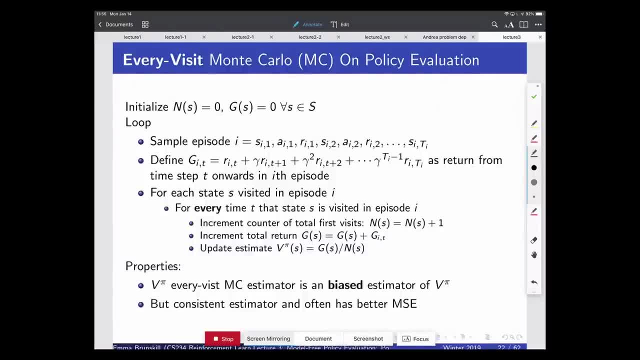 However, the nice thing about this is that it is a consistent- uh, consistent- estimator. So as you get more and more data, it will converge to the true estimate And empirically it often has way lower variance And intuitively it should have way lower variance. 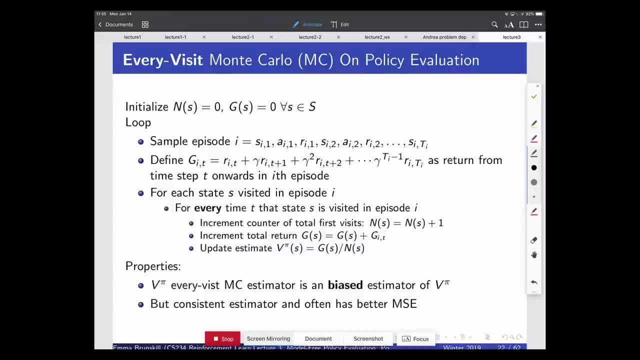 We're averaging over a lot more data points, um, typically in the same. Now you know if you only visit one- if you, if you're very unlikely to repeatedly visit the same state. these two estimators are generally very close to the same thing in an episode. 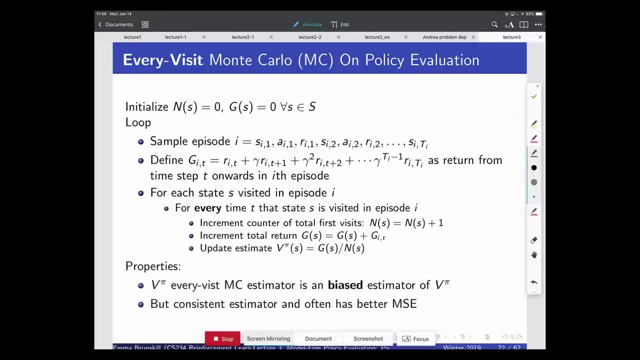 because you're not gonna have multiple visits to the same state, But in some cases you're gonna visit the same state a lot of times and you get a lot more data, And these estimators will generally be much better if you use every visit. 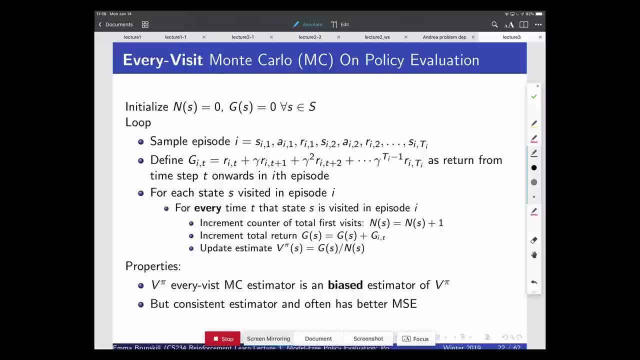 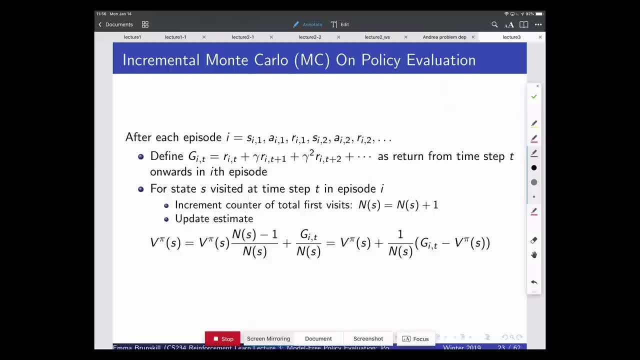 But it's biased. So there's this trade-off. Empirically, this is often much better Now, of course, in practice, often, instead of um the- often you may want to do this incrementally, Um, you may just want to kind of keep track of a running mean. 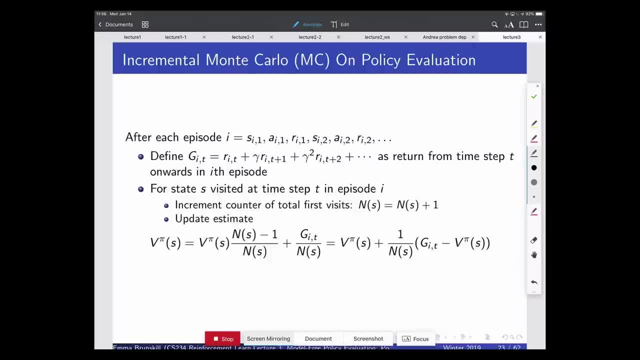 and then you, uh, keep track of your running mean and update your count, sort of incrementally Um, and you can do this also as you visit. You don't have to wait until the end of the-. oh, that's wrong. 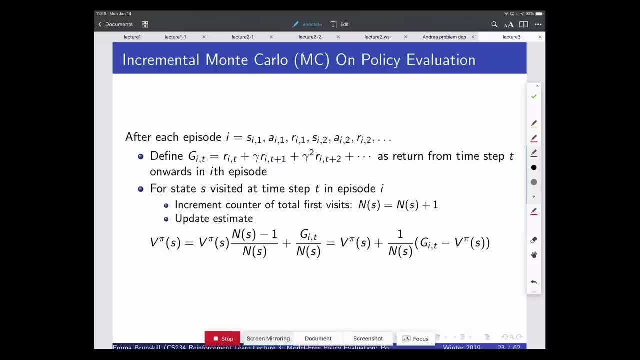 You do have to wait till the end, because you always have to wait till you get, uh, the full return before you can update, Yeah, in the back. Um, so a question on that, If you could like, if you condition on the fact that you have. 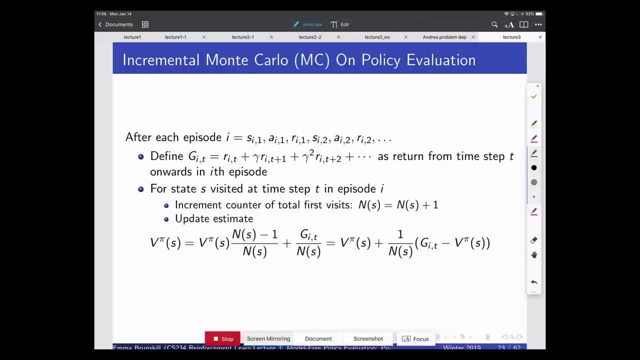 the same number of estimates approximately in each of the states. would then the two be more or less equivalent, but the other one would be less biased? For example, if you did, I guess there's no way that you could have, for example, running the same number of episodes at the same number of countries. 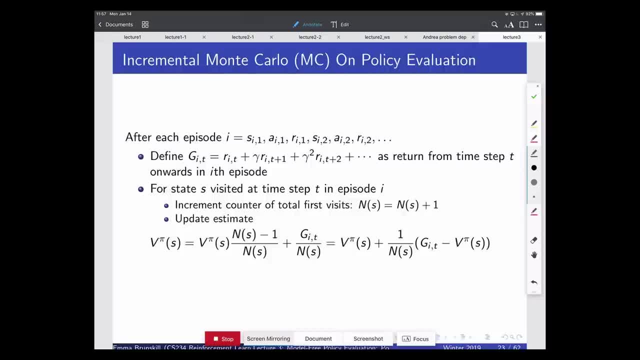 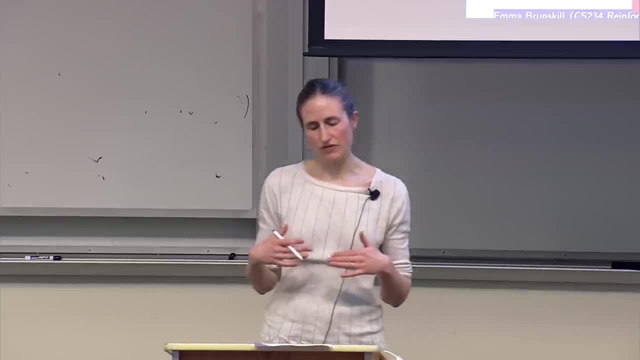 State with the first visit approximation. But if you did have that, would you imagine that the MSU would be lower in that case? I have a question about um. if you have the same number of counts to a state across the two algorithms. 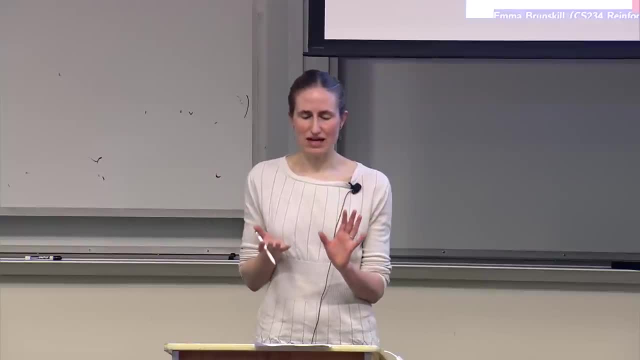 um and- and in terms of episodes. you couldn't have that be the case um unless-. so they'd either be identical if you only visit one state, um once in an episode, and then they'd be totally identical. 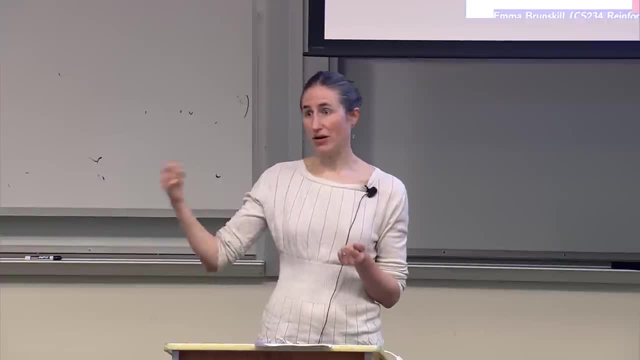 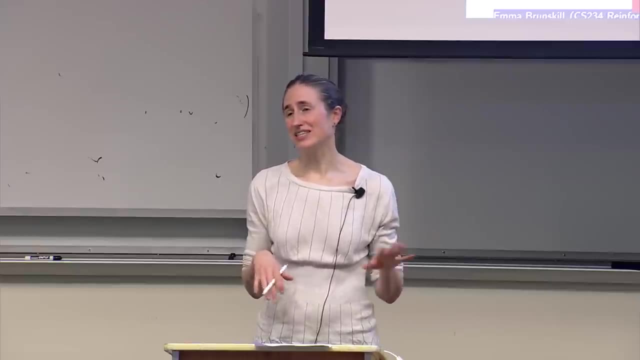 If it's not the case, if you visit um a state multiple times in- in one episode, then, uh, by the time you get to the same counts. the one for the single visit would be better because it's unbiased and it would have basically the same variance. 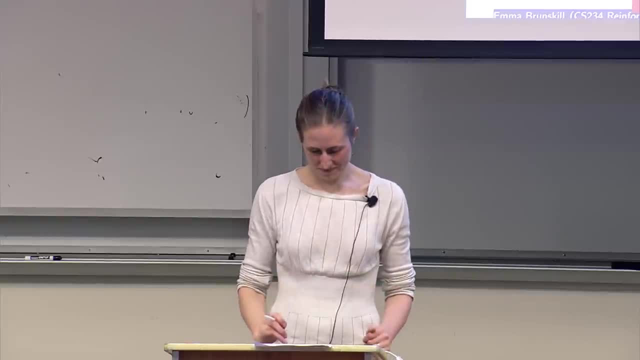 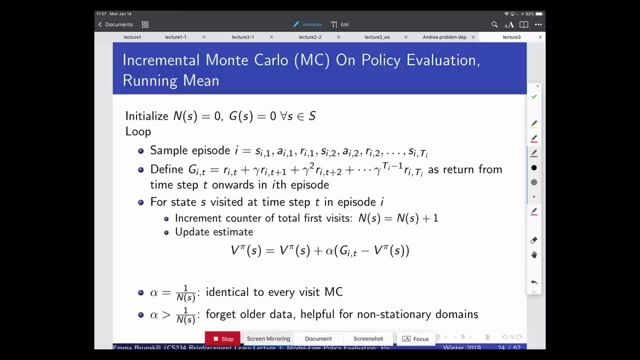 Any other questions about that? Cool Um. so incremental Monte Carlo um on policy evaluation is essentially the same as before, except for you can just sort of slowly move your running average for each of the states, And the important thing about this is that um. 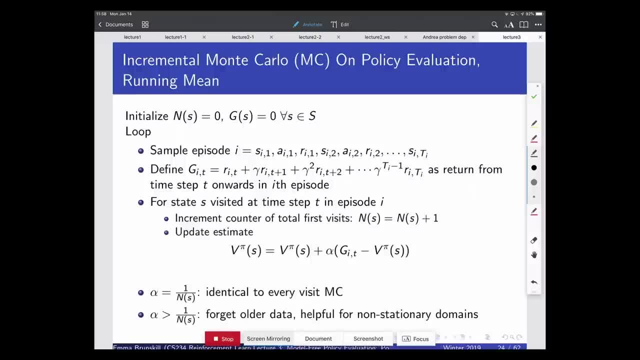 as you slowly move your estimator. if you set your alpha to be one over NS, it's identical to every visit Monte Carlo. Essentially, you're just exactly computing the average Um, but you don't have to do that, So you can slew it so that your running average is more weighted towards recent data. 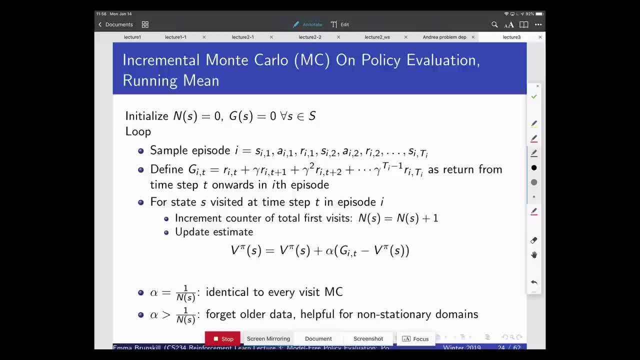 And the reason why you might want to do that is because, if your real domain is non-stationary, Let me have a guess of where- where- domains might be non-stationary. This is kind of an advanced topic. We're not gonna really talk about non-stationary domains for most of this class. 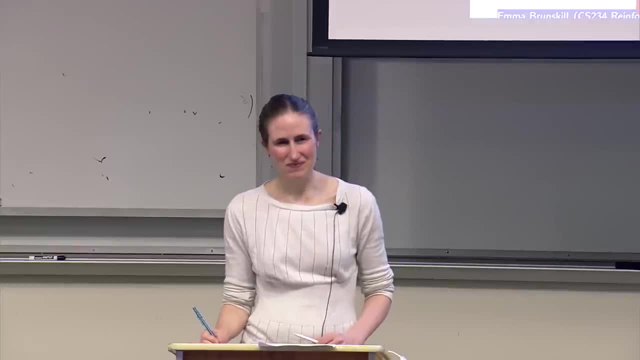 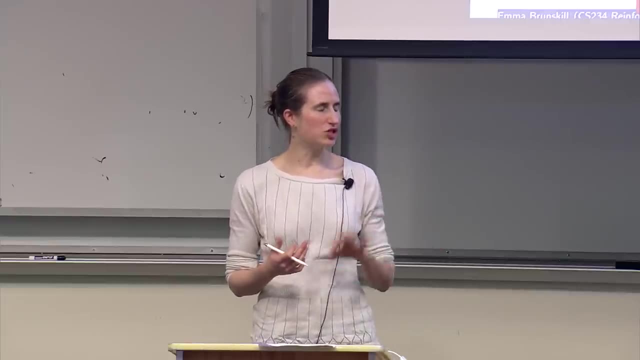 though in reality they're incredibly important. Um, I don't know if your mechanical parts are breaking down as time goes on. Example of like if you're in a manufacturing process and your parts are changing- are breaking down over time, so your dynamics model is actually changing over time. 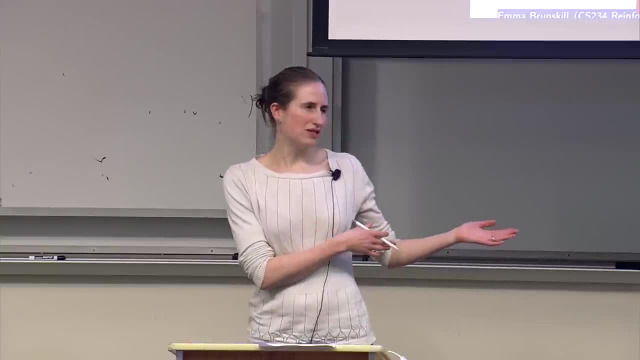 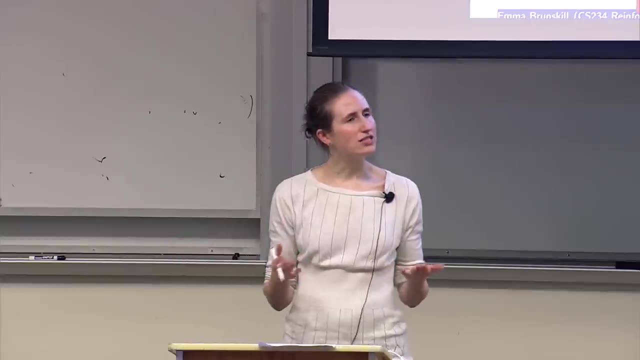 um, then you don't want to reuse your old data because you're actually- your MDP has changed over time, So this is one of the reasons, often empirically, like when people train recommender systems and things like that, you know. 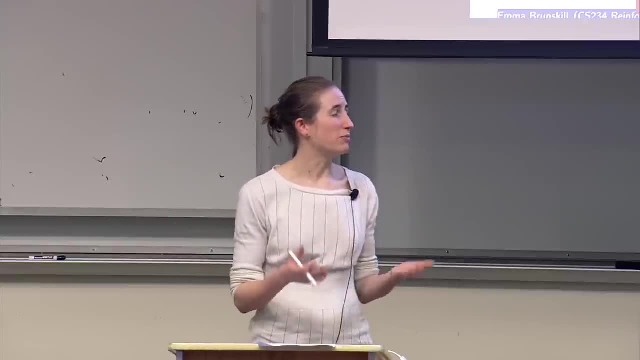 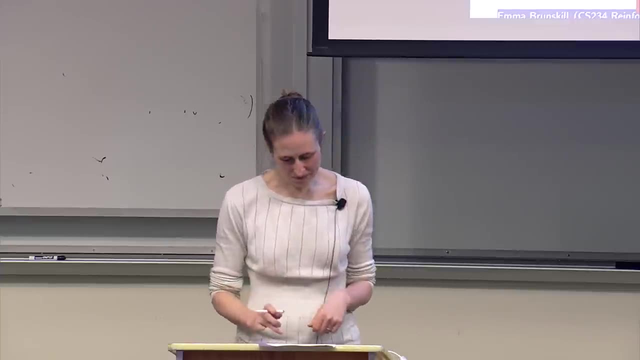 the- the news. all these things are non-stationary and so people often retrain them a lot to deal with this non-stationarity process. Do I see a question in the back? Okay, Yeah, So empirically, that's often really helpful for non-stationary domains. 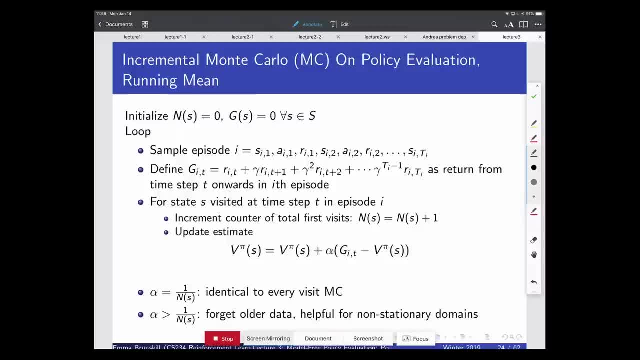 but if it's non-stationary, there's all- there's a bunch of different concerns, Um, so we're gonna mostly ignore that for now. Okay, So let's just check our understanding for a second For Monte Carlo, for on-policy evaluation. 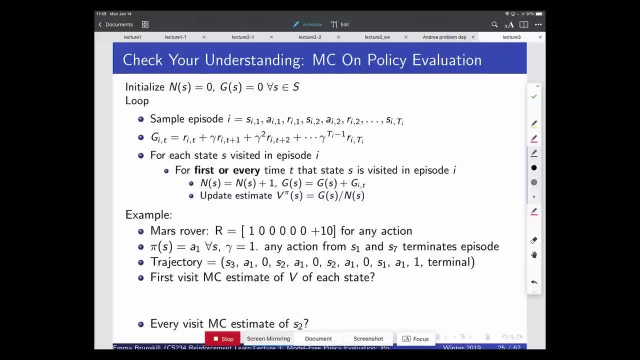 let's go back to our Mars Rover domain. Um. so in our Mars Rover we had these seven states um our rover dropped down. it was gonna explore. our reward is in state S1, 1, in state S7, it's plus 10,. 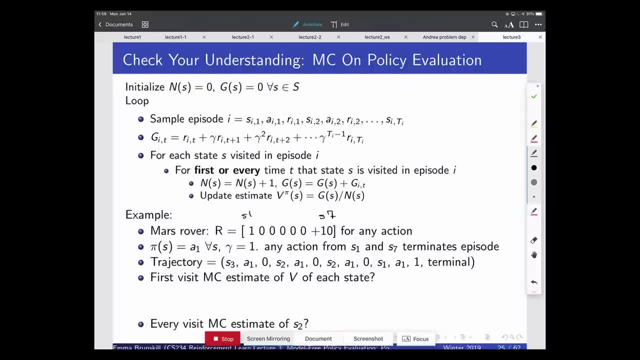 everywhere else it's 0, and our policy is gonna be A1 for all states. Um, and now imagine, we don't know what the dynamics model is, So we're just gonna observe trajectories, Um, and if you get to either state 1 or state 7,, 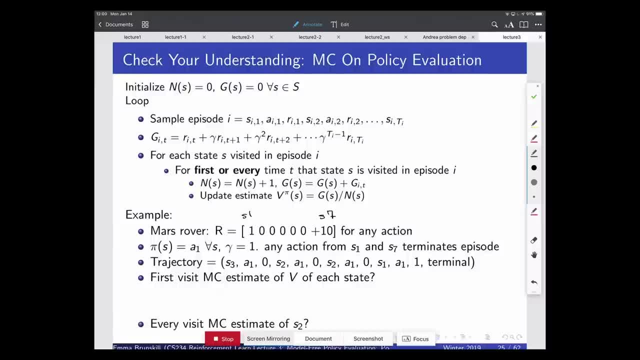 the next action you take terminates the reward. I don't know, maybe it falls off a cliff or something like that, But whenever you get to S-, S7 or S1, then the um the next action you take, so you get whatever reward. 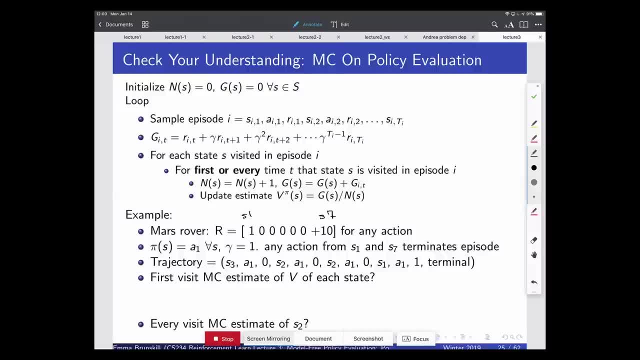 you either get the 1 or you get the 10, um, and then your process terminates. So let's imagine a trajectory under this policy would be: you start in S3, you go to action- you take action A1, you get a reward of 0. This is reward. 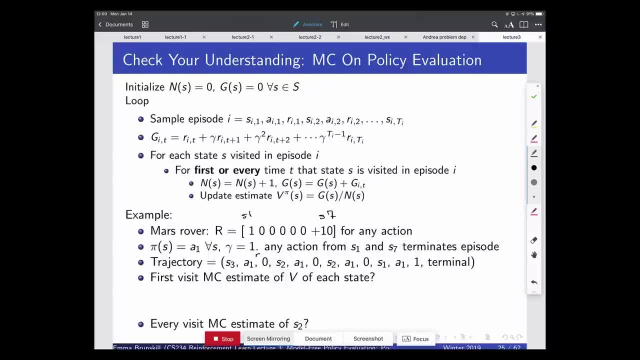 Then you transition to state S2, you take an action of A1, you get a 0. You stay in the same state. So you stay in S2 again, take action A1, you get another reward of 0, and then you reach state S1, take an action A1,. 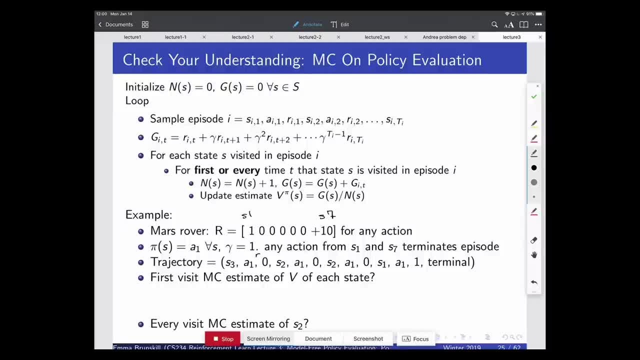 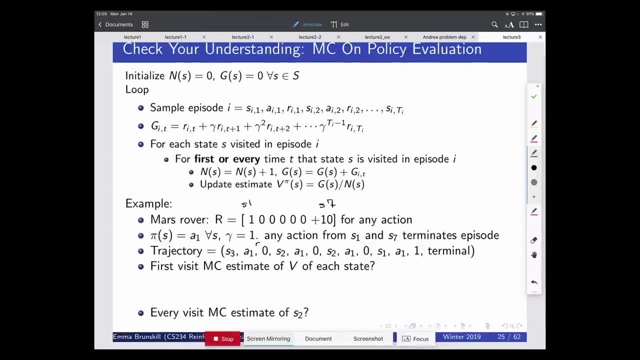 you get a 1, and then it terminates. This is one experience of your Mars Rover's life, Um. so in this case, um, how about we just take a minute or two, feel free to talk to our neighbor and compute what is? 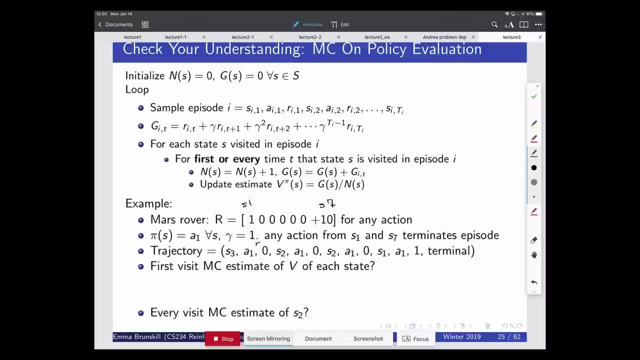 the first visit Monte Carlo estimate of the value of each state and what is the every visit Monte Carlo estimate of state S2?? And I put the algorithm for both um first visit and every visit above. Just depends on whether you update the state only once, for. 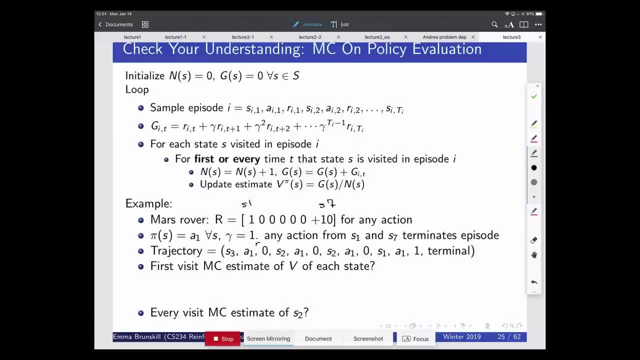 this episode or whether you can potentially update it multiple times. Okay, we'll move on to the question two. if we have not seen it yet, what is the value we use? So the value: you can also say that you initialize V, pay of S equal to 0 for all S. 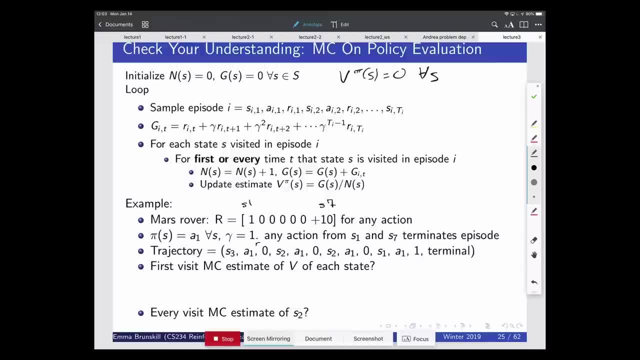 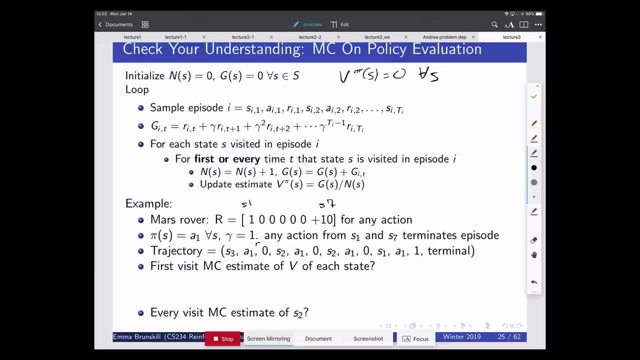 I think the first um, I think the first um, and there's going to be one for every single state, except for the last one, that's 10.. Which states? We've only updated a few of them so far, You would. 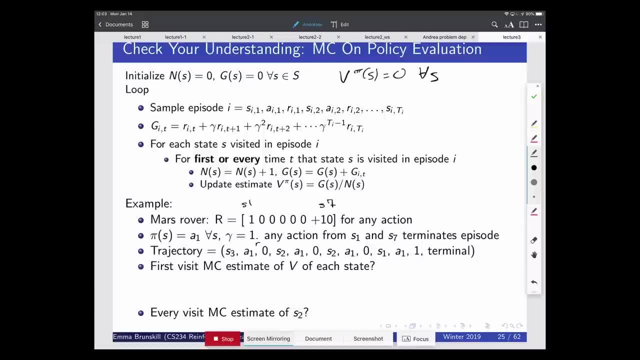 Which? Why don't you give me the full vector? OK, well, let's just start here. So v of s1 is what Is 1.? OK, and v of s2? Is also 1. And v of s3?. 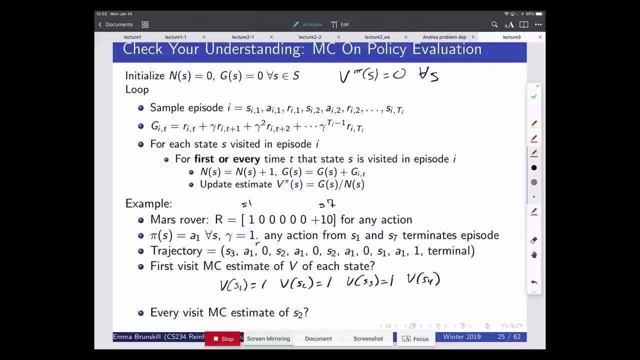 Is also 1. And v of s4? Also 1. That's 0.. You may disagree: 0. 0. 0. 0.. OK, And v of s5? 0. 0. 0.. 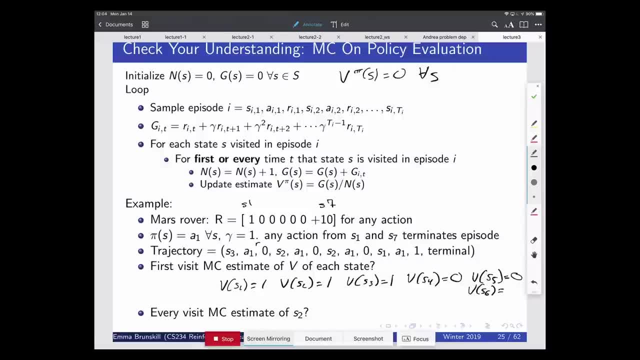 0. 0.. And v of s6? 0. 0. 0. 0. 0. 0. 0.. And v of s7? 0. 0. 0. 0.. 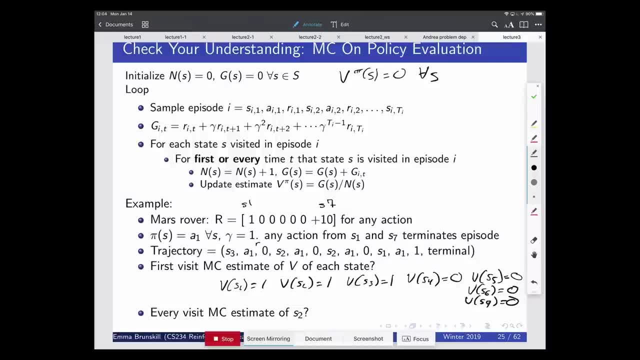 0.. 0. Yeah, so we only get to update in this one the states we've actually visited. So here it's 1, 1, 1, 0, 0, 0, 0.. Now, what about for every visit, the Monte Carlo. 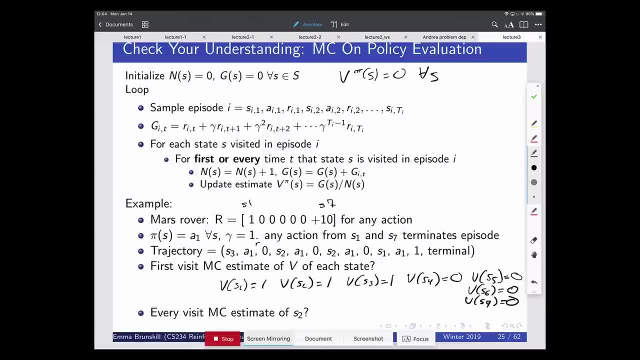 estimate of just s2?? So I picked only s2, because that's the only state we visit twice. What's it- what's its estimate? Well, we increment- yeah, Is it still going to be 1?? Yep, Yes, it is. 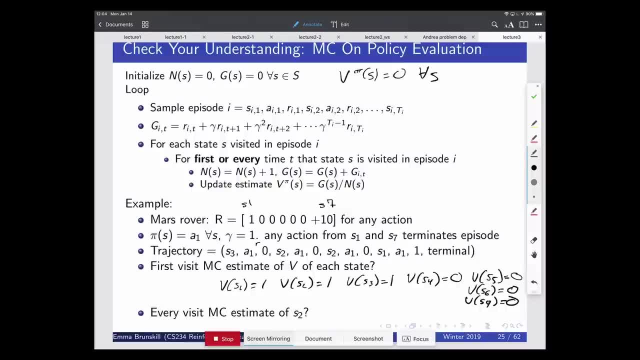 And why Um? because, well, we're both increments- well, so we have: ns is 2 at the end of it, but s- but gs is also 2.. So we incremented both twice, Exactly. So the return from both times when you started in s2 and got. 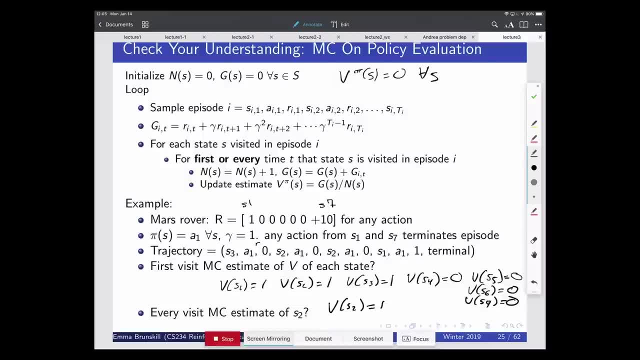 and added up till the end of the episode was 1 in both cases. So it was 1 twice and then you average over that, so it's still 1.. Yeah, Is the reason that they're all 1 because gamma's 1?? 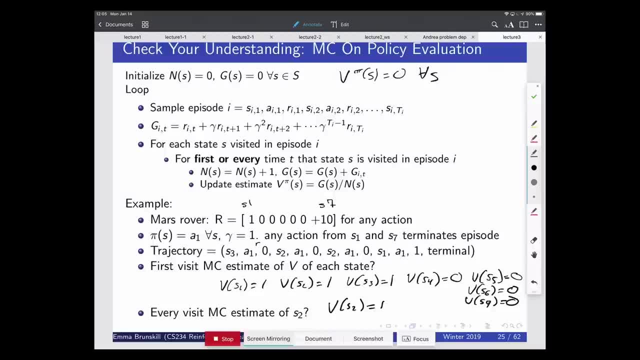 Because, like, shouldn't there be some gamma terms in there? Oh, great question. Yes, Um. so here we've assumed gamma equals 1. Otherwise they would be: um, there'd be a gamma multiplied into some of those two. 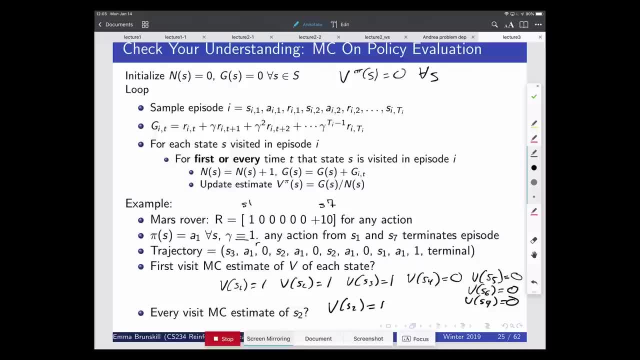 Yeah, No good question. I chose gamma equal to 1 just to make the math a little bit easier. Otherwise it's 1.. Okay, Okay, Great. So you know the-. the second question is a little bit of a red-hanging. 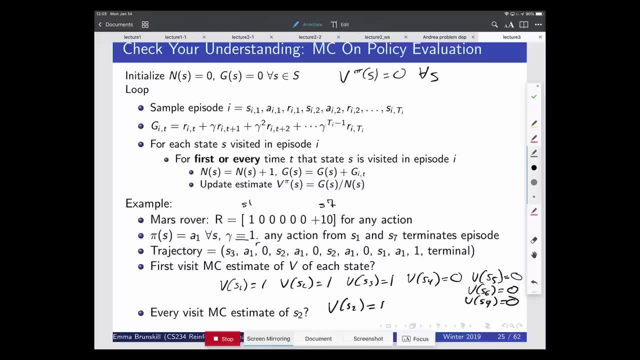 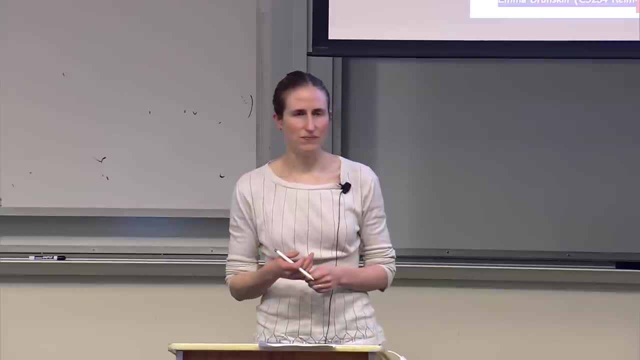 because in this case it's exactly the same. But if the return had been different from s2, um, like, let's say there was a penalty for being in a state- then they could have had different returns and then we would have gotten something different there. 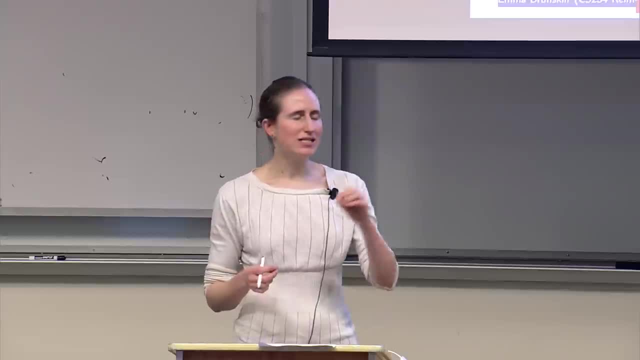 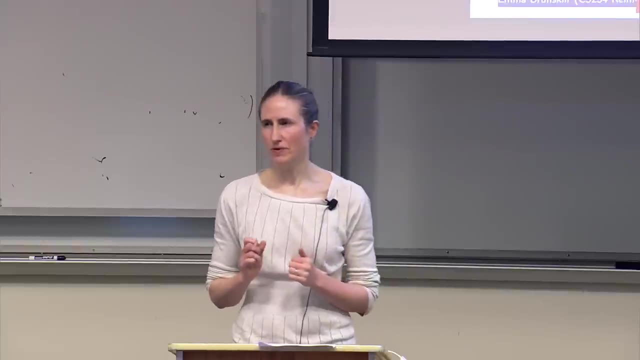 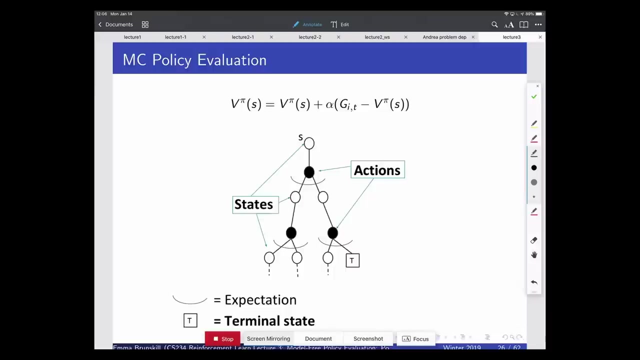 Okay, So Monte Carlo, in this case, updated- we had to wait till the end of the episode, but when we updated till the end of the episode, um, we updated s3,, s2, and s1.. Okay, So what is Monte Carlo doing when we think about how we're averaging over possible futures? 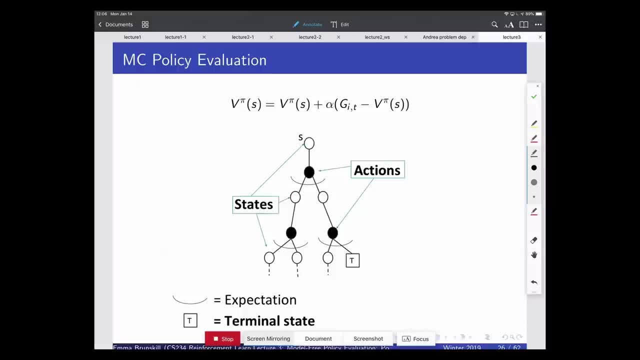 So what Monte Carlo is doing? um, I've put this sort of incremental version here, which you could use for non-stationary cases, but you could think of it in the other way too. Um so- and remember, if you want this just to be equal to every visit- 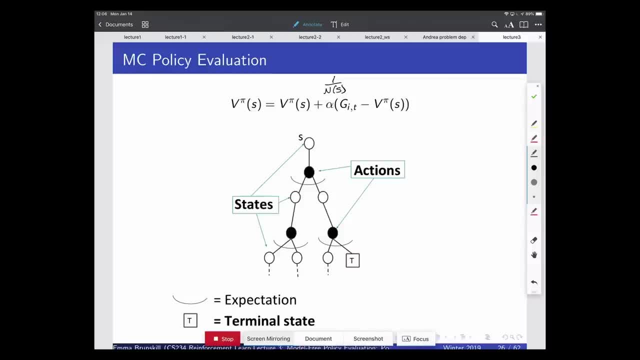 you're just plugging in 1 over n of s here for alpha Um. so this is what Monte Carlo evaluation is doing, is it's just averaging over these returns. So what we're doing is, if we think about sort of what our tree is doing, 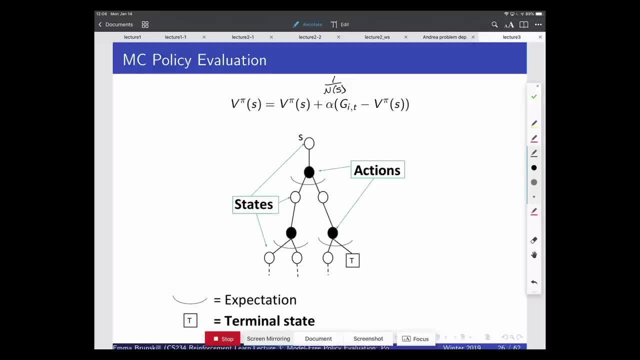 in our case, our tree is gonna be finite. We're gonna assume that each of these sort of um branches eventually terminate. They have to, because we can only evaluate a return once we reach it. So at some point, like here: 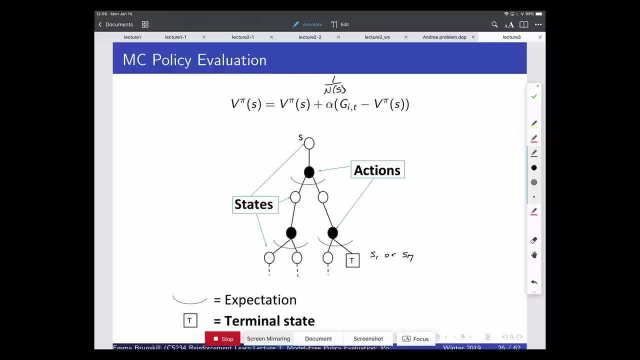 when we got to state s1 or s7 in our Mars example, the process terminated. And so what does Mo- Monte Carlo policy evaluation do? It approximates- It approximates, averaging over all possible futures by summing up one um trajectory through the tree. 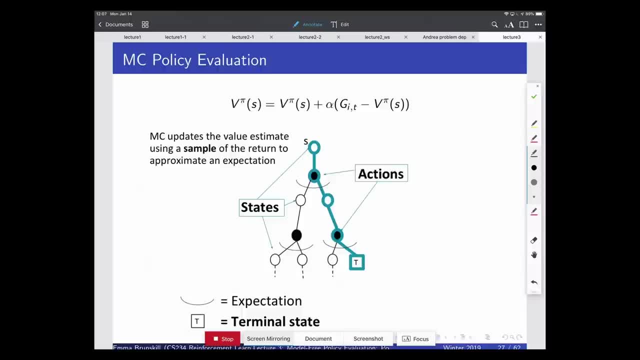 So it samples the return all the way down till it gets to a terminal state. It adds up all of the rewards along the way. So like reward, reward, reward. Well, we'll be more careful than that Reward reward. Here you get a reward for each state action pair. 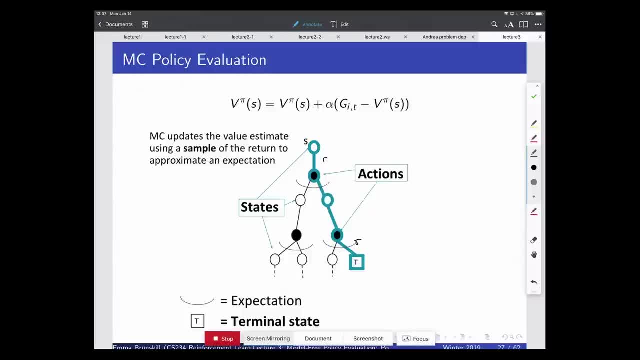 So you sum up all the rewards, in this case um, and that is its sample um of the value. So notice, it's not doing any um- the-. the way it's gonna get into the expectation over states is by averaging across trajectories. 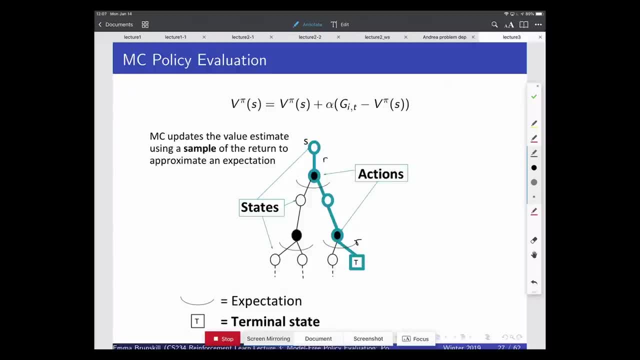 It's not explicitly looking at the probability of next state given S and A, and it's not bootstrapping. It is only able to update when you get all the way out and see the full return. Okay So- so this is- it samples. 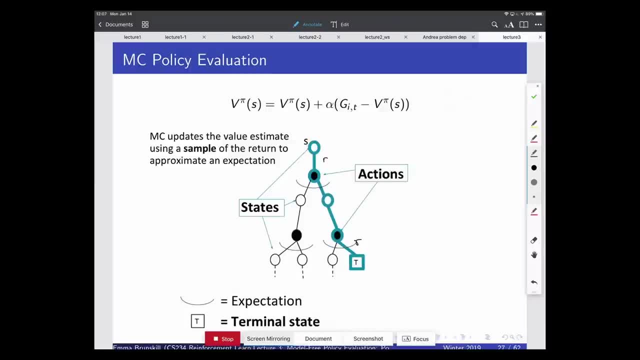 doesn't use an explicit representation of a dynamics model and it does not bootstrap, because there's no notion of VK minus one here. It's only summing up all of the returns Questions. Got it Well, it's interesting. The question is: is it fair to say that this would do? 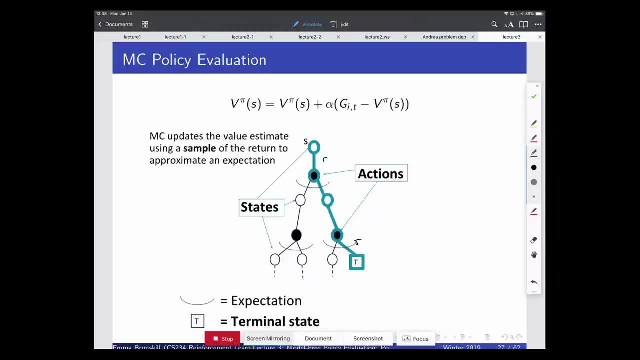 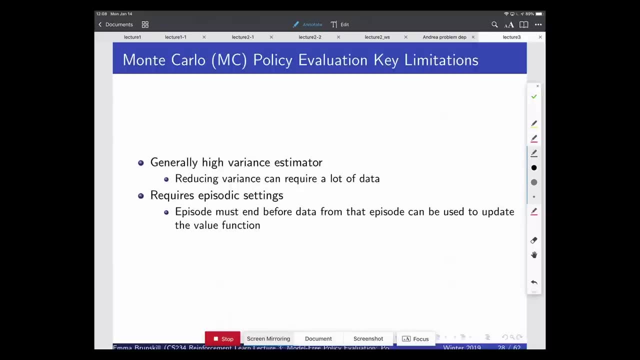 a really bad job in very rare occurrences. It's intriguing: They're very high variance estimators. So if you're- Monte Carlo in general, you're essentially just like rolling out futures right, And often you need a lot of possible futures until you can get a good expectation. 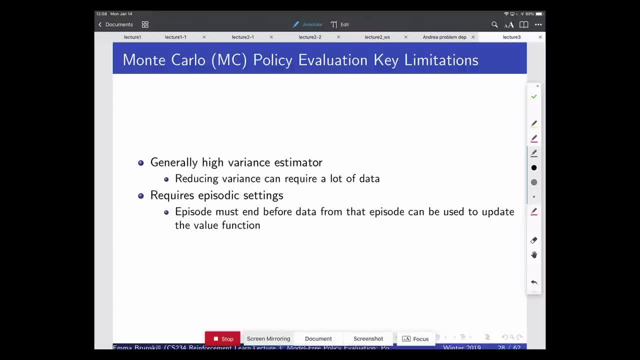 On the other hand, for things like AlphaGo, um, which is, uh, one of the algorithms that was used to solve the board game Go, they use Monte Carlo. So you know, I think, um, you want to be careful in how you're doing some of this rollout, when you start to get into control. 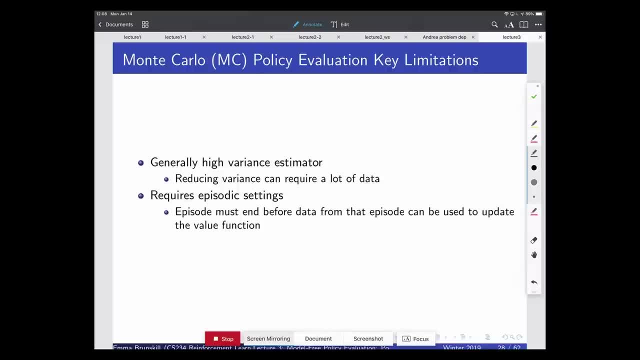 And when you start to- because then you get to pick the actions, um, and you often kind of want to play between, but it's not horrible, even if there's rare events, Um, uh, but if you have other information you can use, it's often good. 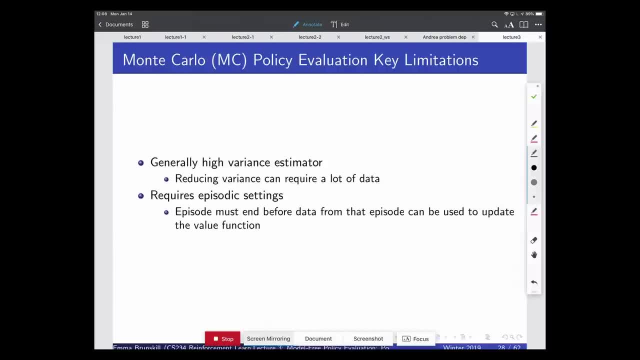 It depends what- what your other options are. So generally, this is a pretty high variance estimate. It can require a lot of data and it requires an episodic setting, Because you can't do this if you're acting forever because there was no way to terminate. 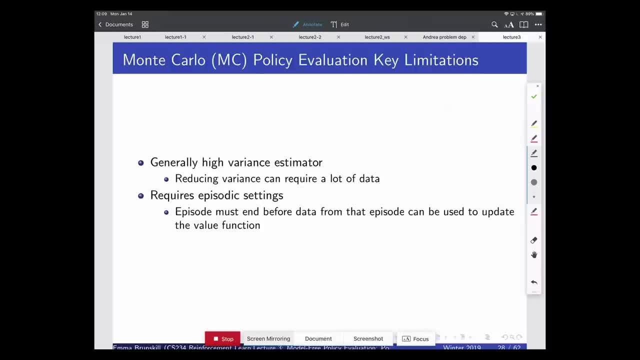 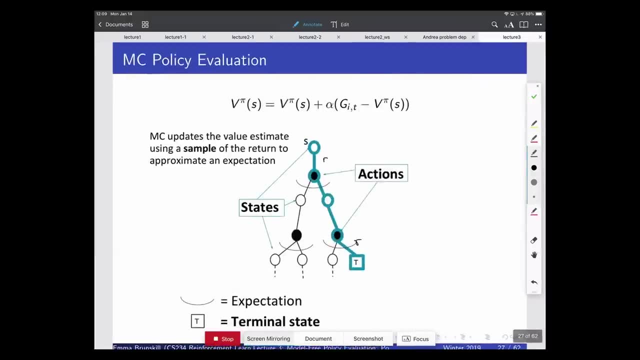 So you have to be able to have processes that terminate. So in the DFP policy evaluation we had the gamma factor because we wanted to take care of the cases where states were looping in between which started like probably equals to one, But in this case I mean. 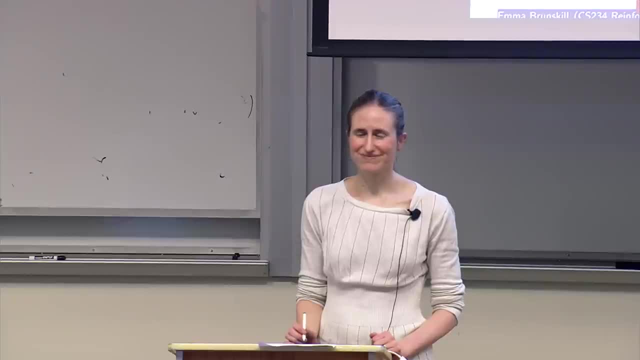 if we had such a case that would never terminate right, Because the episode would never end. So, technically, do we still need a gamma factor to evaluate policy iteration? uh, policy evaluation on? The question was about: do we still need a gamma factor in these cases? 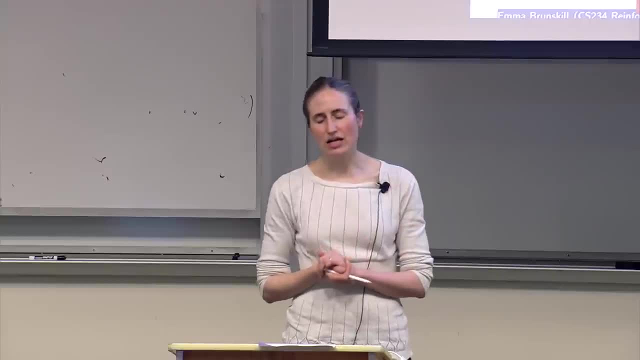 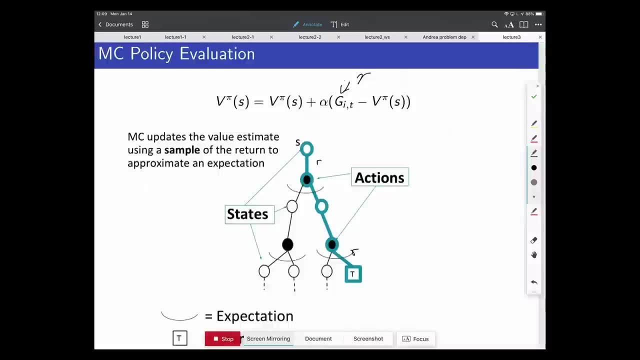 And what about cases where you could have self loops or small loops in your process? So, um, this G in general, can you know, can use a gamma factor, So this can include a gamma. when you compute those, You're right that if the process is known to terminate, 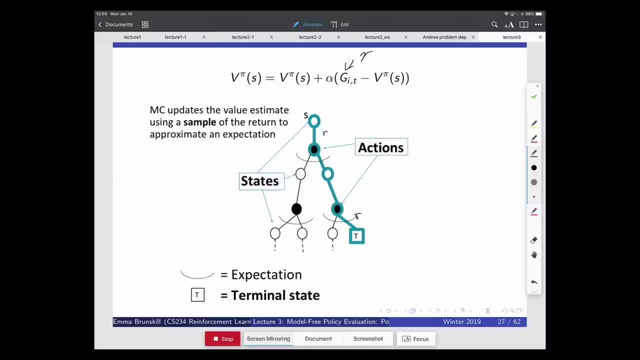 you don't have to have a gamma less than one, Because your reward can't be infinity, because your process will always terminate. Um, this could not handle cases where there's some probability you won't terminate. So if there is a self loop inside of, 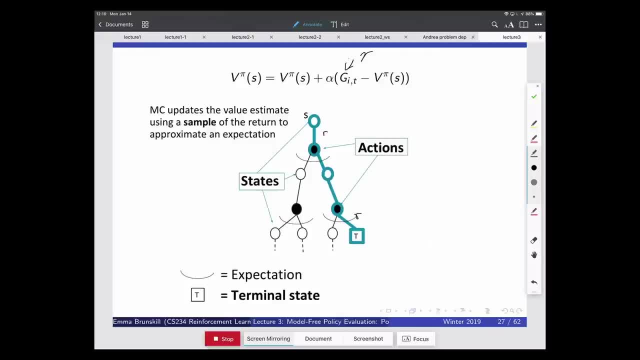 or a small loop inside of your process such that you could go around it forever and never terminate. you can't do Monte Carlo, And having to get this out there won't help. There are physical reasons why you might have a gamma, not just like that right. 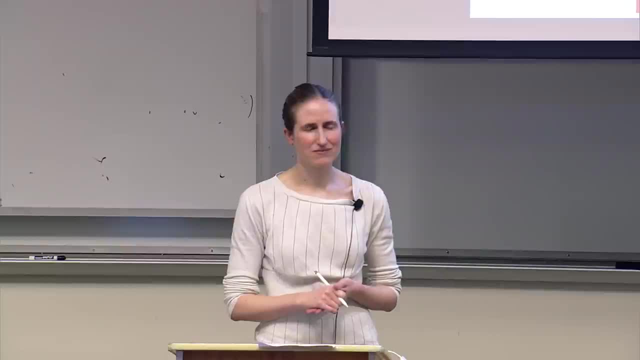 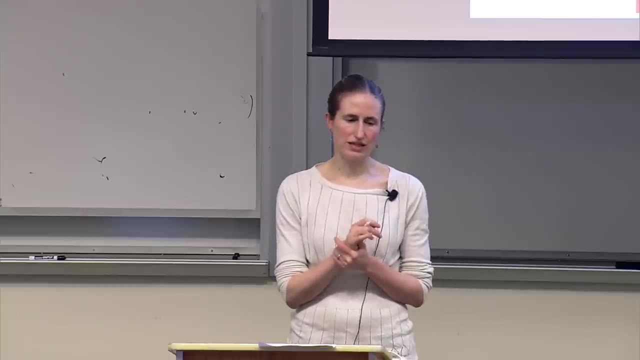 Like, say, modeling fuel costs or something or something moving around. Would that be reasonable? Um, the question is whether or not there might be a physical reason for gamma, um, like fuel costs or things like that. I mean, I think normally I would put that into the reward function. 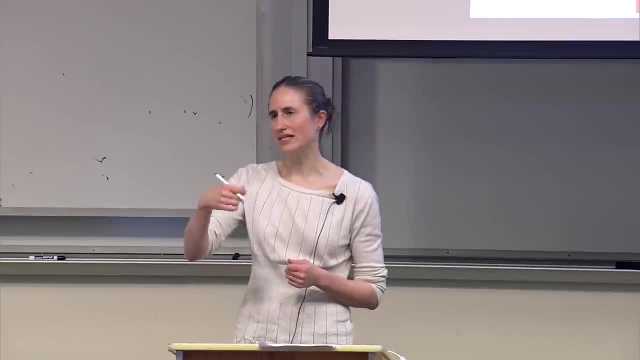 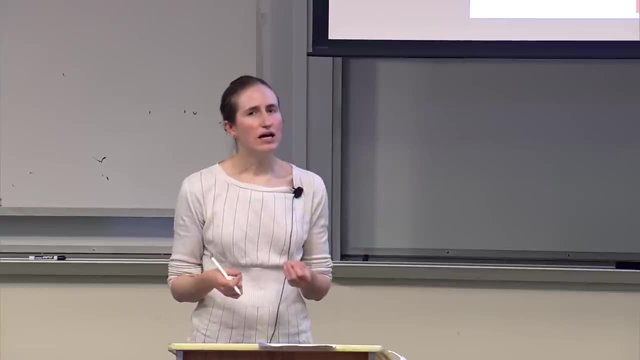 Okay. So if you have something like you- you can have that. So I think, thinking about cases like where, basically, you want to get to a goal as quickly as possible, um, and you want to sort of do a stochastic shortest path type problem. 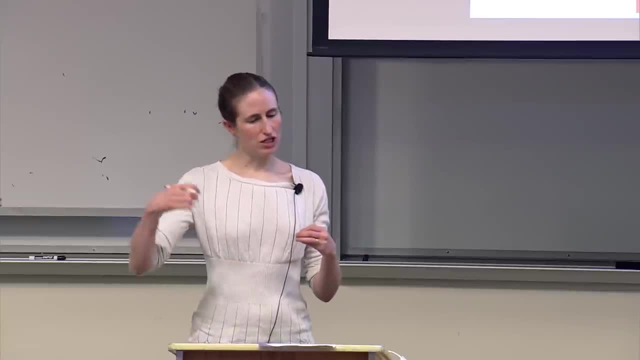 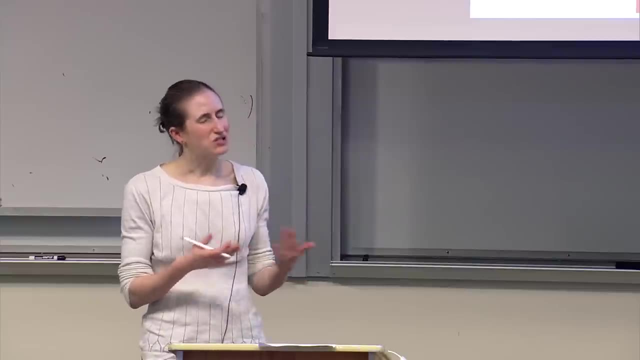 Um, I think generally there I would probably rather pick making it a terminal state and then having like a negative one cost, if you really have a- a notion of how much fuel costs, Um, but you can also use it as a proxy to try to encourage quick progress towards a goal. 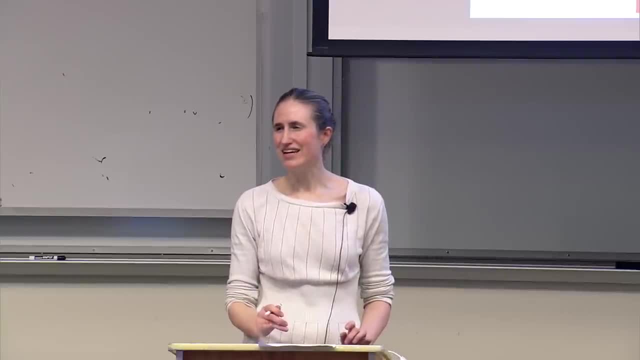 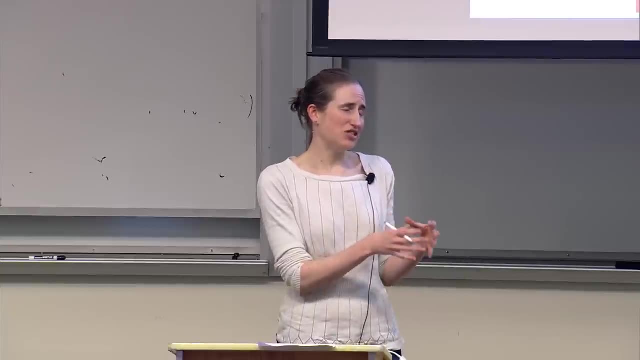 The challenge is that how you set it is often pretty subtle, because, um, if you set it too high, you can get weird behavior where your agent is sort of effectively like too scared to do anything. It'll stay in really safe areas. 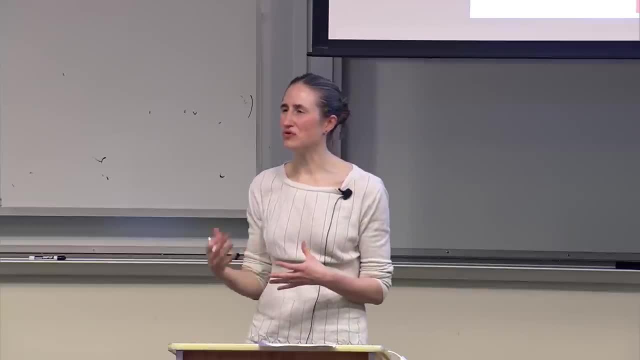 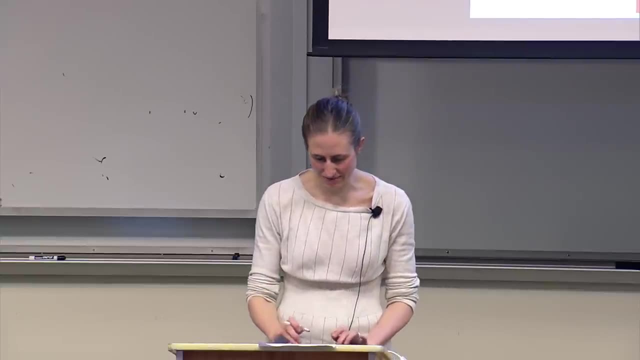 Um, and if it's too high in some cases, if it's possible to get sort of trivial reward, your agent can be misled by that. So it's often a little bit tricky to set in real-world cases. Okay, So there are high variance estimators. 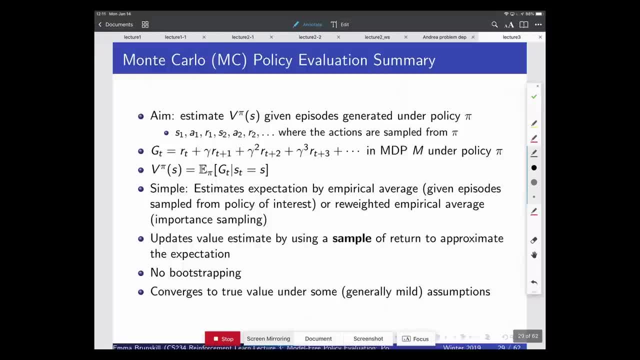 They require these episodic settings Um and um. there's no bootstrapping and generally they converge to the true value under some- uh, generally mild assumptions. We're gonna talk about important sampling at the end of class if we have time. 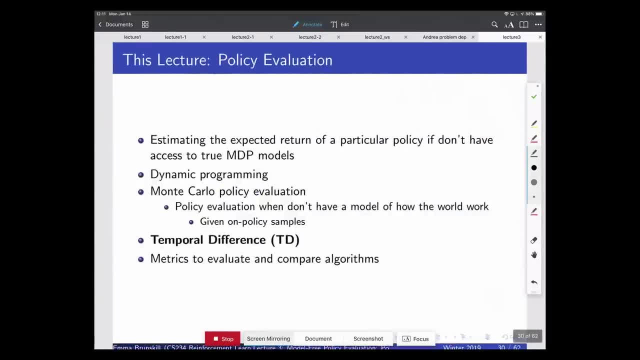 Otherwise, we'll probably end up pushing that towards later. That's for how we do this. if you have off-policy data- data that's collected from another policy- Okay, Now let's talk about temporal difference learning. So if you look at Sutton and Bartow, 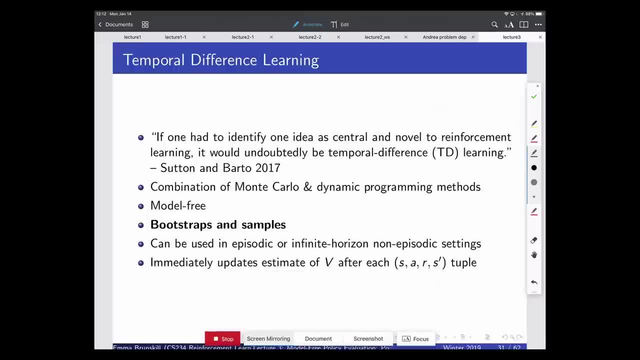 um and if you talk to Rich Sutton or a number of- and a number of other people that are very influential in the field, they would probably argue that the central um contribution to reinforcement learning, or contribution to reinforcement learning- that makes it different, perhaps, than some other ways of thinking about adaptive control. 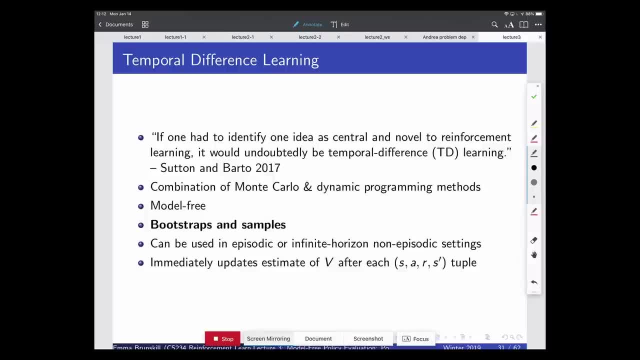 is the notion of temporal difference learning And essentially it's gonna just combine between Monte Carlo estimates and dynamic programming methods and it's model-free: We're not gonna explicitly compute a dynamics model or a reward model or an estimator of that from data. 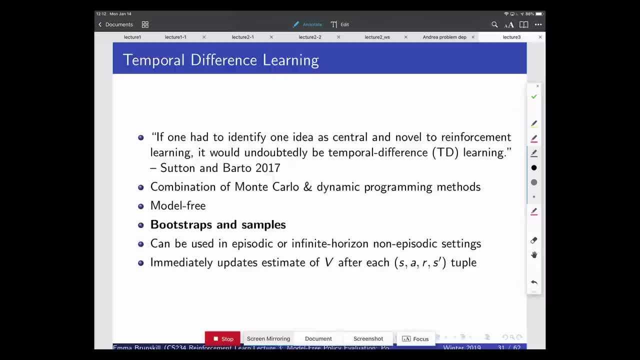 And it both bootstraps and samples. So remember dynamic programming as we've defined it so far. um, it bootstraps And the way we've thought about it so far. you actually have access to the real dynamics model and the real reward model. 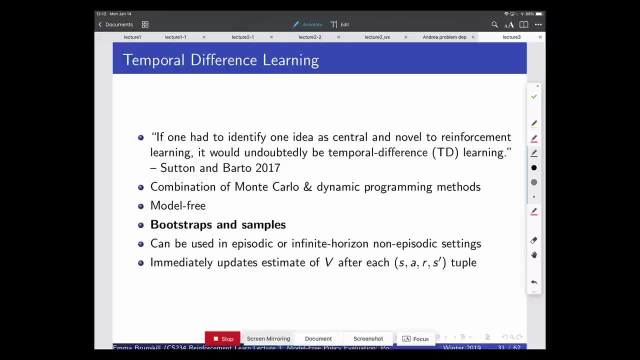 but it bootstraps by using that Vk minus one. Monte Carlo estimators do not bootstrap. They go all the way out to the end of the trajectory and some of the rewards, but they sample to approximate the expectation. So bootstrapping is used to approximate the future discounted sum of rewards. 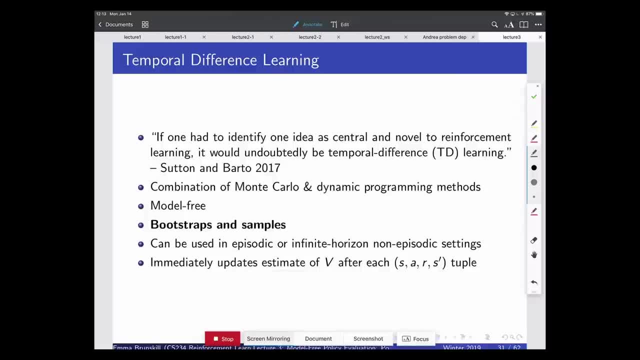 Sampling is often done to approximate your expectation over states. The nice thing about temporal difference learning is you can do it in episodic processes or continual processes, And the other nice aspect about it is that you don't have to wait till the end of the episode to update. 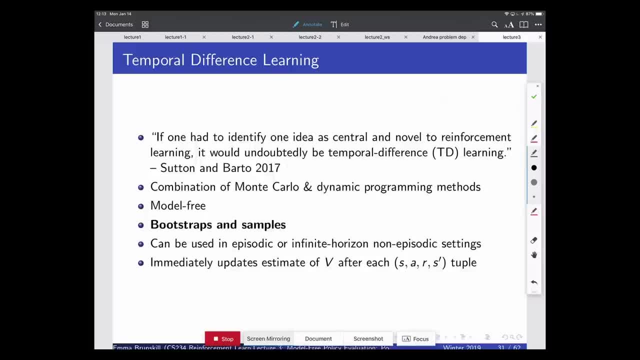 So as soon as you get a new observation, taking a- starting in a state, taking an action and going to a next state and getting some reward- um, you can immediately update your value. And this can be really useful because you can kind of immediately start to use that knowledge. 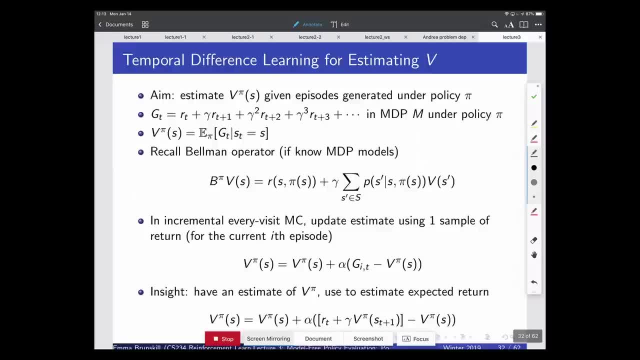 Okay, So how- what are we gonna do in temporal difference learning? Again, our aim is to compute our estimate of V? pi and we still have the same definition of return. Um, and we're gonna look at- remind ourselves of the Bellman operator. 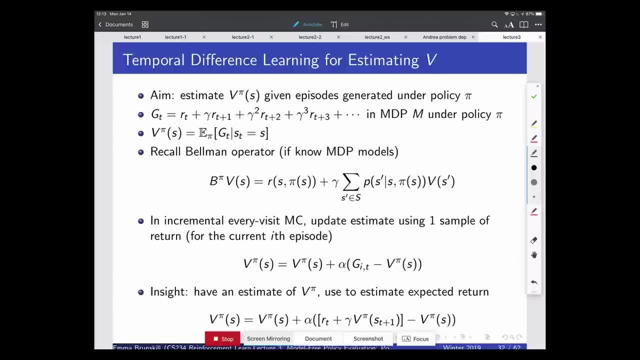 So if we know our MDP models, our Bellman operator said we're gonna get our immediate reward plus our discounted sum of future rewards And an incremental every visit Monte Carlo. what we were doing is we were updating our estimate using one sample of the return. 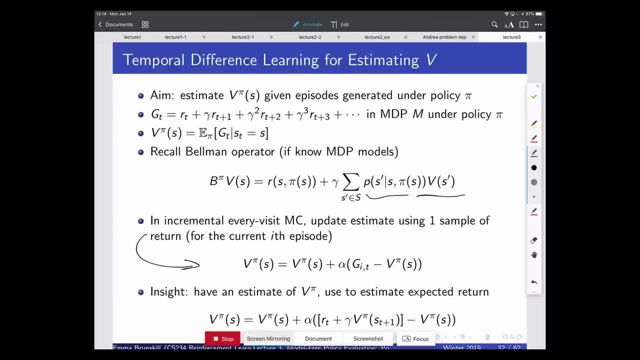 So this is where we said our vet- our new vet estimate of the value is equal to our old estimate plus alpha times the return we just saw minus V. But this is where we had to wait till the end of the episode to do that update. 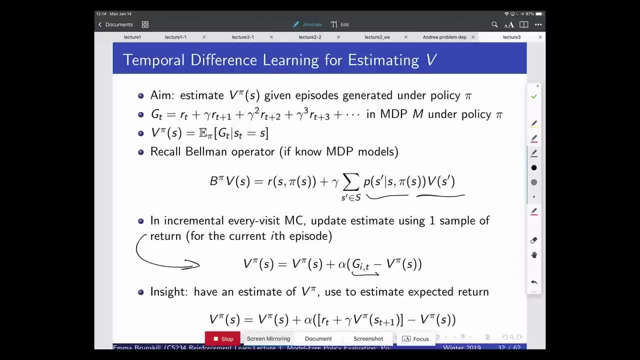 What the inside of temporal difference learning is. well, why don't we just- Use our old estimator of V? pi for that state, and then you don't have to wait till the end of the episode? So instead of using GI there, you use the reward you just saw, plus gamma times the value of your next state. 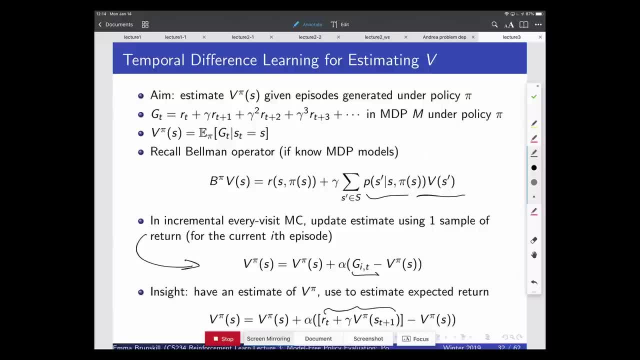 So you bootstrap, Say I'm not gonna wait till I get all the way to the episode start in my state. I got a reward. I went to some next state. what is the value of that next state? I don't know. I'll go look it up in my estimator and I'll plug that in. 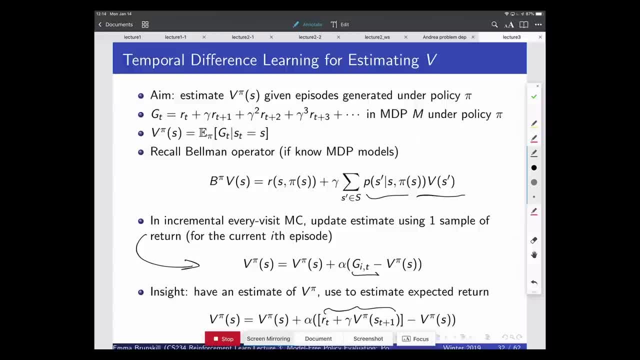 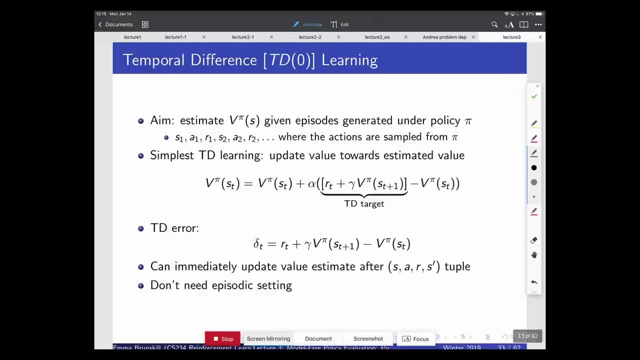 and I'll treat that as a-, as an estimate of the return. So the simplest TD learning algorithm is exactly that where you just take your immediate reward plus your discounted expected future value, where you plug that in for the state that you actually reached. 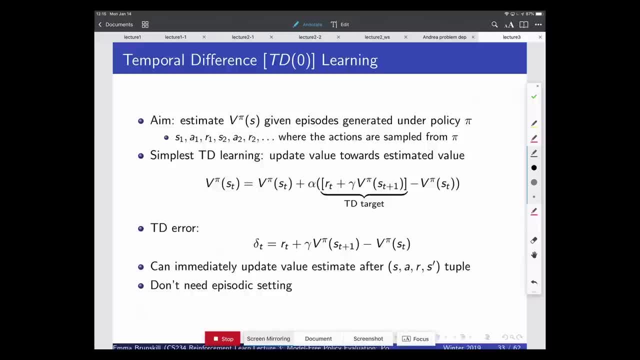 Now notice that this is sampling. There is no- normally we would have like that nice sum In the Bellman operator. we would normally have a sum over S prime. probability of S prime given S A of V pi of S prime. 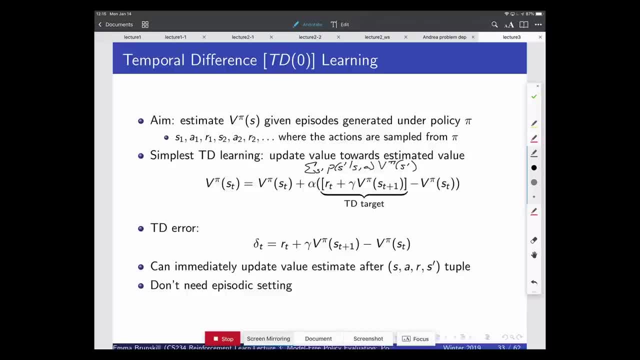 We don't have that here. We're only giving you a single next state and we're plugging that in as our estimator. So we're still gonna be doing sampling to approximate that expectation. But just like dynamic programming, we're gonna bootstrap because we're gonna be using our previous estimate of V pi. 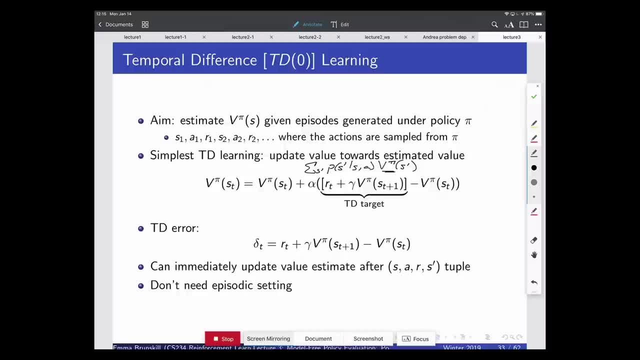 We also write this with like a sub k and sub k minus 1, to show that like the iterations: Yeah, I might have that on there, let me see. No, I don't. in this case, You could also write this with- um. 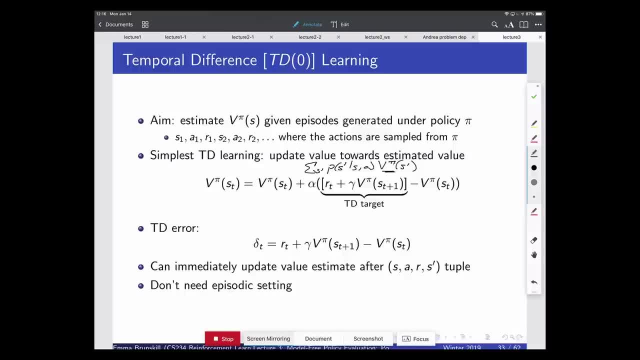 the suggestion is: if we want to just be clear about what is happening in terms of iterations, you can also think of this as V of k plus 1, and this is V of k, for example. You're updating this over time. The thing is is that you're doing this for every single state. 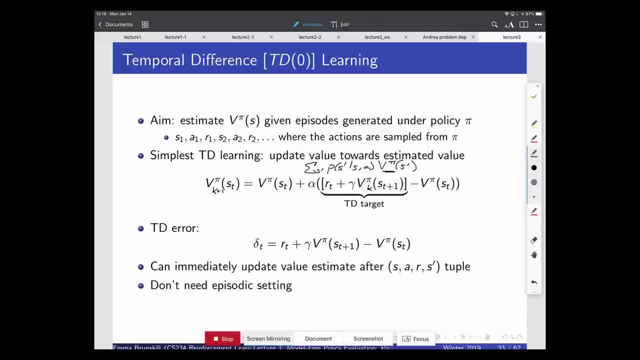 Compared to dynamic programming where you do this in ways where for all states. so you have sort of a consistent Vk and then you're updating Here- we can think of there as just being a value function and you're just sort of updating one entry of that value function, depending on which state you 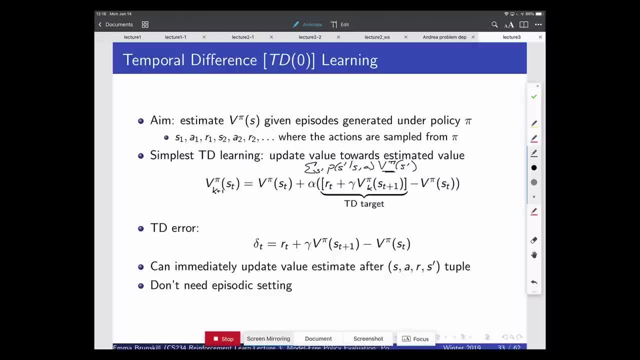 just reached. So there's not kind of this nice notion of the whole previous value function and the new value function. I'll keep it there just for that reason. Now people often talk about the TD error, the temporal difference error. What that is is it's comparing. what is your estimate here? 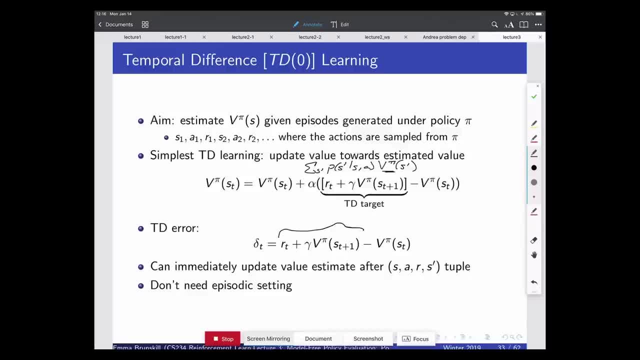 So your new estimate, which is your immediate reward, plus Gamma times your value of the state you actually reached, minus your current estimate of your value. Now notice, this one should have been sort of essentially approximating the expectation over S prime, Because for that one you're going to be averaging. 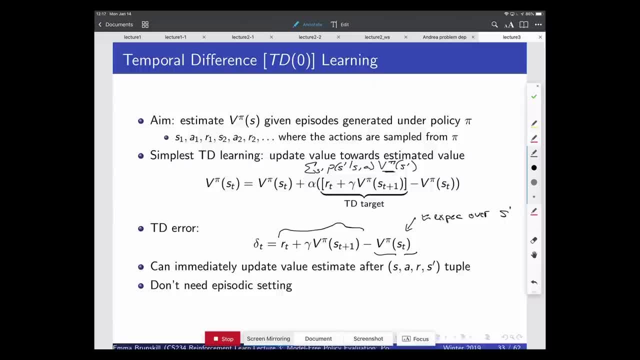 And so this looks at the temporal difference. So this is saying how different is your immediate reward plus Gamma times your value of your next state, versus your sort of current estimate of the value of your current state. Now note that that doesn't have to go to zero. 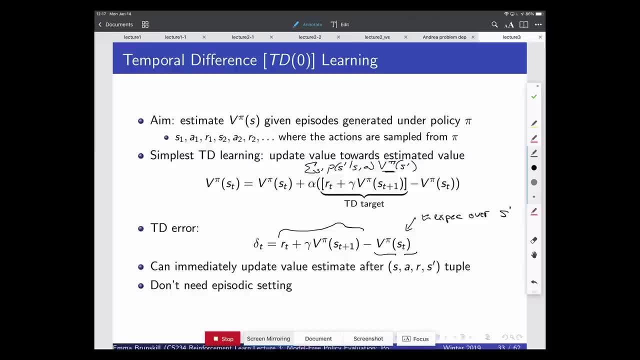 because that first thing is always, ever, just a sample. It's one future. The only time this would be defined to go to zero is if this is deterministic, So there's only one next state. So you know if half the time when I try to drive to the airport, 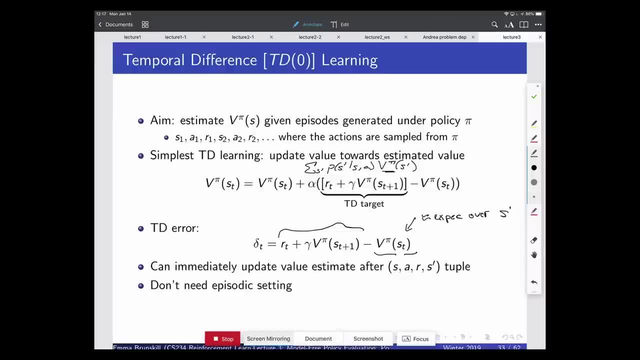 I hit traffic and half the time I don't, then that's sort of two different next states that I could go to from my current start state: either hit traffic or don't hit traffic. And so I'm either going to be getting that b? pi of hitting traffic or b? pi of not hitting traffic. 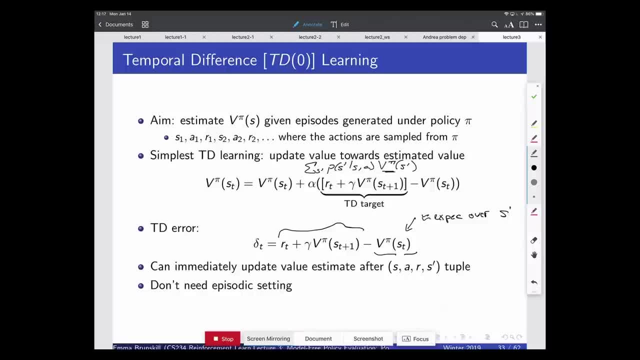 So this TD error will not necessarily go to zero, even with infinite data, because one is an expected thing from the, from the current state, and the other is: which actual next state did you reach? So the nice thing is that you can immediately update this value estimate. 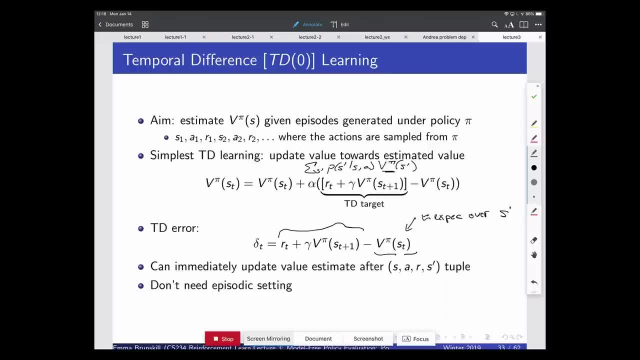 after your state action reward as prime tuple and you don't need episodic settings. Yeah, Scotty, Does this affect convergence if you keep Alpha constant? Yes, Good question: Does this affect convergence if you keep Alpha constant? Yes, And you normally have to have some mild assumptions on decaying Alpha. 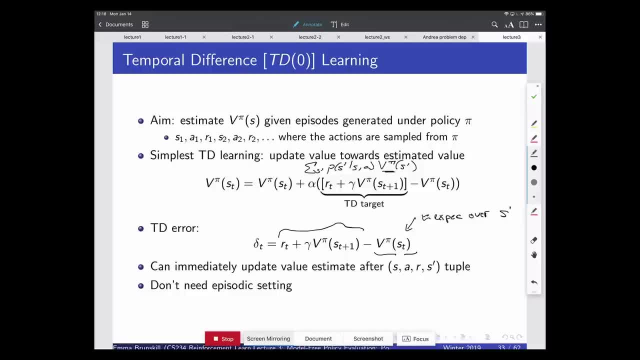 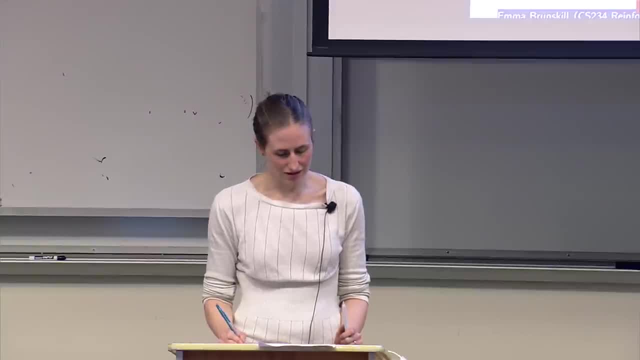 So things like one over T is normally sufficient. 20. To ensure these estimates converge: Yeah, question, Yeah, Um, can you say anything about the bias of this estimator? Yeah, The question was whether- question was a good one. 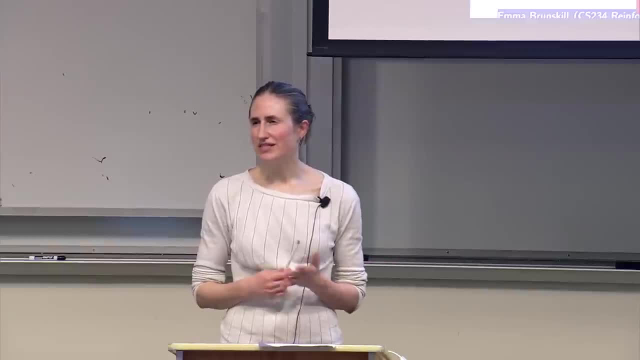 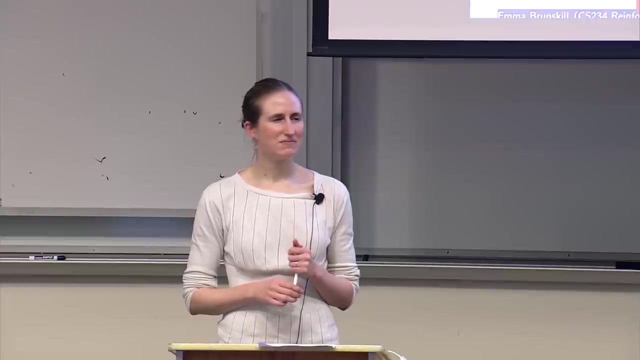 Can you say anything about the bias of this estimator? I may have a sense of whether this is going to be a bias estimator. What if your previous-? sorry, Do you have a sense of whether it's going to be biased? Well, think back to dynamic programming. 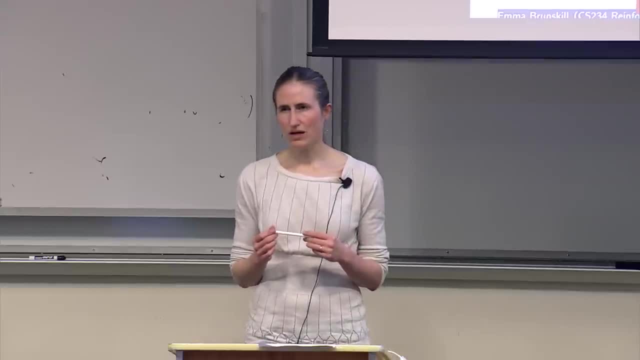 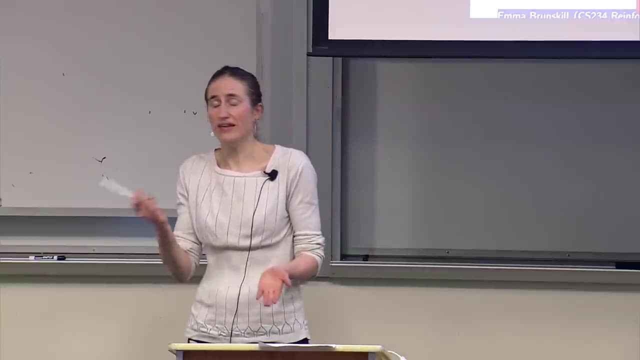 Was vk minus one. um, an unbiased estimator of the infinite horizon, Like, let's say, k is equal to two and you want the infinite horizon value, Is that- no matter how you've done those updates, it's not going to be equal. 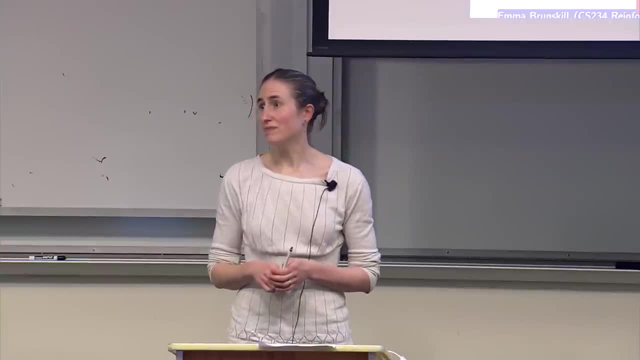 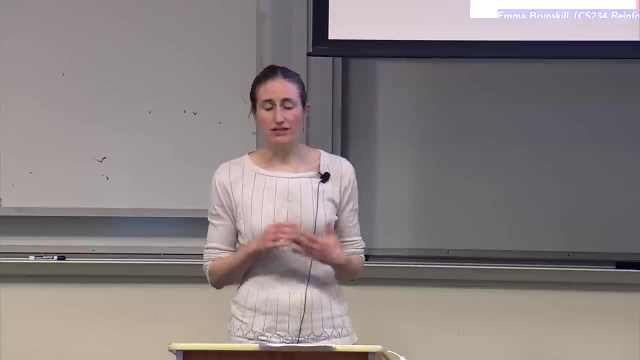 Generally, when you bootstrap, um, it's going to be a bias estimator, because you're relying on your previous estimator, which is generally wrong, And so that's going to be biasing you in one particular direction. So this is definitely a biased estimator. 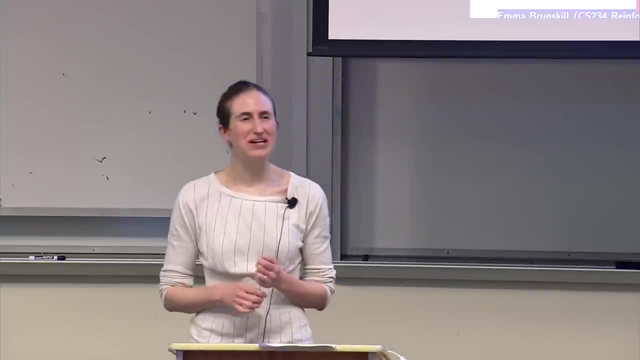 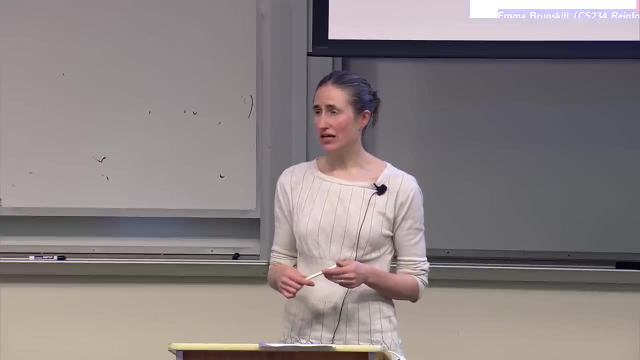 Um, it also can have fairly high variance, So it can both be high variance and be biased, But on the other hand, you can update it really really quickly. Um, you don't have to wait till the end of the episode. 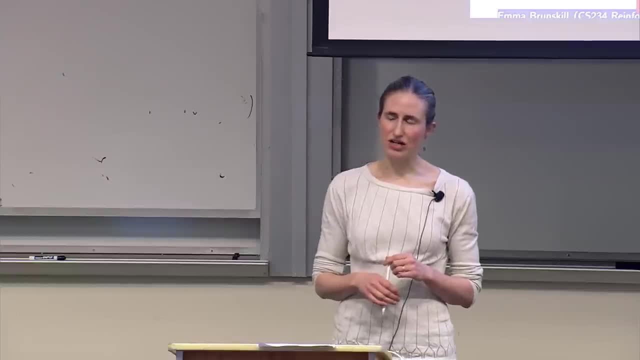 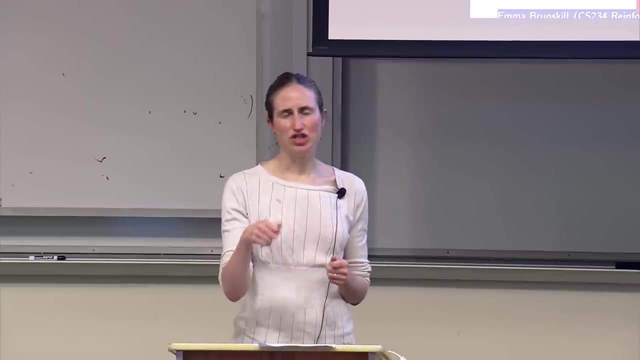 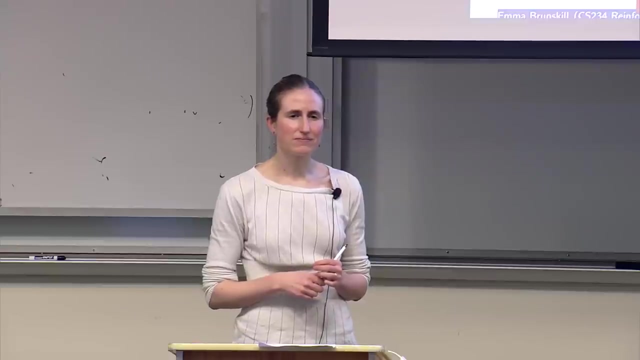 and you can use a lot of information. So it's generally much less high variance than um uh Monte Carlo estimates because you're bootstrapping And that's sort of helping average over a lot of your uh variability. So the random effect is we are initializing the same values. 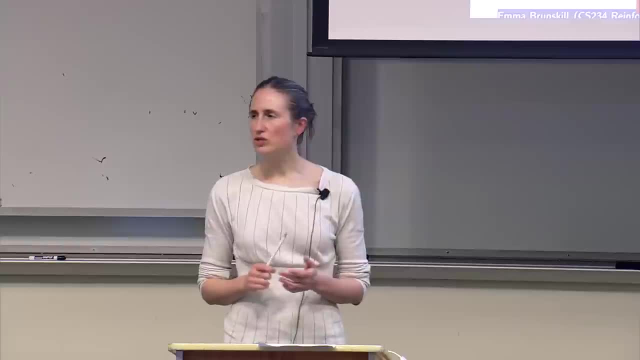 It's a value function- zeroes- which is okay. My question is whether or not it's a function of the initialization. It's not. It's a. it's a function of the different properties of the estimators. You could initialize differently. 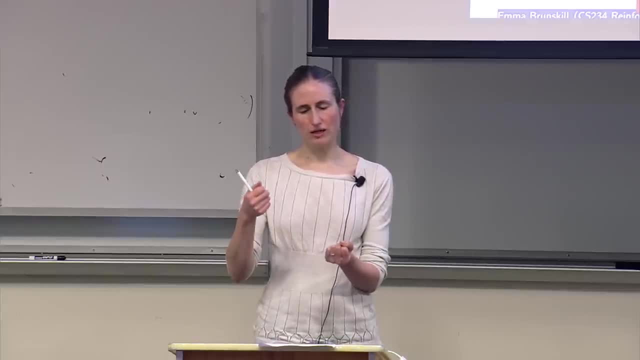 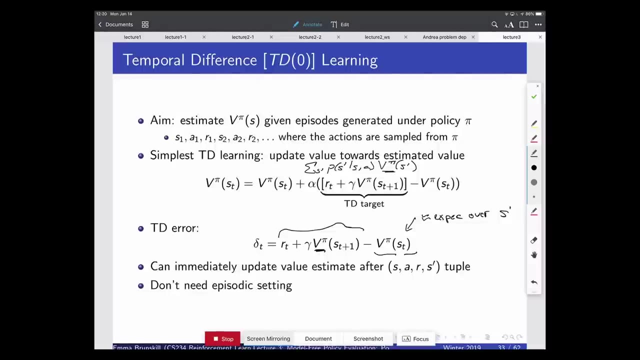 Um, the the bootstrapping is because you're using, uh, by bootstrapping and using this V pi as a proxy for your real expected discounted sum of returns. Um, unless this is the true value, it's just going to bias you. 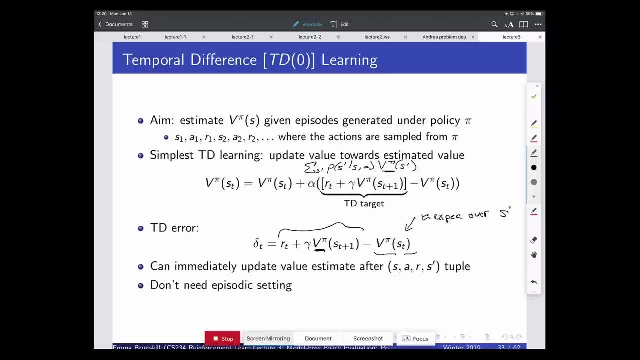 Note that this um, this doesn't- you don't get bias in dynamic programming when you know the models, because that V pi when you bootstrap it's actually V pi, It's actually the real value. So the problem is the here is that it's an approximation of the real value. 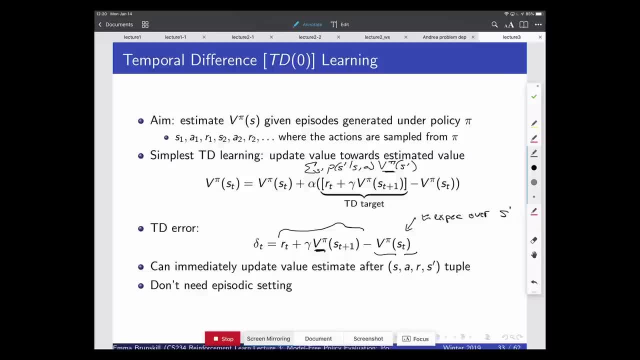 and that's why it's biasing you. So bootstrapping is fine if you know the real dynamics model of the over-, the real reward functions and you've computed V, pi of k minus one, exactly Um. but it's not okay here because we're introducing bias. 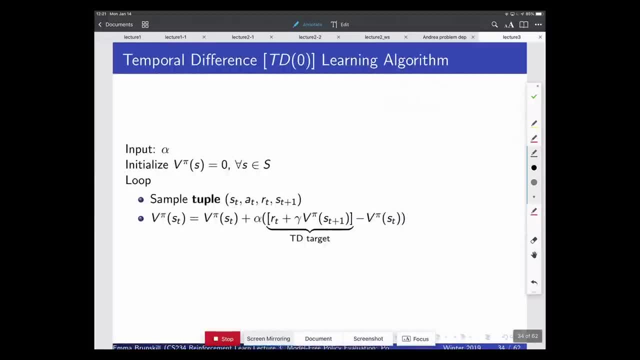 So how does TD zero learning work? Um, I do zero here because there's sort of some interesting um in-betweens between TD learning and Monte Carlo learning, where, instead of doing an immediate reward plus the discounted sum of future rewards versus summing all of the rewards. 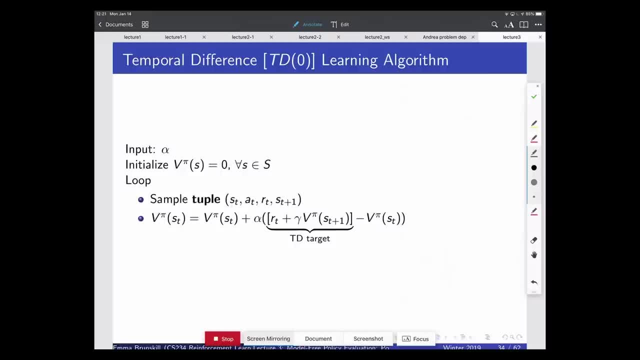 you can imagine continuums between these two, where you maybe sum up the first two rewards and then bootstrap. So there's um, there's a continuum of models based- a continuum of algorithms between um, just taking your immediate reward and then bootstrapping versus never bootstrapping. 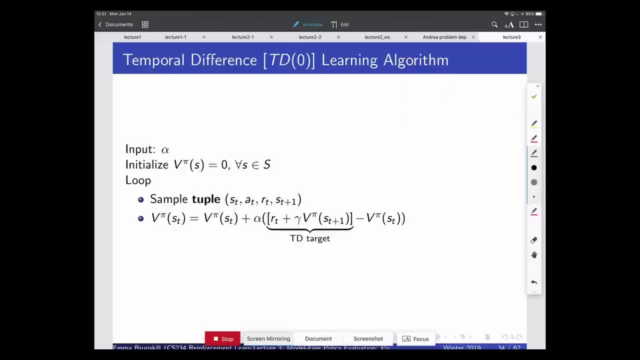 Um, but we're just gonna talk right now about taking your immediate reward and then bootstrapping. So TD learning works as follows: You have to pick a particular alpha um which can be a function of the time step Um. you initialize your value function. 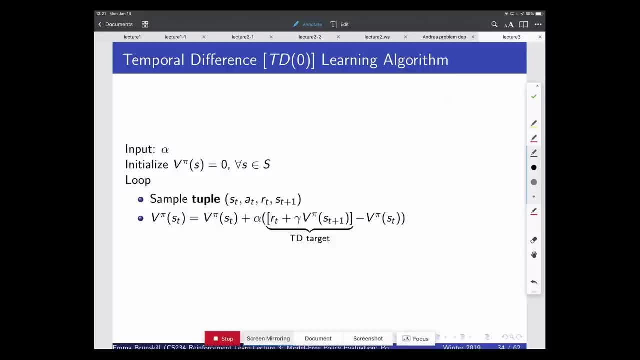 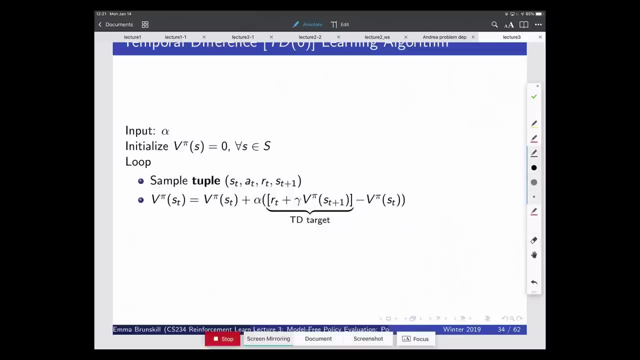 you sample a state action, reward next state. Now, in this case, because we're doing policy evaluation- oh sorry, let me- this will be equal to pi of st, And then you update your value. Okay, So let's look um. 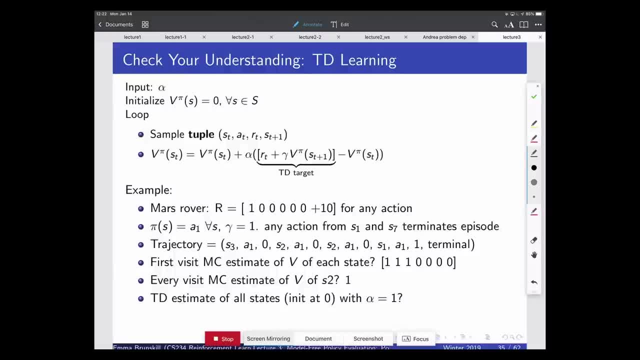 again at that example we had before. So we said that for first visit Monte Carlo you would get 1, 1, 1, 0, 0, 0, 0.. The every visit would be 1.. What is the TD estimate of all states at the end of this episode? 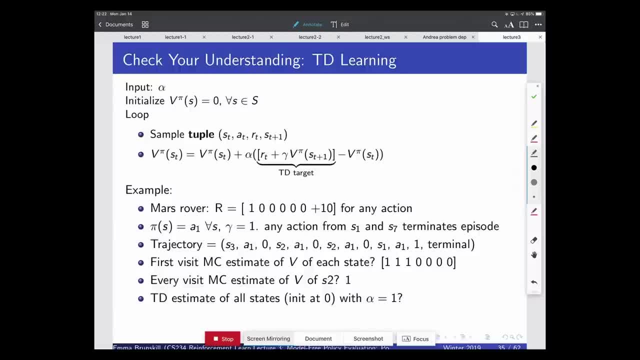 So notice what we're doing here. We loop, We sample a tuple, We update the value of the state we just reached. We get another tuple, We sample it. So what would that look like? in this case? We would start off and we'd have S3.. 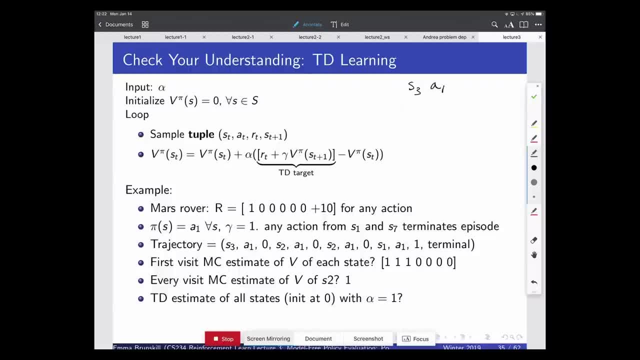 We'd have S3, A1, 0, S2.. We'd have S2, A1, 0, S2.. S2, A1, 0, S1.. S1, A1, plus 1, terminate. 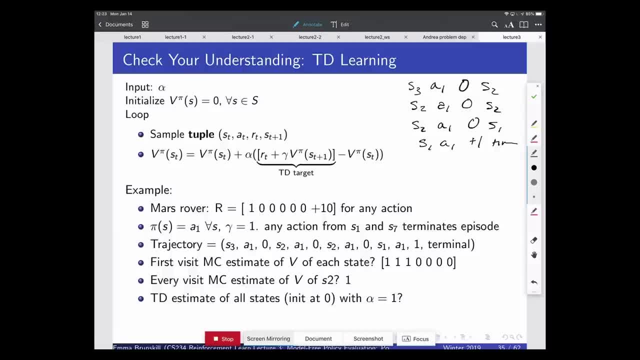 So why don't we just wait a minute and think about what the value would be under TD learning And what implications this might have too? Okay, Does anybody want to say what the value is? that you get Yeah, Uh, 1, followed by all zeros. 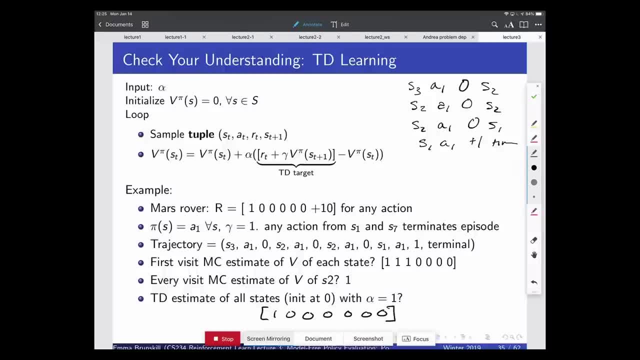 That's right, Okay. 1 followed by all zeros: Okay, So we only updated the final state in this case. I also just wanted to- yeah, question, Um, verify why that happens? Yeah, Because, um, what we are doing in this case is that we get a data point. 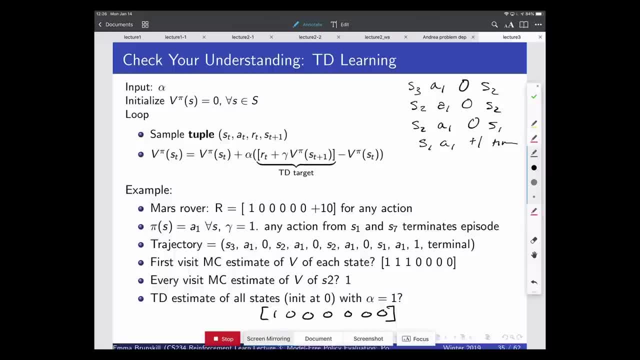 So we're in a state, we take an action, we get our word. we get next state, We update the value only for that state. So what we did here is we got S3. We updated, we did action. A1,. 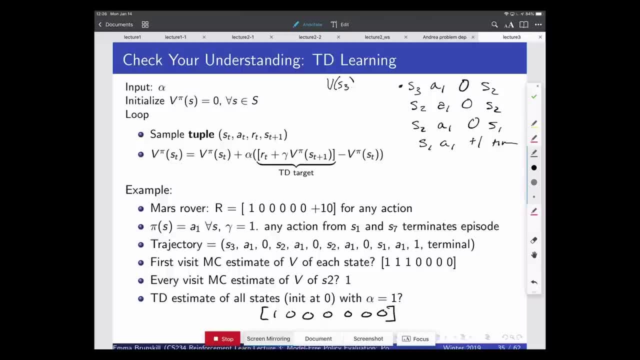 we got a 0, S2.. So our new value for S3 was also equal to 0.. Okay, So what we did here is: we got S3, we updated, we did action A1, we got a 0, S2.. So our new value for S3 was also equal to 0.. So our new value for S3 was also equal to 0.. 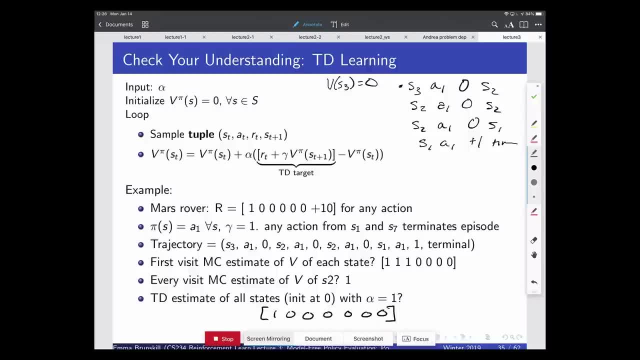 So we went to S2, we took action A1, we got a 0,. we went to S2, we got- so we updated S2, it was also 0.. We did that again and we finally got to state S1, and we got a 1.. 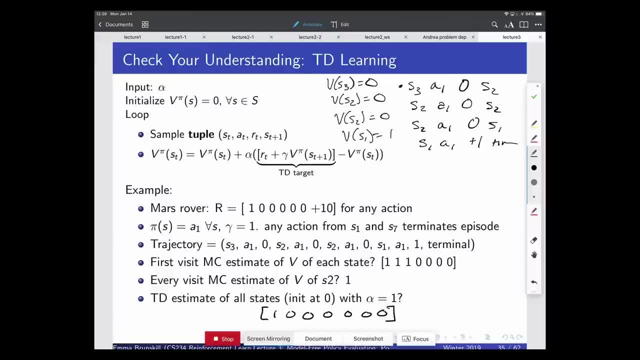 So the thing about this that can be beneficial or- or not beneficial is you throw away your data. in the most naive form, You have a S A R S prime tuple and then it goes away again. You don't keep it. 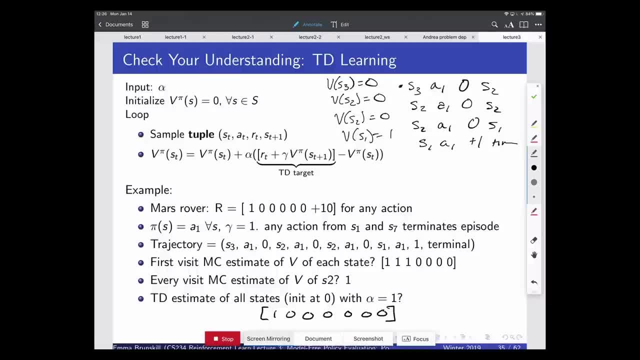 And so when you finally see that reward, you don't back up, you don't propagate that information backwards. So what Monte Carlo did is it waited till you got all the way there and then it computed the return for every state along the episode. 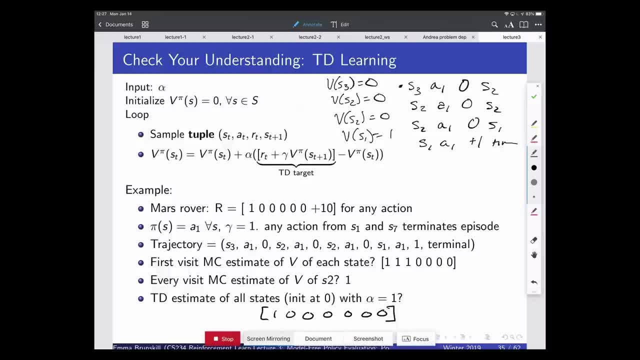 which meant that that's why we got 1, 1,, 1, 1.. But here you don't do that. By the time you get to um S1, you've thrown away the fact that you were ever in S3 or S2,. 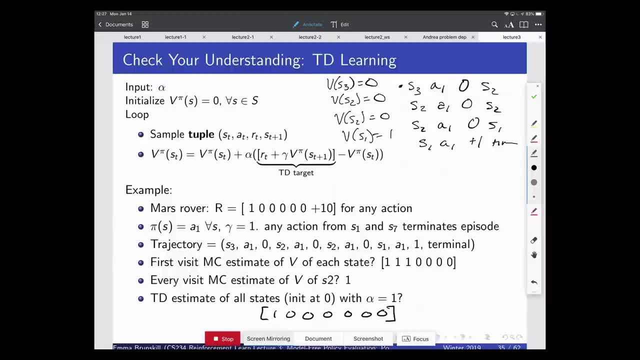 and then you- you don't update those states Time until a reward is proportional to the number of samples. you need to get a good estimate of value function. Say that again. Uh, I'm assuming that like the long-term value function. 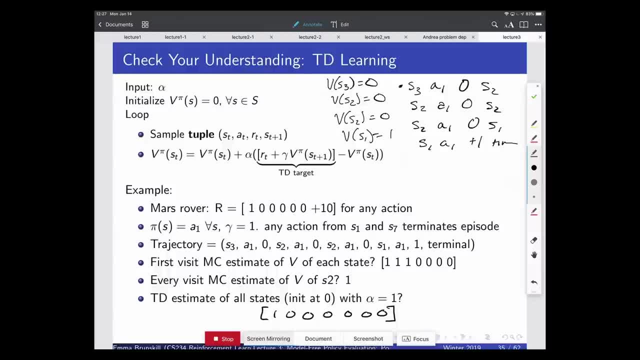 the longer it takes for you to get a reward, the more samples you need to like properly estimate uh value function. Question I'm not totally sure is sort of: you know, how long does it take you to get a reward? 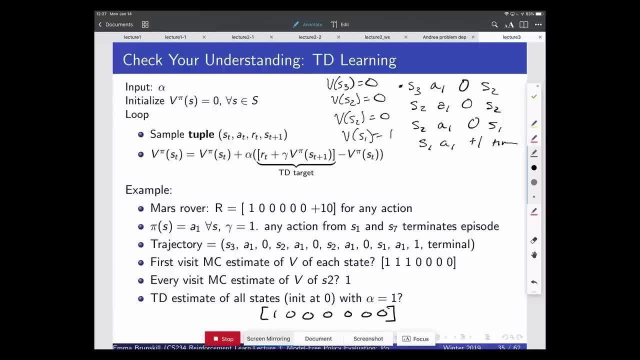 and how many samples do you need to get an estimate of the value function? Um, you mean for all states. It's a little nuanced. Um, it depends on the transition dynamics as well. Um, you can say for a particular like how- how many um samples you need. 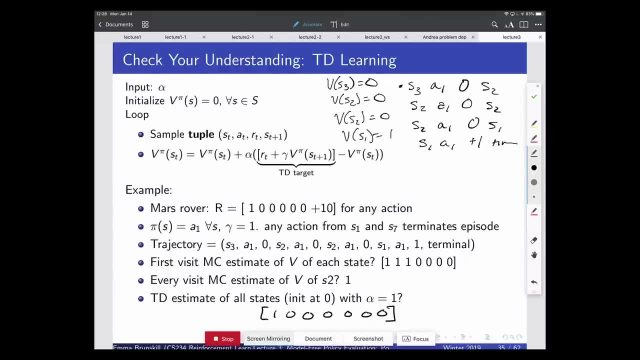 for a particular state to get a good estimate of its reward. Let's say, your rewards are stochastic, But in terms of how long it takes you to propagate this information back, it depends on the dynamics. Um, so in this case, you know. 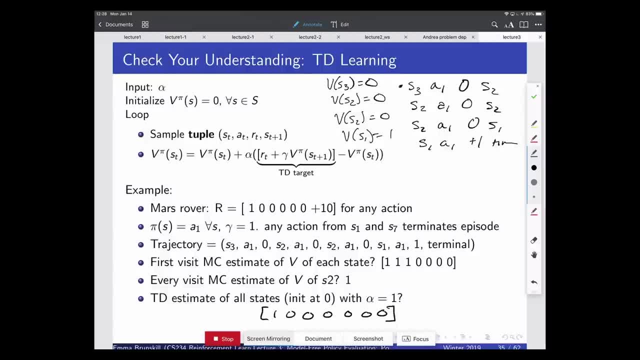 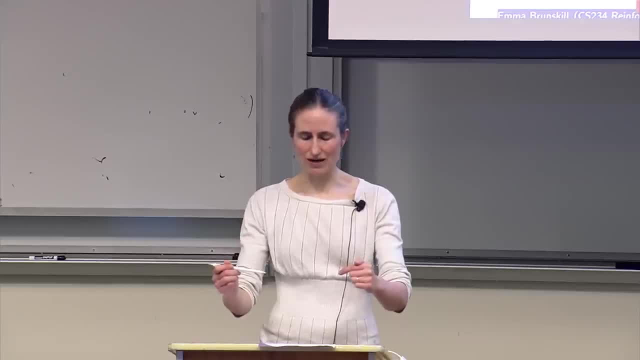 if you had exactly the same trajectory and you did it again, then you would end up updating that S2.. And then, if you got that same trajectory again, then you would propagate that information back again to S2, and then one more time. then you get it back to S3.. 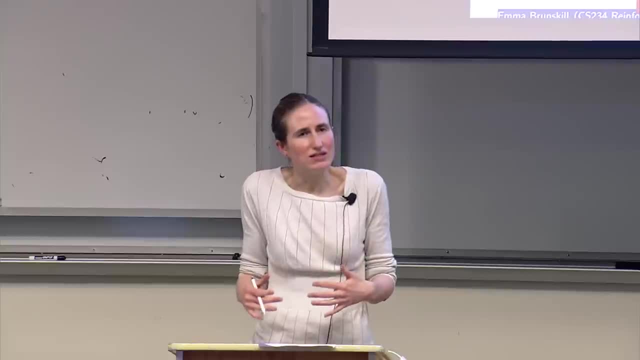 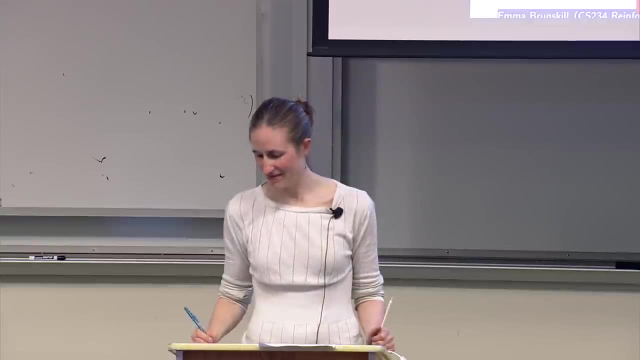 Actually for S3, and that's the third one. So you can slowly just propagate this information back Um, but you don't get to kind of immediately like what Monte Carlo would do. Question: I was wondering if you could highlight the differences between this and. 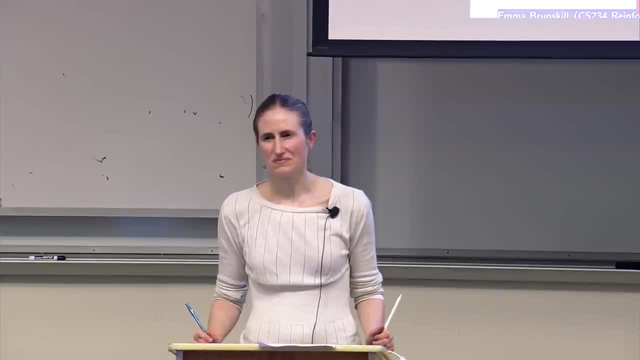 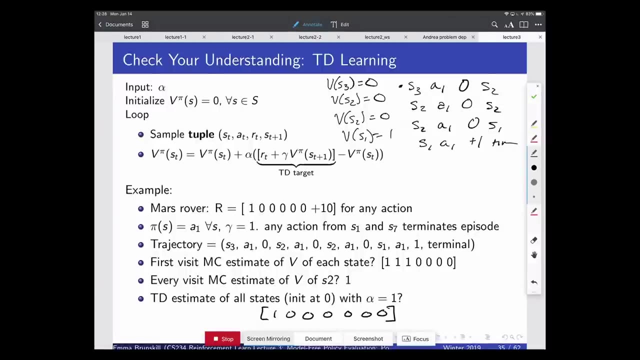 the Q-learning that we talked about last time, because they seem like kind of similar ideas. That's great, So exactly right. In fact, TD-learning and Q-learning are really close analogs. Q-learning is um when you're gonna do control. 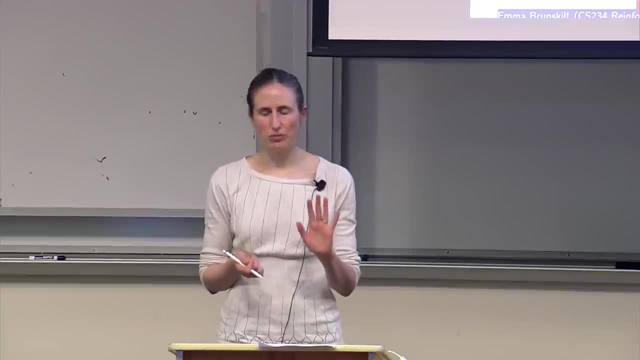 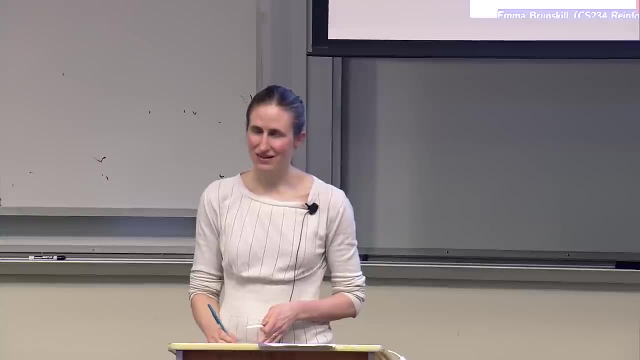 So when we're gonna look at actions, TD-learning is basically Q-learning, where you're fixing the policy. Yeah, question back there. So if you're gonna actually like implement this- though you would- you would keep looping right. 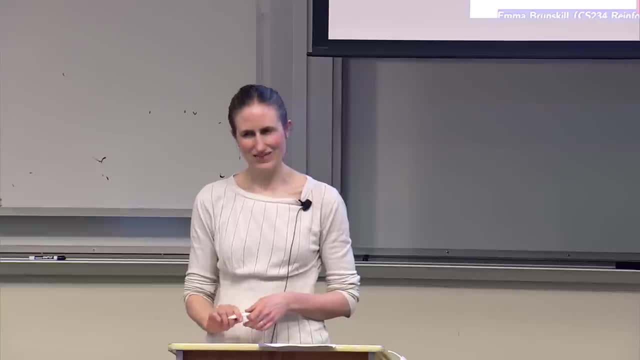 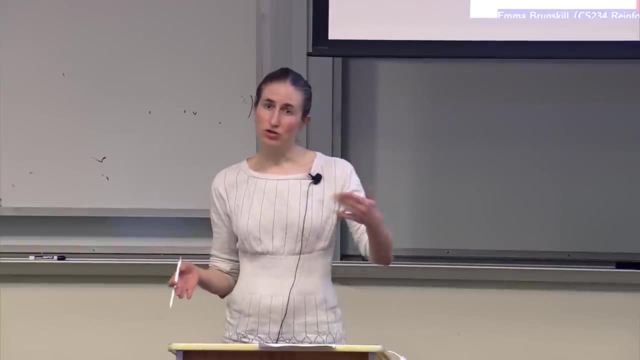 and- and updating, or you would just run through uh once. It depends. So, um, uh, it depends who you ask to. So if you're really really comp- concerned about memory, um, you just drop data. 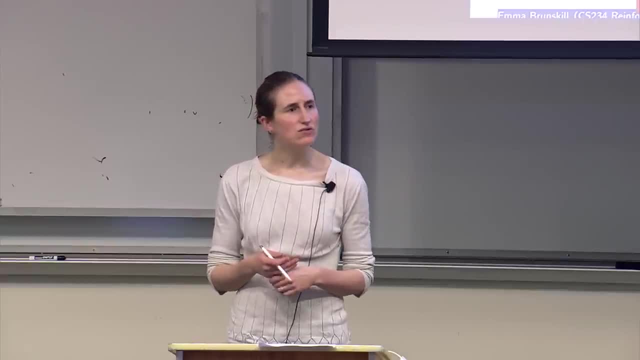 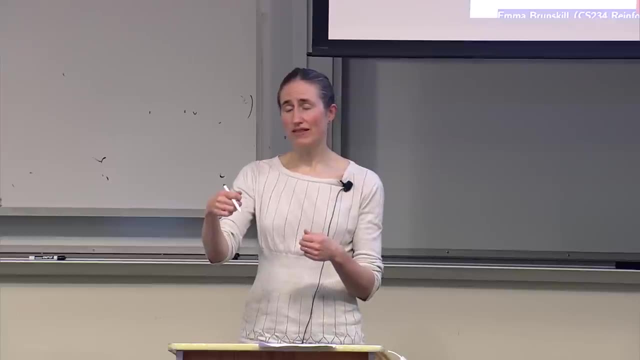 So then you only have this: If, um, in a lot of the existing sort of deep learning methods, you maintain a sort of a a-, a episodic replay buffer, and then you would resample samples from that and then you would do this update for the samples from there. 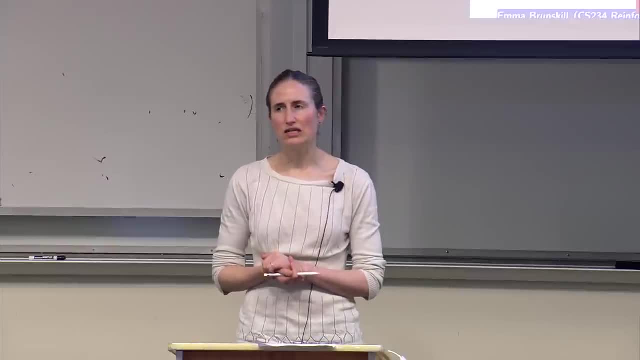 So you could revisit sort of past stuff and use it to update your value function. Um, you could also- it could- it can matter the order in which you do that. So in this case, you could do a pass through your data. 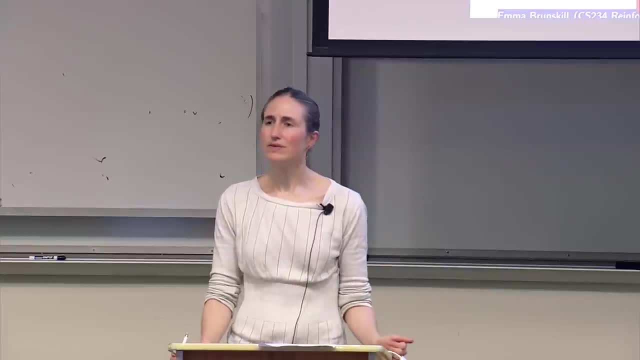 and then do it another pass, or maybe go backwards from the end, If you, if you like, do another pass through, right, then you would end up, you know, propagating some alpha back to S2,, right, Yeah? 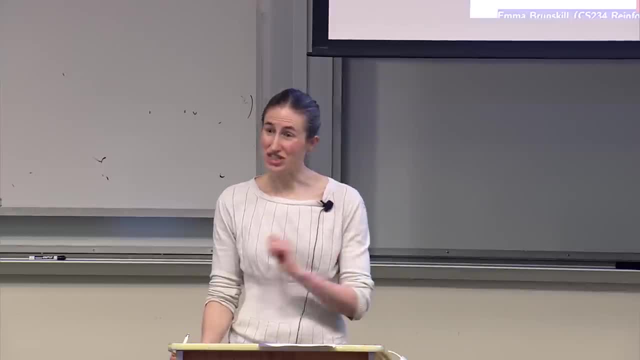 So you just go into like convergence or We'll talk about that very shortly? Yes, There's a great question of like. so what happens if you do this to convergence- And we'll talk about that in a second. 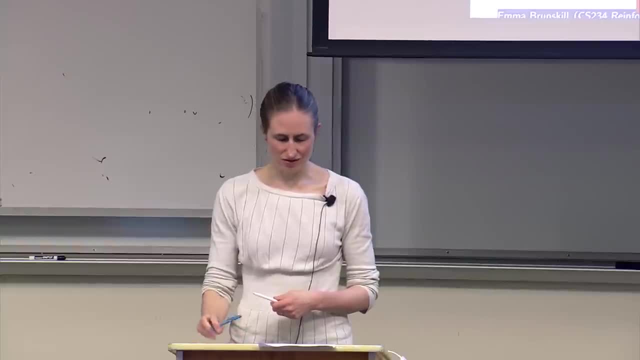 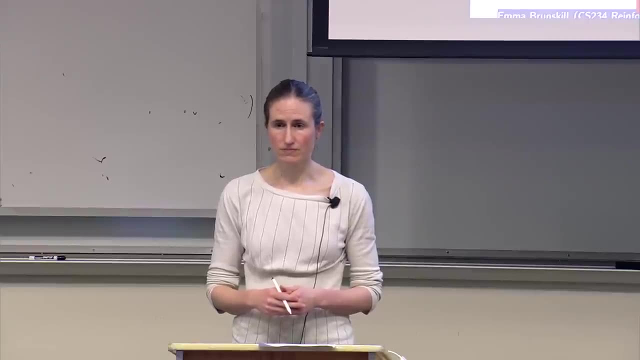 Yeah, So just so I make sure I understand. So when we talk about sampling in tuple, what's really happening is you're going through a trajectory and you're iterating through the- I say, uh, the SARS tuples in that trajectory, in order. 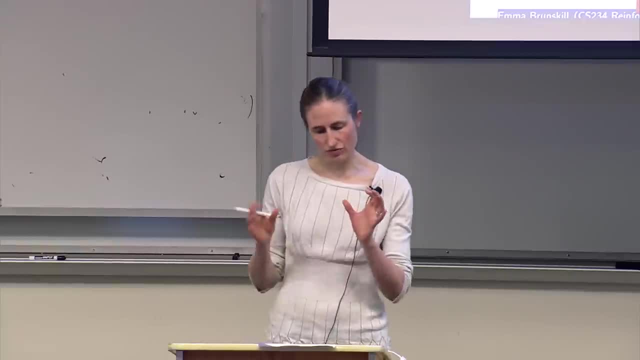 Right, But we're thinking of this really as acting as so, um to repeat the question, The question is like we're going through this trajectory and we're updating in terms of tuples, Yes, but we're really thinking about this as like. 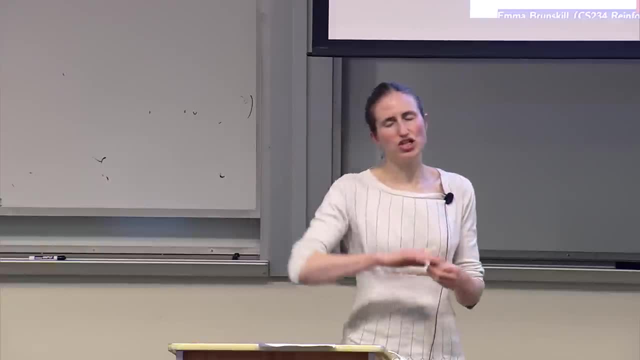 your agent being in some state taking an action, getting a warning into a next state. So there doesn't exist a full trajectory. It's just like I'm driving my car. what's gonna happen to me in the next like two minutes. 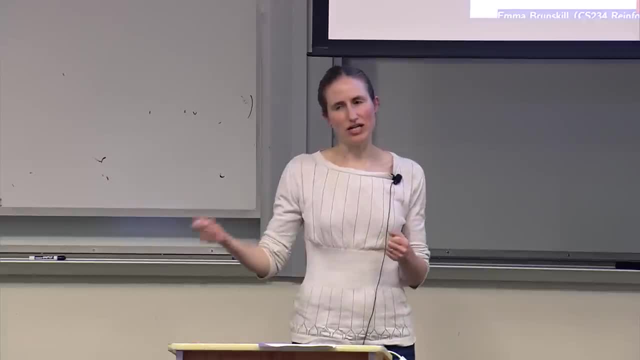 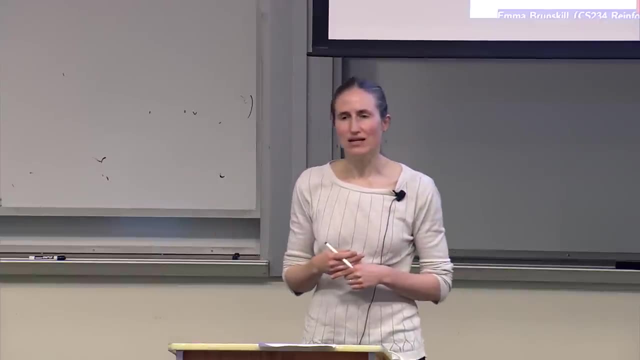 So I don't have the full trajectory and that I'm iterating through it. It's like this is: after every single time step inside of that trajectory, I update. So I don't have to wait till I have the full trajectory, Right And I guess, just to follow up. 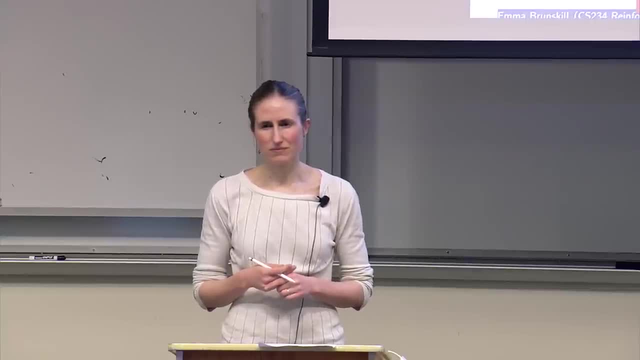 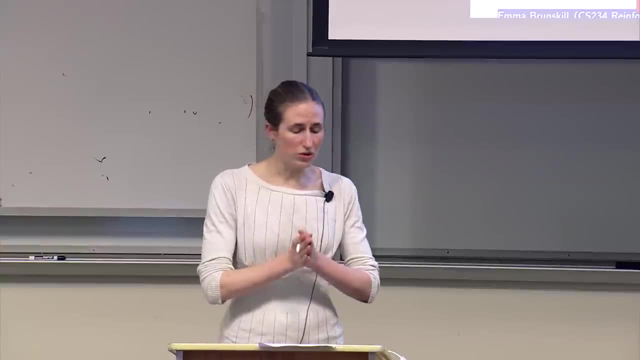 does the order in which those tuples are chosen? I- I'm guessing it matters for the values that you're getting in the estimates? Yes, So the question is: like you know, the order in which you receive tuples. that absolutely affects you know. 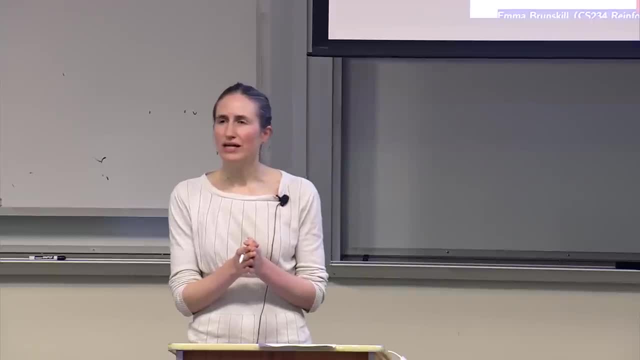 the order in which you receive tuples. that absolutely affects you. know the order in which you receive tuples. that absolutely affects you. know your value. Um so in uh, if- if you're getting this in terms of how you're experiencing in the world. 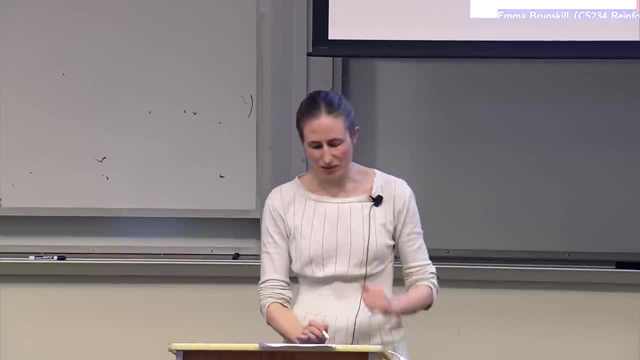 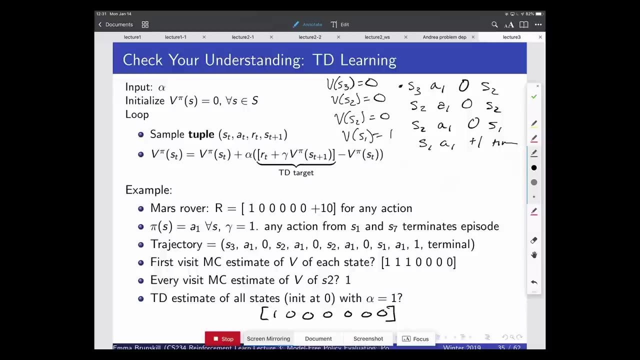 it's just the order you experience these in the world. So this S? t plus pri-, t plus 1 prime becomes your S? t on the next time step. So these aren't being sampled from a trajectory, It's like that's just wherever you are now. 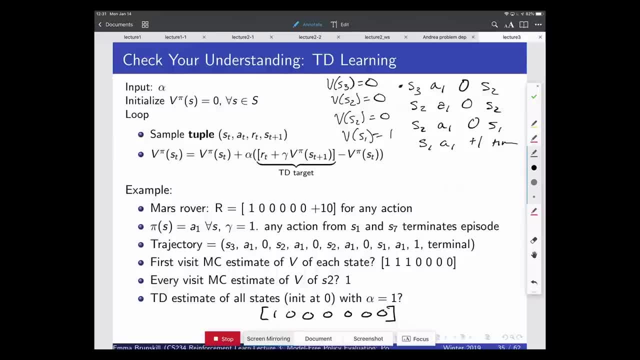 Um, if you have access to batch data, then you can choose which ones to pick, and it absolutely affects your convergence. The problem is you don't often know which ones to pick in advance Questions. Um, the other thing that I just want to mention there. so it's a little bit subtle. 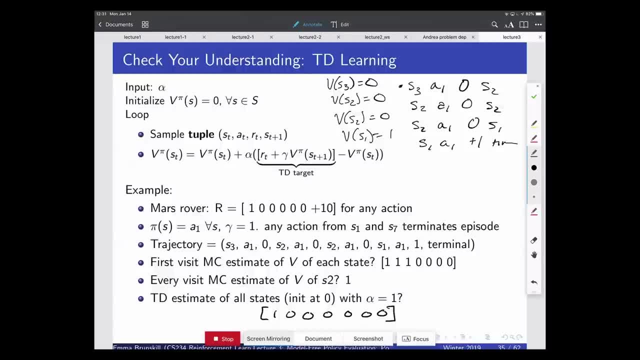 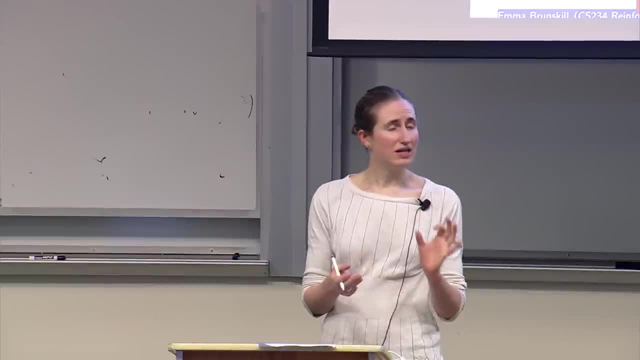 Um, the-. if you set alpha equal to, like you know, 1 over t or things like that, you can be guaranteed to um for these things to converge. Uh, sometimes if alpha is really small, um, also, these are gonna be guaranteed to converge under minor conditions. 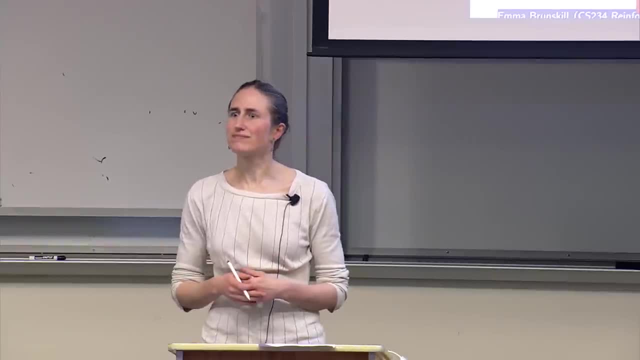 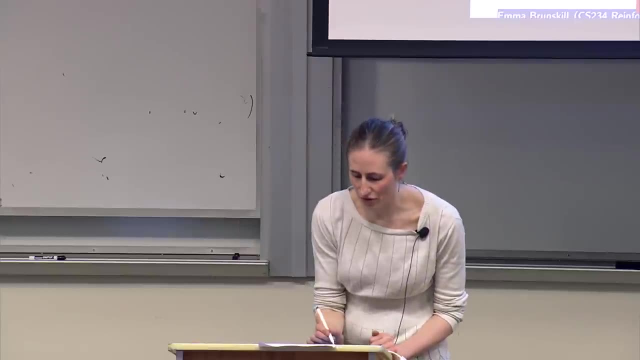 Um, but if you set something like alpha equals 1, it can definitely oscillate. Alpha equals 1 means that essentially, you're ignoring your previous estimate, right? So if you set alpha equal to 1, then you're just using your td target. 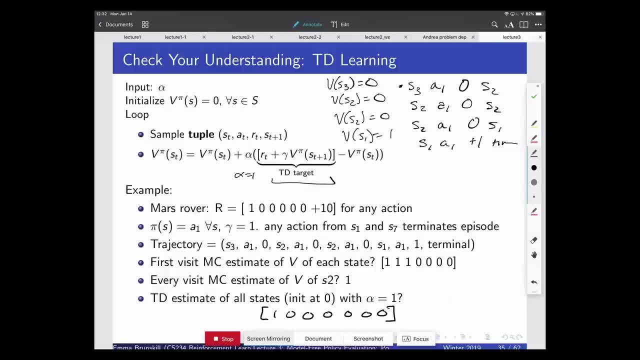 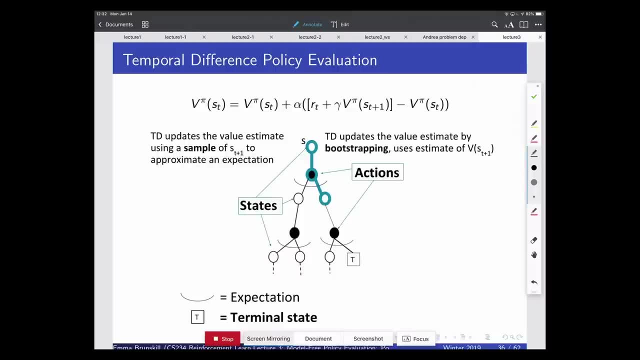 All right, Okay, So what is temporal policy- difference policy evaluation doing If we think about it in terms of this diagram and thinking about us as taking an expectation over futures? So it's um, this is the equation for it up there. 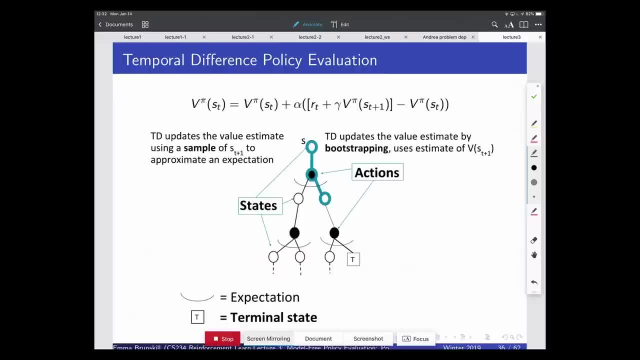 And what it does is it updates its value estimate by using a sample of st plus 1 to approximate that expected next state distribution or next future distribution, And then it bootstraps because it plugs in your previous estimate of v pi for this This one. So that's why it's a hybrid between dynamic programming. 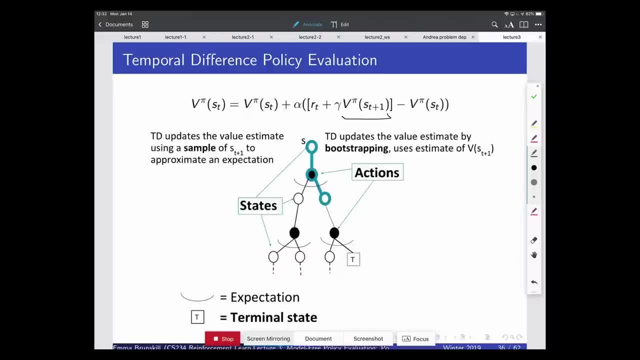 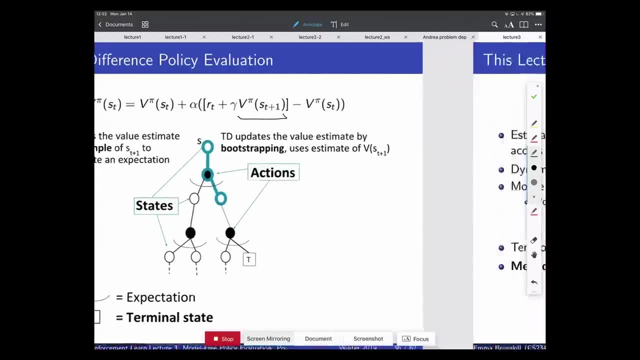 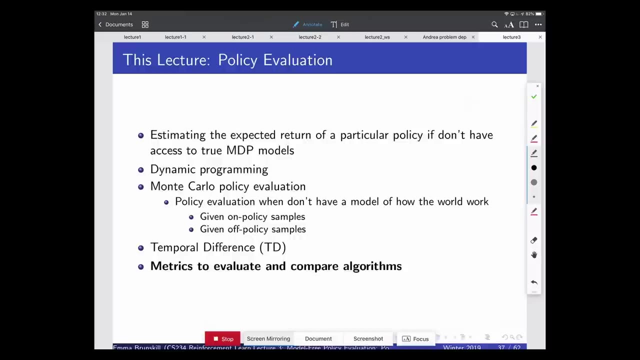 because it bootstraps, and Monte Carlo because it doesn't do an explicit expectation over all the next states. it just samples one. Okay, So now? why don't we think about some of these things that, like, allow us to compare between these different algorithms and their strengths and weaknesses? 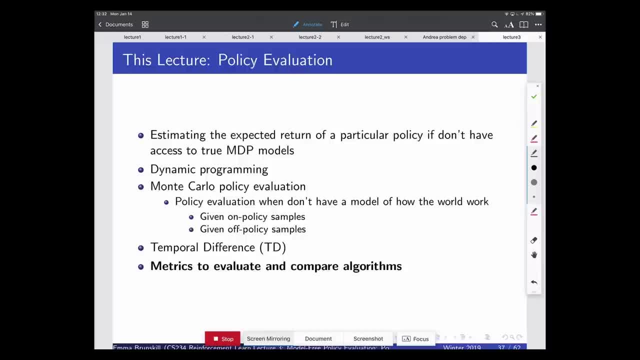 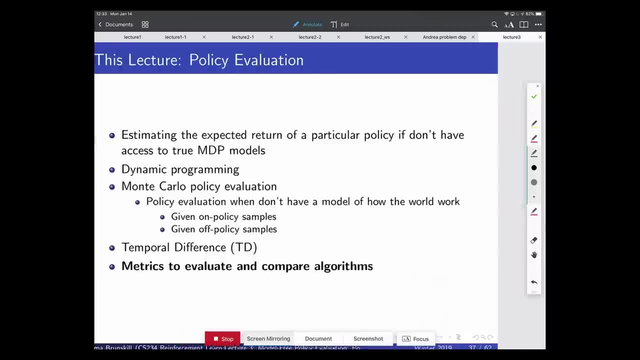 And it sometimes depends on the application. Um, uh, I've had to pick which one is most popular. probably td-learning is most popular, but it depends on the domain. It depends on um, whether you're constrained by data or 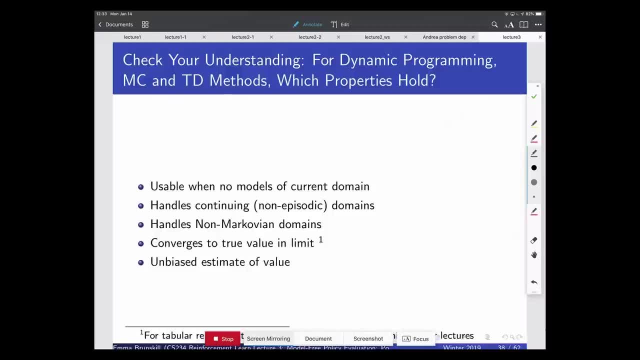 um, you know computation or memory, et cetera, All right. So, um, why don't we spend a few minutes on this briefly? So try to spend a minute and think about which of these properties, from what you remember so far, apply to these three algorithms. 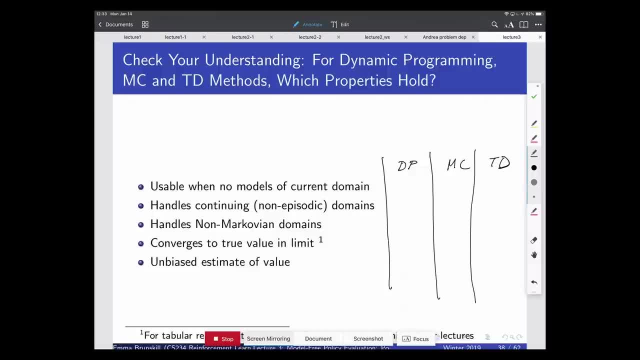 So whether they're usable when you have no models of the current domain. um, whether they handle continuing non-episodic domains. they can handle non-Markovian domains if they converge to the true value and the limit. We're assuming everything's tabular right now. 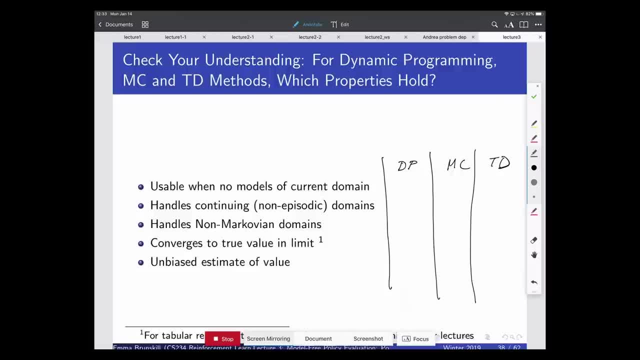 We're not in function approximation land, Um, and whether or not you think they give you an unbiased estimate of the value. So if, at any time point, if you were to take your estimator, if it's unbiased, So why don't we just spend a minute? 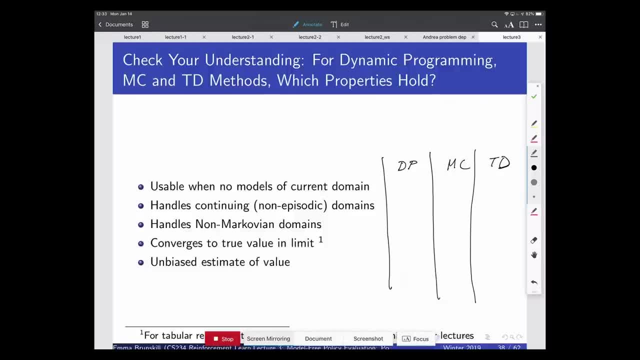 see if you can fill in this table. feel free to talk to someone next to you and then we'll step through it. All right, Which of these are usable when you have no models of the current domain? Does dynamic programming need a model of the current domain? 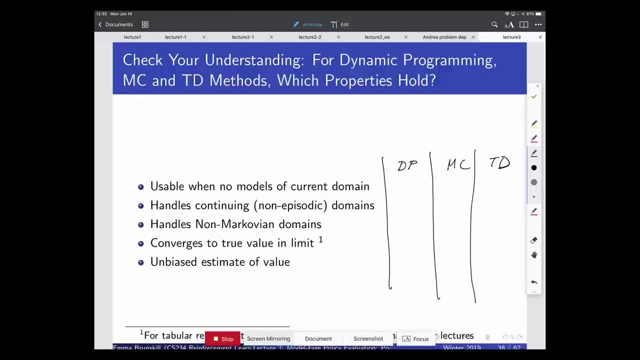 Yes, Yes, Okay. What about Monte Carlo? Usable, Usable. What about TD? Usable? Yeah, Neither of those. TD is known as what- as a model-free algorithm doesn't need an explicit notion. It relies on sampling of the next state from the real world. 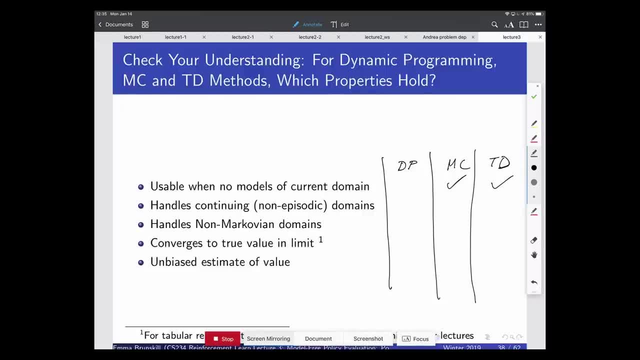 Which of these can be used for continuing non-episodic domains, So like where your process might not terminate ever. Okay Well, can TD learning be used? Yes, Can Monte Carlo be used? No, No. Can DP be used? 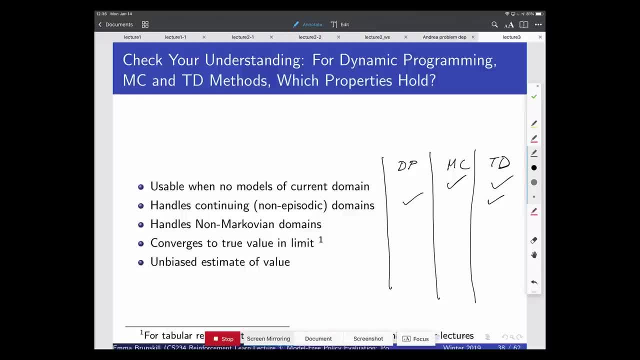 Yes, Yes, Okay, Which of these? um does DP require Markovian? Does Which- does Monte Carlo require Markovian? No, No, Does TD require Markovian? Yeah, it does. So, um ah, temporal-deferential-deferential. um Nah. 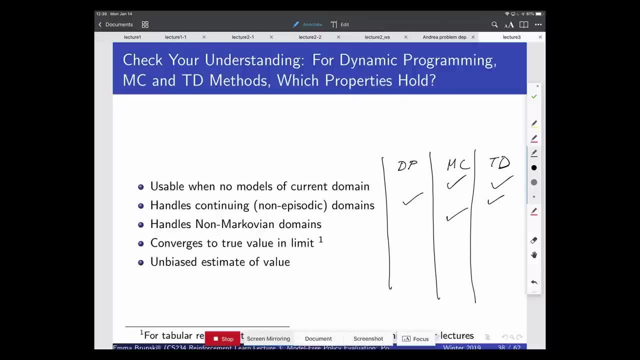 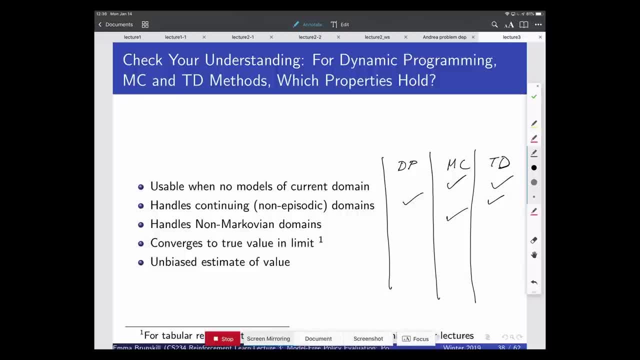 on the history. So, however you got to that current state, it ignores that Um, and then it uses that when it bootstraps too. It assumes that it doesn't. So Monte Carlo just adds up your return from wherever you are now till the end of the episode. And note that, depending on when you got to that, 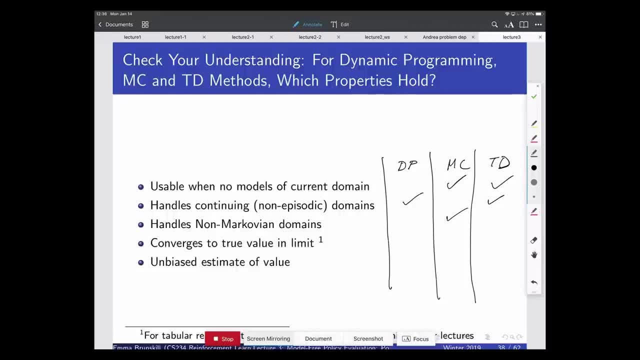 particular state. your return may be different and it might depend on the history. So Monte Carlo doesn't rely on the world being Markov. Um, you can use it in partially observable environments. TD assumes that the world is Markovian. so does dynamic programming in the ways we've defined it. 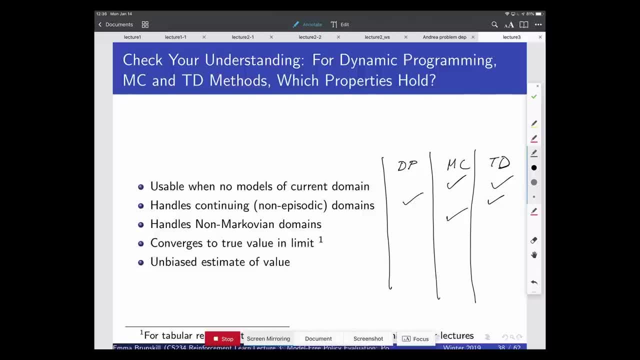 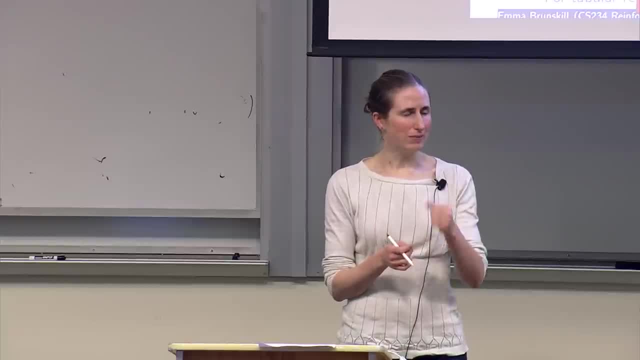 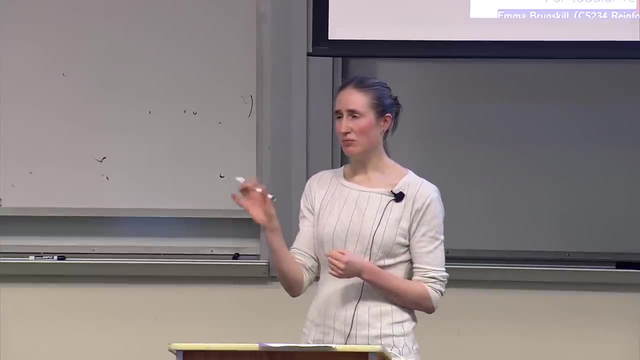 so far. So you bootstrap, you say, um, for this current state, my prediction of the future value only depends on this current state. So I can say I get my immediate reward plus whatever state I transition to. That's a sort of a sufficient statistic of the history and I can plug in my 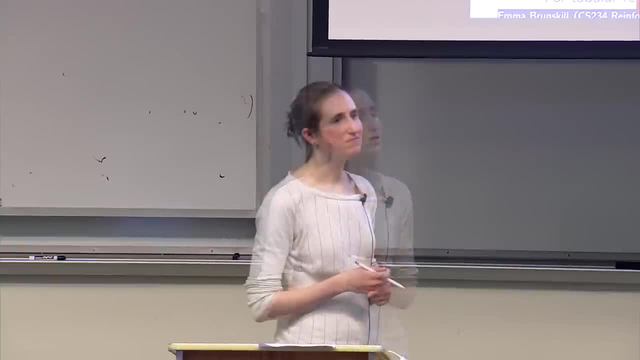 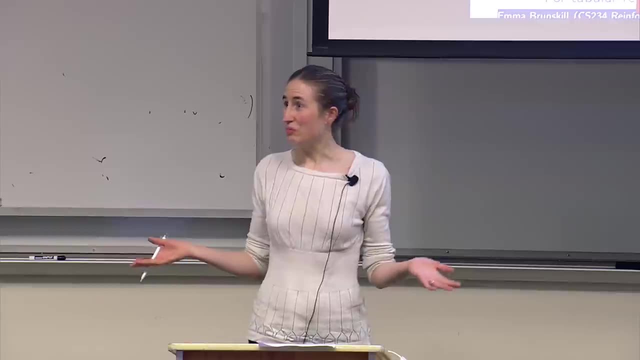 bootstrap estimator, So it relies on the Markovian. essentially What non-Markovian domain? I guess you could apply it? Um yeah, So the question is well, what do you mean by non-Hudley Like? these are algorithms you could. you could apply them. 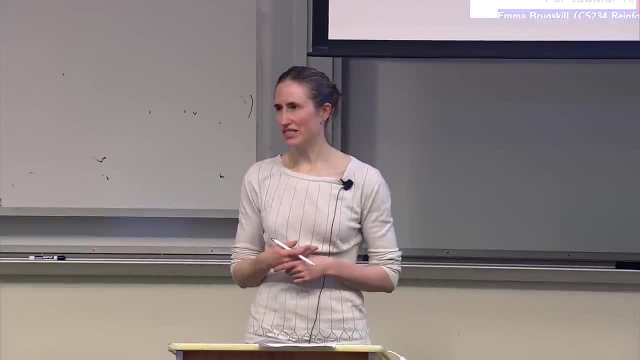 Um. so yeah, you can apply these algorithms to anything. The question is whether or not they're guaranteed to converge in the limit to the right value, And they're not. if the world is not Markovian And they don't Like um. 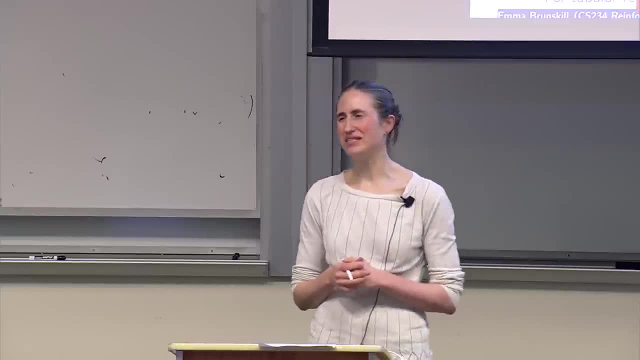 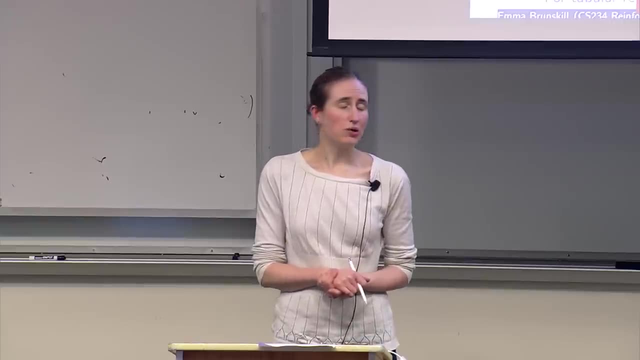 we've seen in some of our work on intelligent tutoring systems. early on we were using some data, um from a fractions tutor and we were applying Markovian techniques and they don't converge. I mean they converge to something. it's just totally wrong. and it doesn't matter how much data you have. 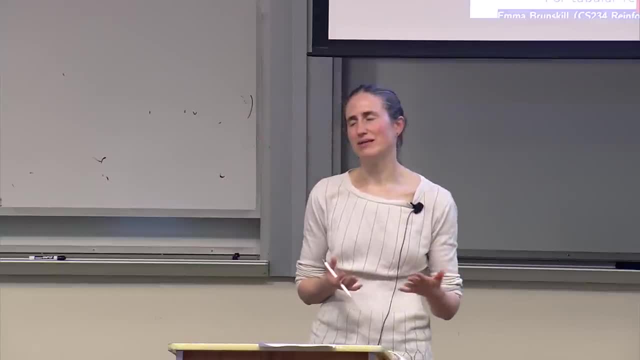 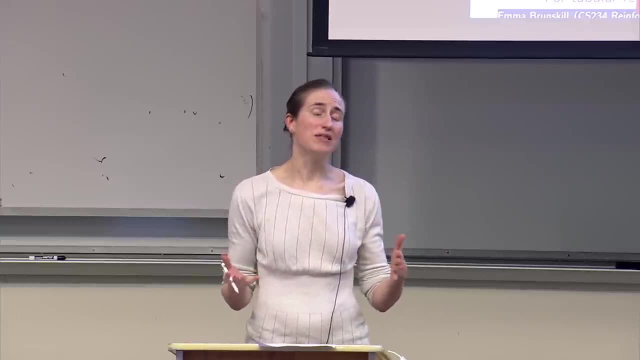 because you're- you're using methods that rely on an assumption that is incorrect. So you'd need to be able to evaluate whether or not Markovian or- or try to bound the bias or do something, Um, otherwise, your estimators of what the value is of 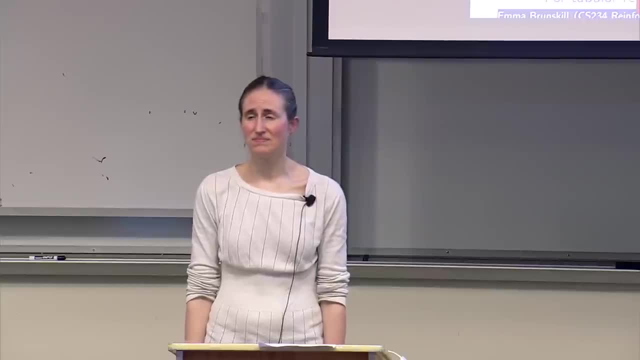 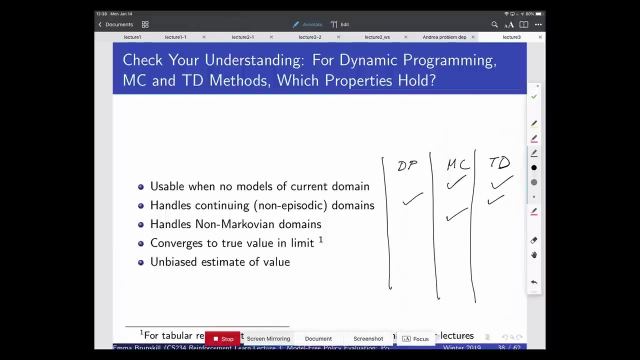 policy can just be wrong, even in the limit of infinite data. Um, what about converging to the true value in the limit? Let's assume we're in the Markovian case again. So for- for Markovian domains, does um Dp converge to the true value in the limit? 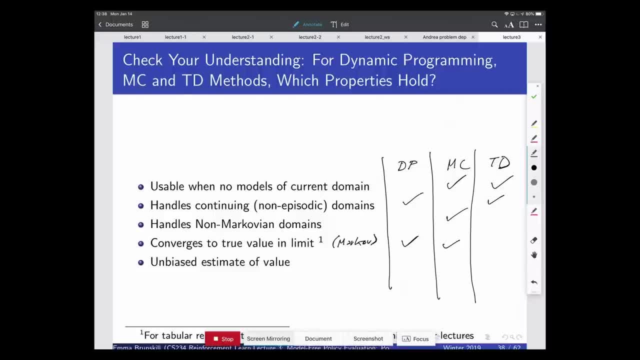 What about Monte Carlo? Yes. What about Td? Yes, All of them do. If the world is really Markovian, um, everything converges asymptotically. Now, under minor assumptions, all of these require minor assumptions, Um I- so under minor assumptions. 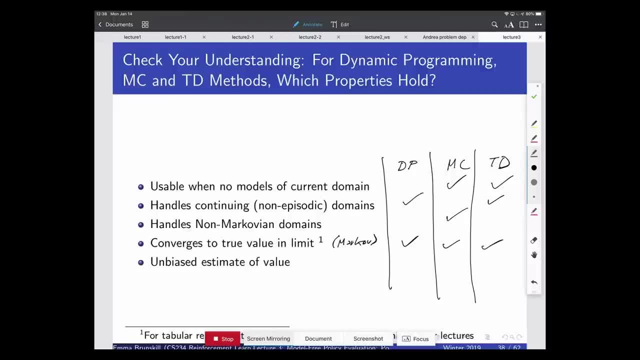 it'll converge to the true value of the limit depending on, like, the alpha value. Um, uh, what about being an unbiased estimate of the value? is Monte Carlo An unbiased estimator? Yes, Okay, Td is not. Dp is a little bit weird. 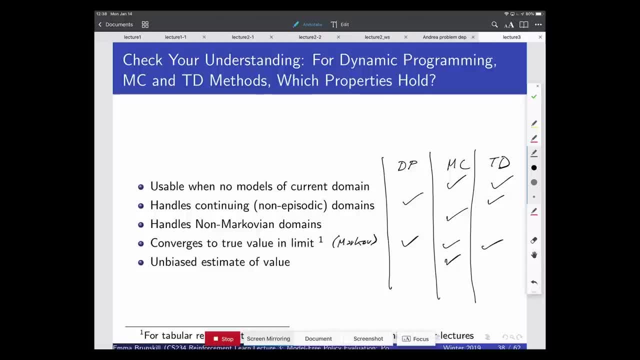 It's sort of a- not a quite fair question there. Dp is always giving you the exact v k minus 1 value for that policy. So that is perfect. That is the- the exact value if you have k more 1-, k minus 1. more time steps to act. 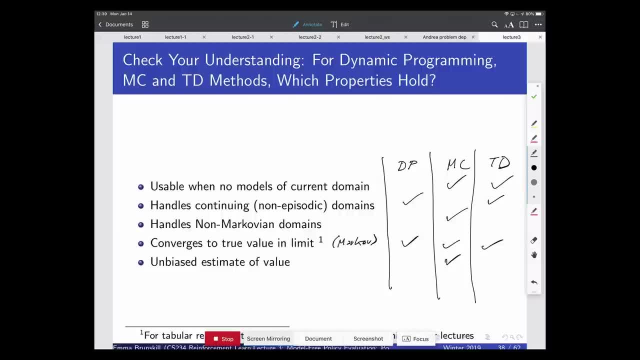 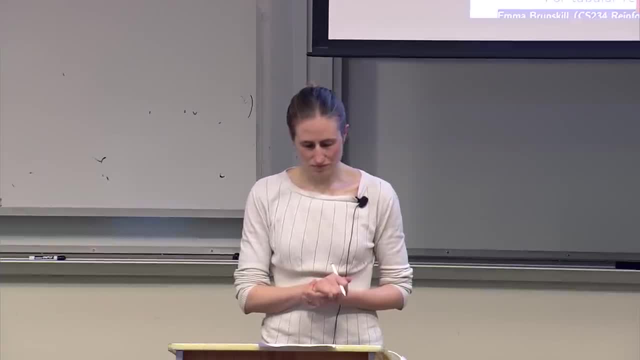 That is not gonna be the same as the infinite horizon value function. Yeah, Can you explain how- the last two lines are different. Like I don't understand the difference between an unbiased estimator of value and something that converges to the true value of the limit. 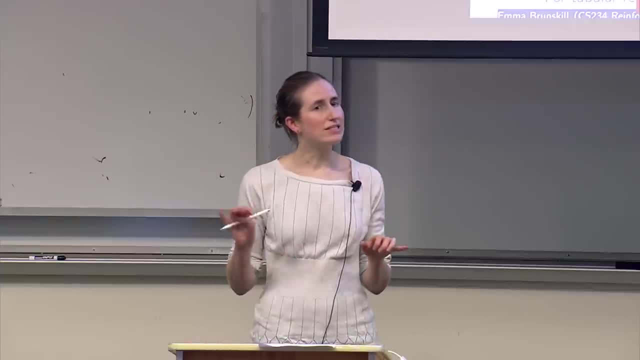 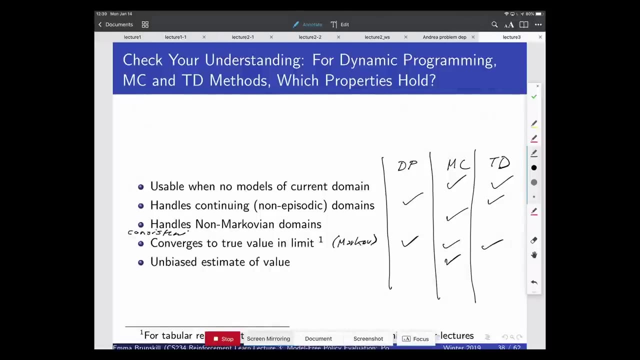 Question is great. So the question is: what's the difference between something being unbiased and consistent? Um, so, when we say converges to the true value of minute, that's also known as formally being a consistent estimator. So the unbiased estimate of the value means. 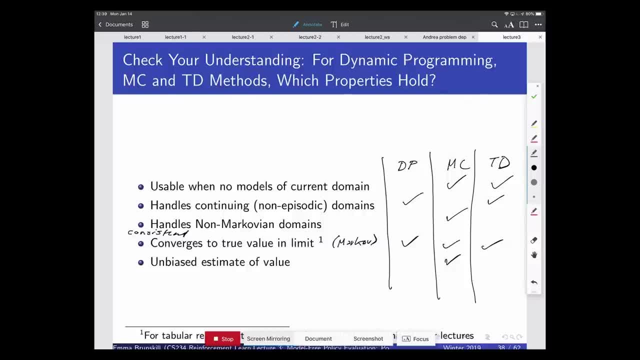 if you have a finite amount of data and you compute your statistic, in this case the value, and you compare it to the true value, that on average that difference will be zero. And that is not true for things like TD, But, um, and that can be- that's being evaluated for finite amounts of data. 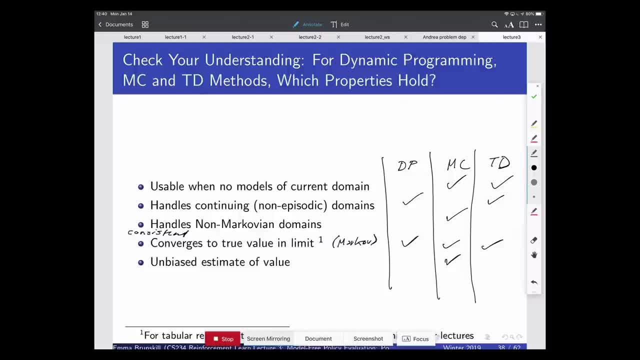 What consistency says: if you have an infinite amount of data, will you get to the true value? So what that implies is that say for TD that asymptotically the bias has to go to zero, And if you have infinite amounts of data, 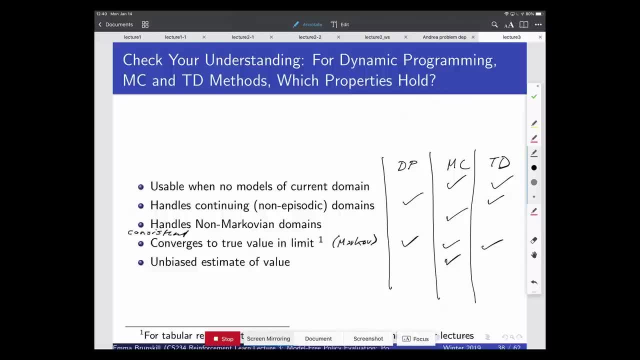 eventually its bias will be zero, But for a small amount. you know, for finite amounts of data and really you know, you don't know what that n is Um. it could be a bias estimator, but it's the amount of data you have. that goes to infinity. 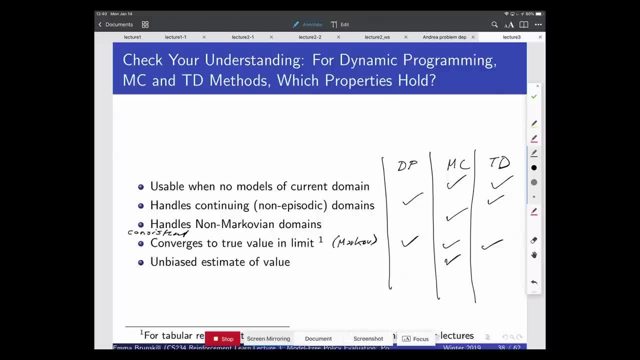 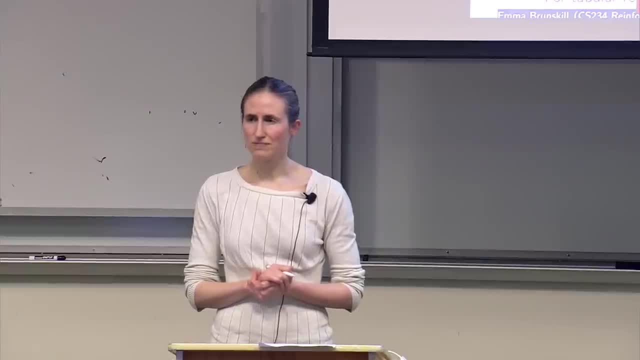 then it has to converge to the true value So you can have things that are biased, estimators that are consistent. Yeah, For Monte Carlo. I thought we said that the implementation has an effect on whether or not it's biased, Because I thought we said that if it's every visit, then it-. 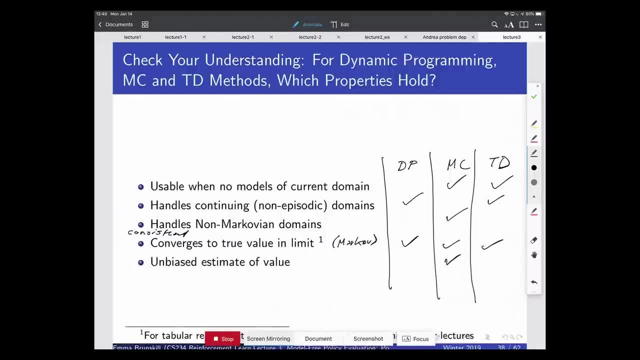 Good question. yes, So I. um question is good. So this is um. it's an unbiased estimate for the um first visit and for every visit it's biased. Okay Question. Um, so this might be a redundant or, uh, dumb question. 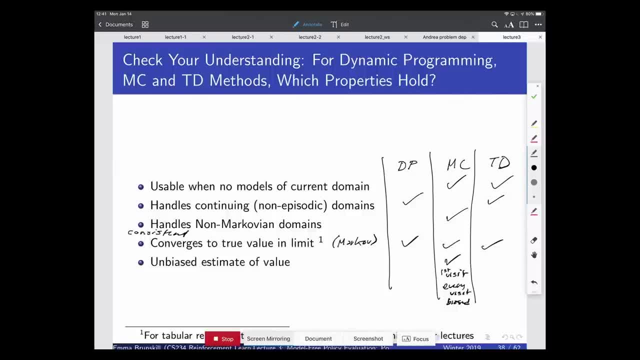 but are there any- uh, you know, model-free policy evaluation models that aren't actually convergent? Yes, The question was: are there any model-free policy evaluation methods that are not convergent? Yes, and we will see them a lot when we get into function approximation. 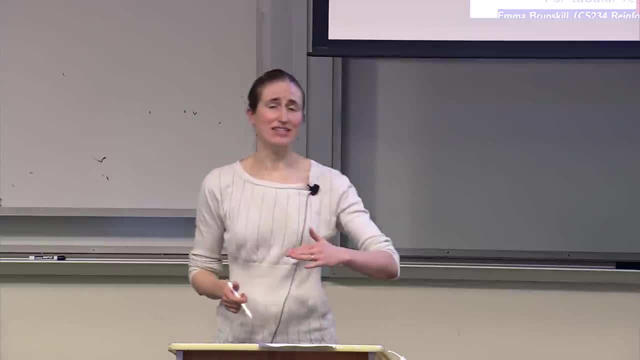 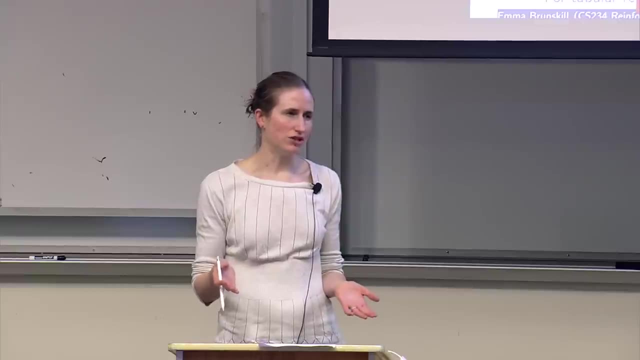 When you start-. so right now we're in the tabular case, which means we can write down as a table or as a vector what our value is When we move up to infinite state spaces. um, a lot of the methods are not even guaranteed to converge to anything. 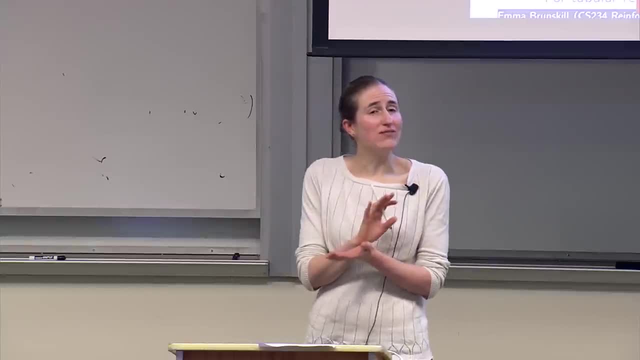 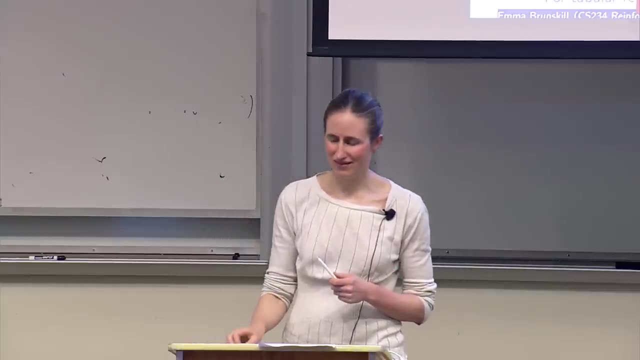 Not even- we're not even talking about whether they converge to the right value. They're not even guaranteed to stop oscillating. Okay, They can just keep changing. Okay, Yeah, question. So: how can- is there any intuitive explanation why TD is not unbiased? 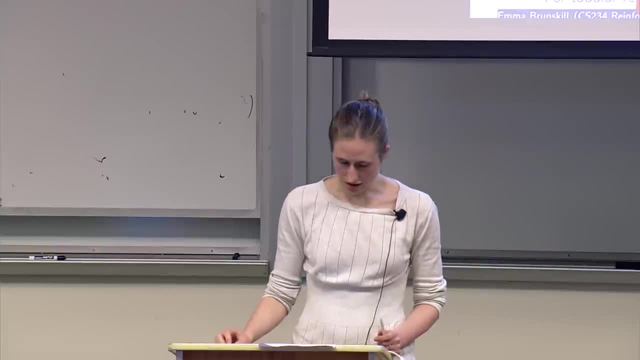 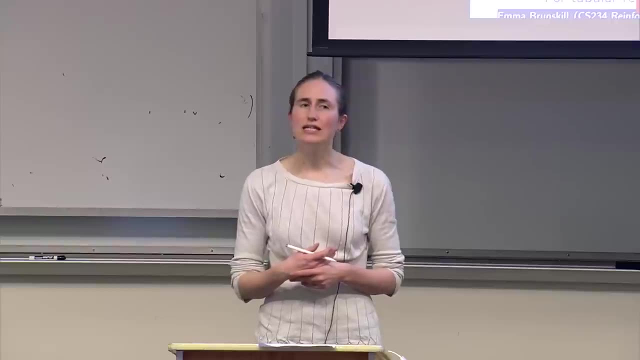 Is- is what? Why TD is not unbiased, Why it's not biased? Ah yeah, great question. So the question was to say: you know, why is TD biased? TD is biased because you're plugging in this estimator of the value of the next state. that is wrong. 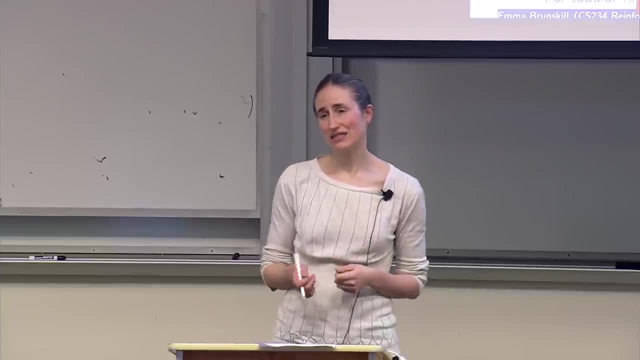 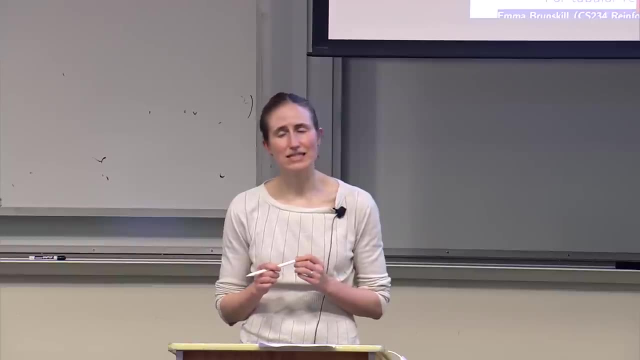 And that's generally gonna lead to- lead to- some bias. You're plugging in an estimator that is not the true b-pi for S prime. It's gonna be a little bit of bias. So it's really that- that- that bootstrapping part. that's the problem. 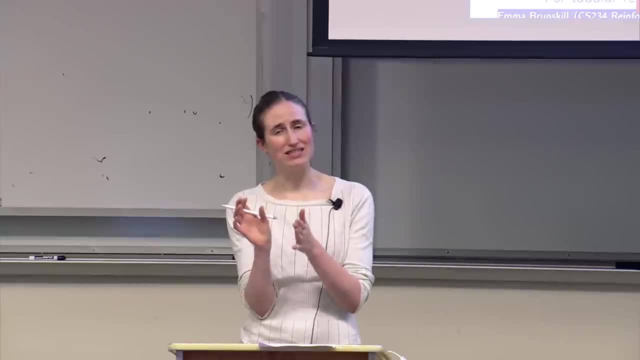 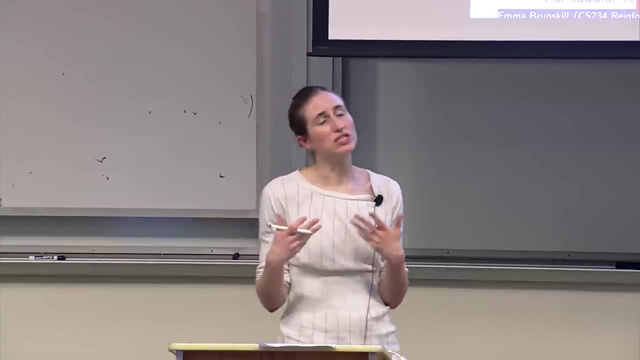 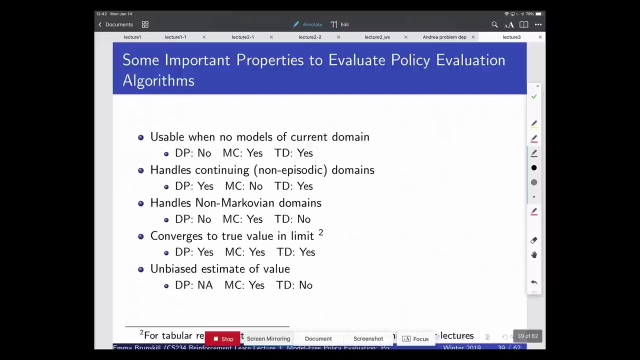 The Monte Carlo was also sampling the expectation and it's unbiased, at least in the first visit. case Problem here is that, um, you're plugging in an expected discounted sum of rewards. that is wrong. All right, So, um, that just summarises those there. 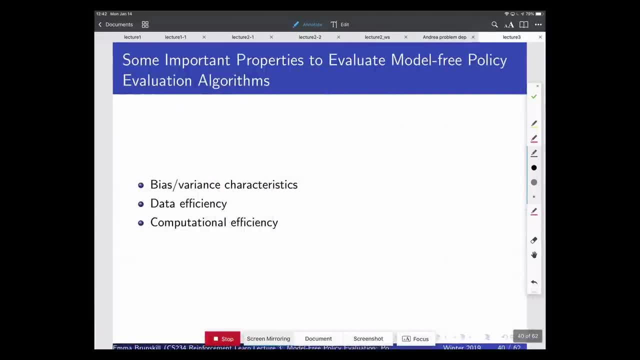 I think there are important properties to think to compare between them. Um, how would you pick between these sort of algorithms? So I think thinking about bias, invariance, uh, characteristics, is important, um, data efficiency efficiency is also important, as well as computational efficiency. 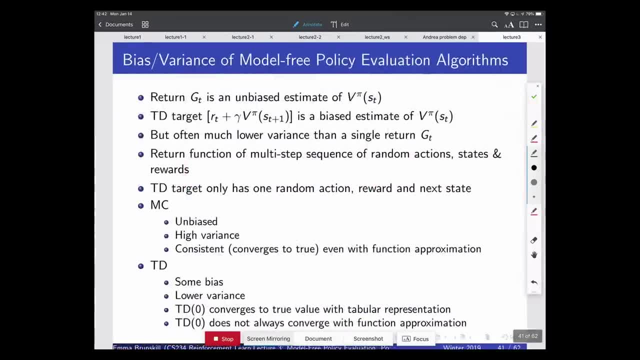 And there's gonna be trade-offs between these Um. so if we think about sort of the general bias variance of these different forms of algorithms, um, Monte Carlo is unbiased, generally high variance um and it's consistent. TD has some bias, much lower variance than Monte Carlo. 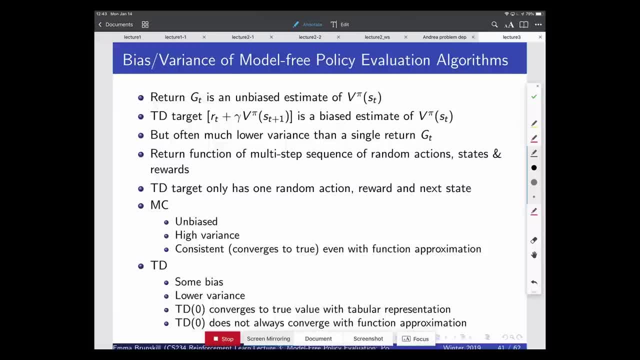 Um TD0 converges to the true value with tabular representations And, as I was saying, it does not always converge once we get into function approximation And- and we'll see more about that shortly, I think with the last few minutes. 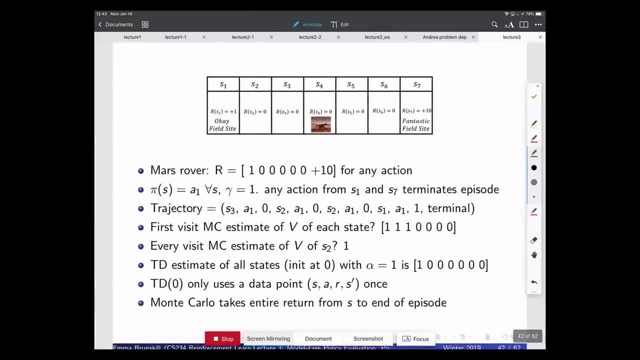 I think we'll have a chance to get through um a little bit about how these methods are related to each other when we start to think about the batch setting So, as we saw in this particular case for the Mars Rover, just to again contrast them um. 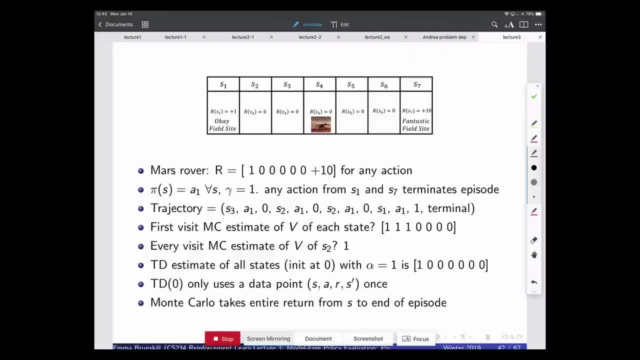 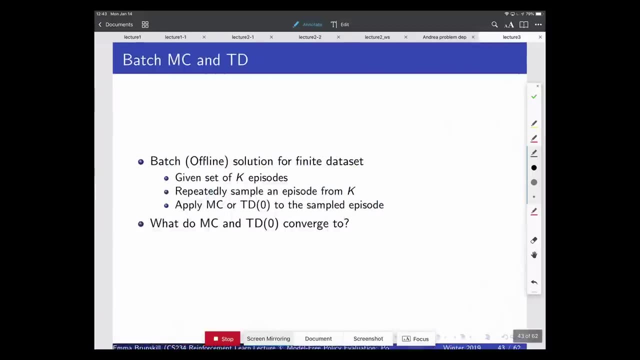 Monte Carlo estimate waited till the end of the episode and then updated every state that was visited in that episode. TD only used each data point once, and so it only ended up changing the value of the final state In this case. so what happens if we want to go over our data more than once? 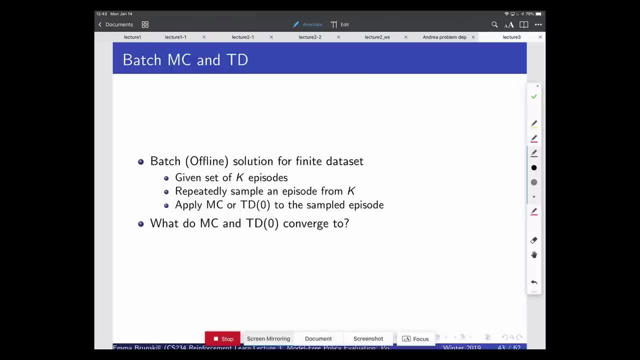 So let's say we're willing to spend a little bit more computation so we can actually get better estimates and be more sample efficient, meaning that we want to use our data more efficiently so that we can get a better estimate. So often we call this batch. 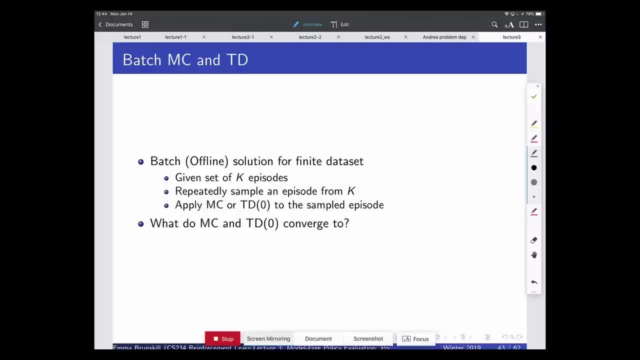 or offline um policy evaluation, where we've got some data and we're willing to go through it as much as we can in order to try to get an estimate of the policy that was used to gather that data. So let's imagine that we have a set of 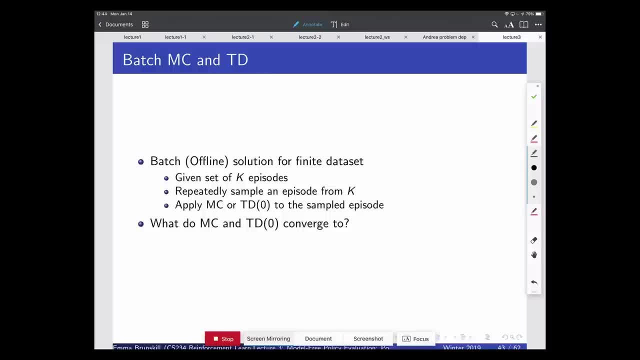 K episodes, and we can repeatedly sample an episode, Um, and then we either apply Monte Carlo or TD to the whole episode. What happens in this case? Um, so there's this, uh, nice example from Sutton and Barto. Um, let's say, there's just two states. 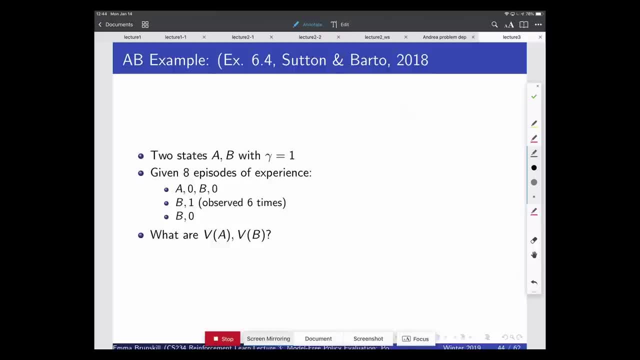 So there's states A and B and Gamma is equal to 1, and you have eight episodes of experience. So you either- the first episode you saw A 0,, B- 0, so this is the reward In B. you saw- in the- sorry. 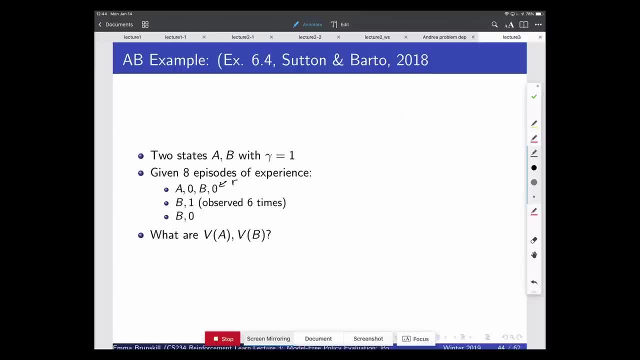 in the- in the- another set of episodes, you just started in B and you got 1, and you observed that six times And then in the eighth episode you started in B and you got a 0.. So first of all, can we compute what V of B is in this case? 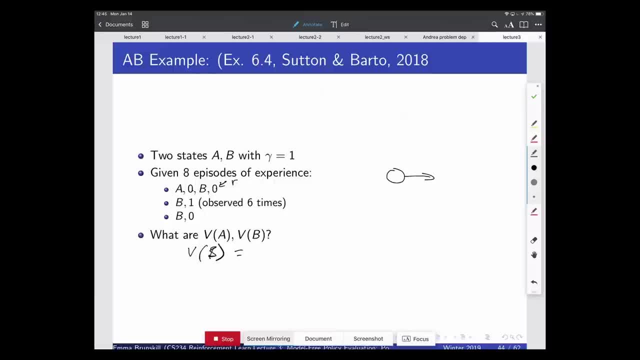 So the- the- the model of the world is gonna look something like this: You got a, B and the B sometimes goes to 1, and B sometimes goes to 0, and then we always terminate. So in all eight episodes we saw B. 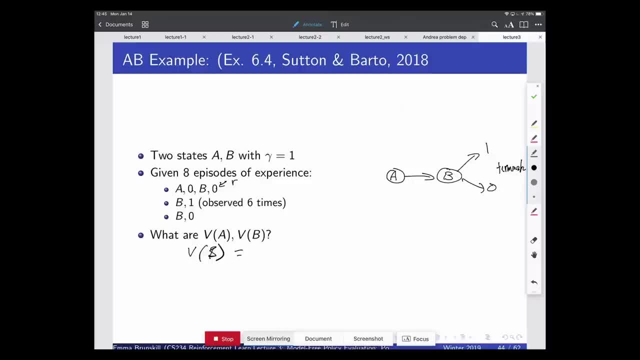 In six of those we got a 1.. In two of them we got a 0.. So if we were doing Monte Carlo, what would be our estimate of B, value of B? So if we do the Monte Carlo estimate, 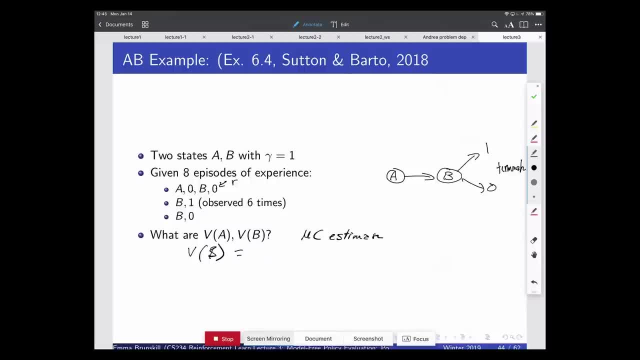 using these eight episodes And we can go over them as many times as we want. We don't just have to experience each episode once. This is the batch dataset. Someone already collected this for us. You can do Monte Carlo updates of this dataset as much as you want. 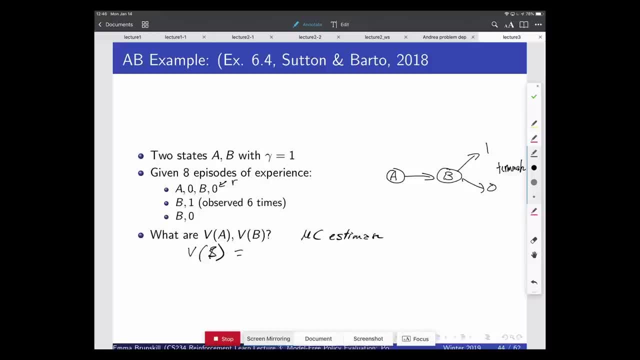 What will be the estimate of V of B, in this case, Three quarters, Which is just equal to six divided by eight In the Monte Carlo estimate. or do TD what will be the TD estimate of B? Remember what TD does is they get this S A R S prime and you bootstrap. 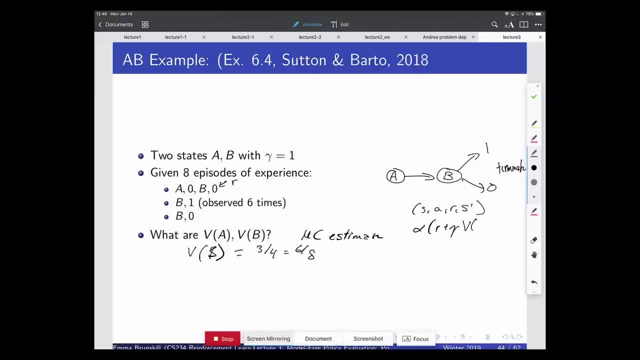 You do alpha times R plus gamma V of S prime, And then you do one minus alpha of your previous estimate Um. here, in this case, you can make alpha anything small. You're going to do it an infinite number of times. 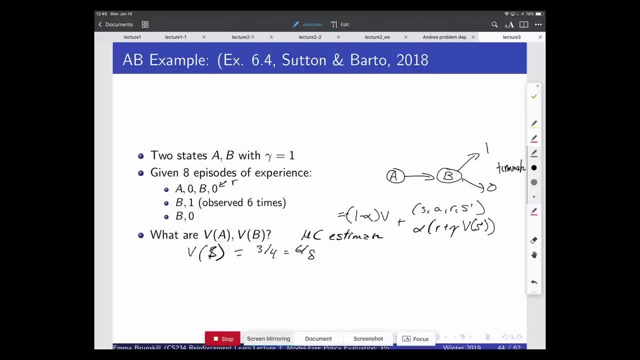 So this is the batch data setting. So for TD, you're just going to run over your data like millions and millions of times until convergence. basically, Does somebody have any guesses of what V of B would be for TD? It's also three quarters, okay. 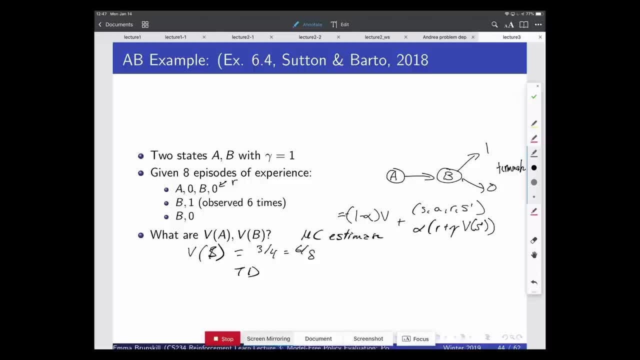 So for- for TD it's the same, because whenever you're in B you always terminate, So it's really like just a one-step problem from B And so for TD it'll also say: V of B is equal to six divided by eight. 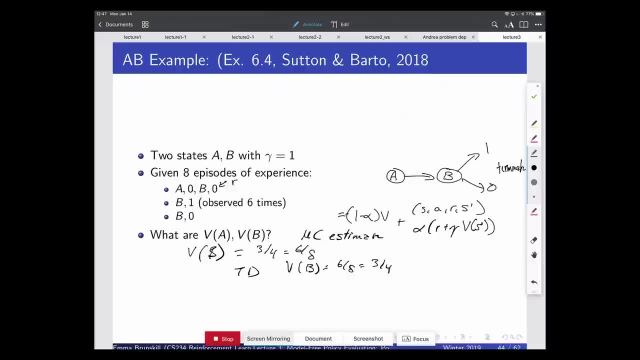 which is equal to three quarters. So the two methods agree in the batch setting for this. If you can go over your data in infinite amount of time, um V of B is equal to three-, uh, six-eighths, and so is um. 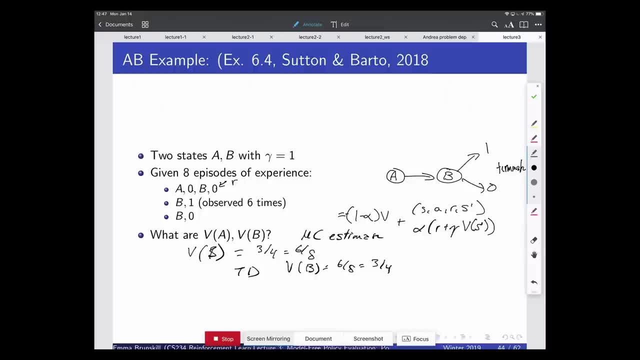 uh, under both methods. Um, does anybody know what V of A would be under Monte Carlo? Okay, Yeah, V of A under Monte Carlo is going to be zero. Why, Yeah, go ahead. Uh, because the only- only uh. 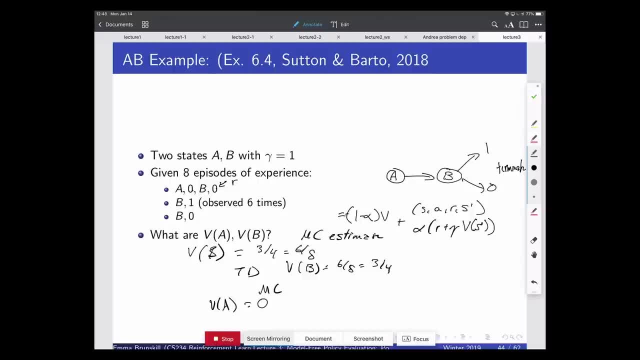 trajectory is where you have A and not with zero- That's right. There's only one trajectory where you have an A and it got a zero award. What do you think might happen with TD? Is it just-? is it going to be zero or non-zero? 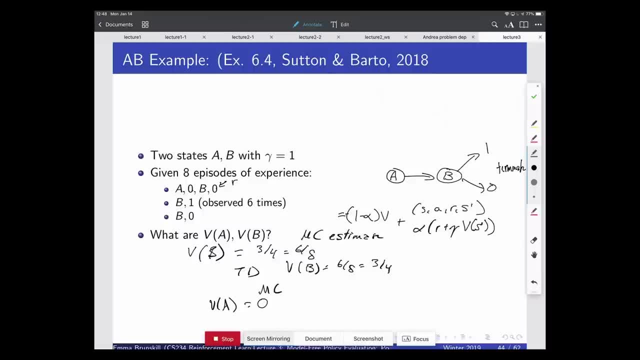 It's non-zero. It's non-zero Why? Because you could strap the-. Because you could strap right So- so yes, the only time you're in A, you happen to get zero in that trajectory. But this is- in TD, you would say. 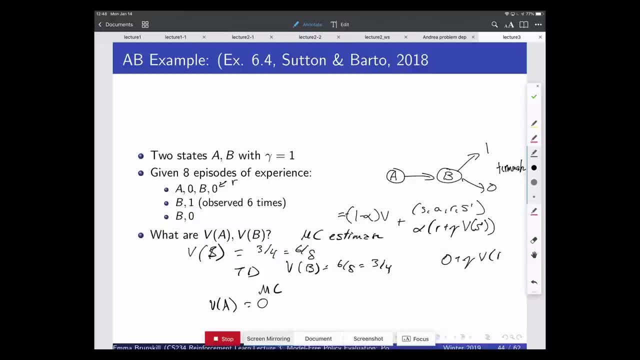 well, you got an immediate zero plus gamma times V of B, And V of B is three-quarters. So here gamma is equal to one. So your estimate of this under TD would be three-quarters. So they don't converge to the same thing. 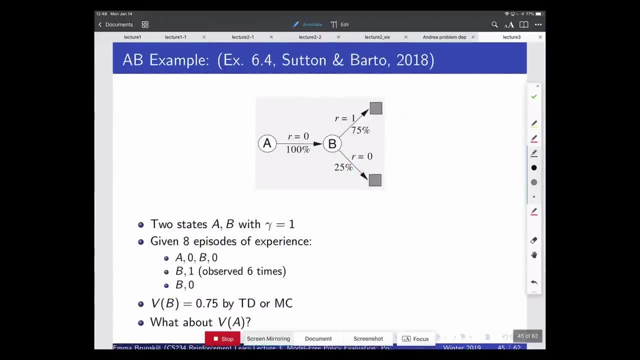 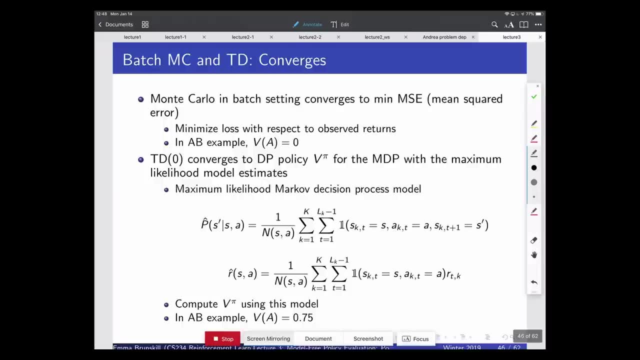 Okay, So why does this? um, uh, so this is what we just went through and we can think about it in terms of these probabilities. Um, so what does- what's happening here? Monte Carlo, in the batch settings, converges to the minimum mean squared error estimate. 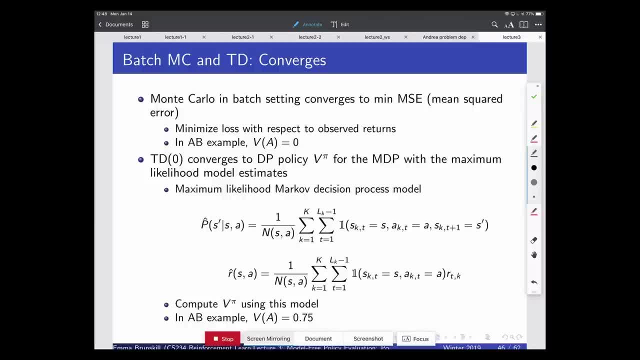 So it minimizes loss with respect to the observed returns. Um, and in this example V of A is equal to zero. TD zero converges to the dynamic programming policy with the maximum likelihood estimates for the dynamics and the reward model. So it's equivalent to: if you essentially just through counting 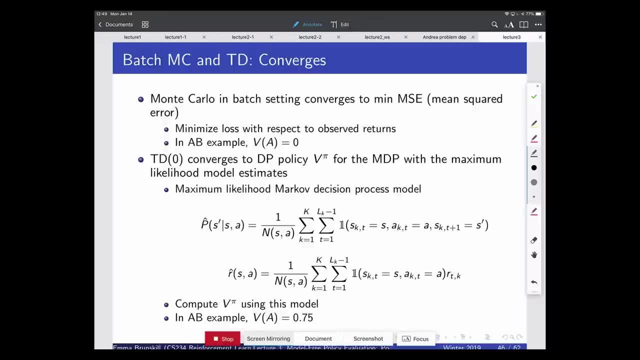 you estimated P hat of S prime given S A, So for-. this would say the probability of going B given to A is equal to one In this case, because the only time you've been in A you've went to B. 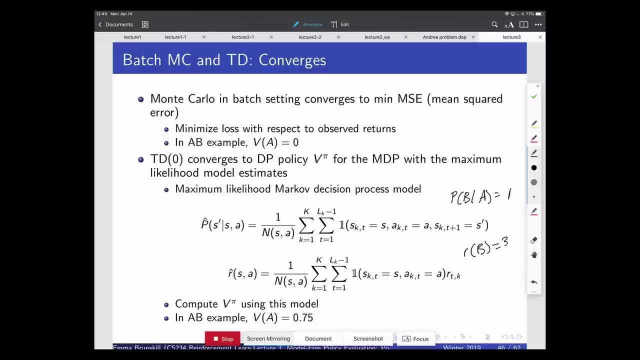 And then the reward for B is equal to three-quarters and the reward for A is equal to zero. And then you would do dynamic programming with that and you would get out the- get out the value. So TD is converging to this sort of maximum likelihood. MDP value estimation. 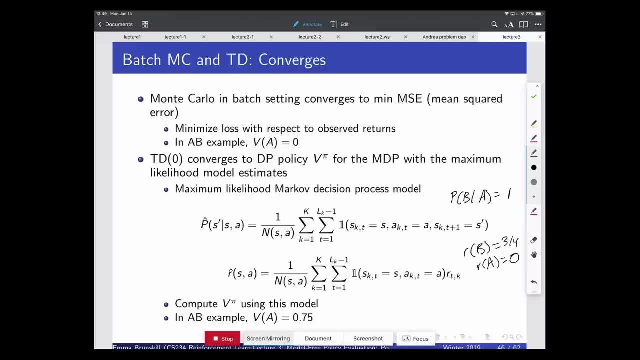 And Monte Carlo is just converging to the mean squared error. It's ignoring-. well, it doesn't assume Markovian-ness, so it's not using the- this Markov structure Question. Sorry, just to confirm on the previous slide. 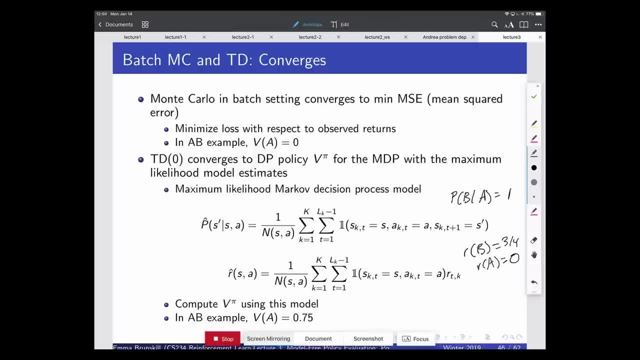 um, you're talking about going over the data many times. Because for TD learning on the first iteration, V of A would be zero, right, Because V of B hasn't been set yet. You're just assuming that after a while. 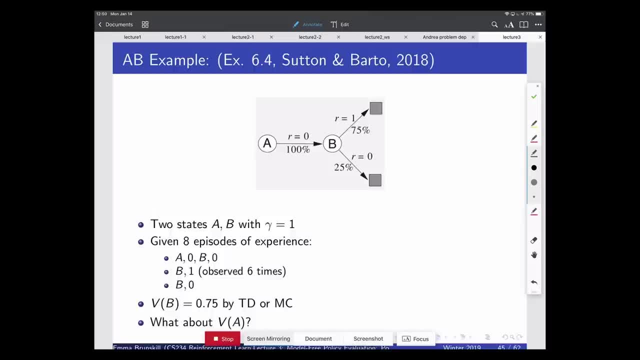 V of B has converged to three-quarters. Exactly, Exactly, right. So in- in um in the online setting um, if you just saw this once, uh, then this- then V of A would be zero For that particular update. 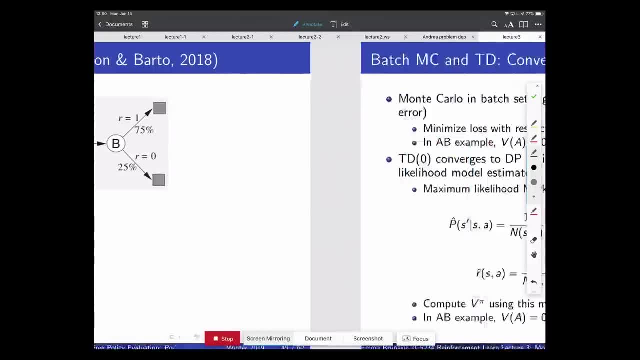 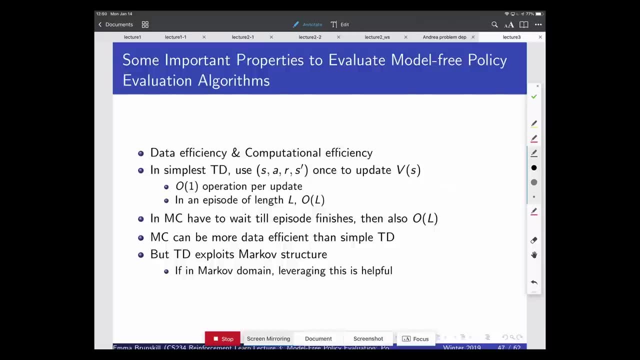 It's just that if you did it many, many, many times, then it would converge to this other thing. So you know which one is better? Well, if your world is not Markovian, you don't want to converge to something as if it's Markovian.